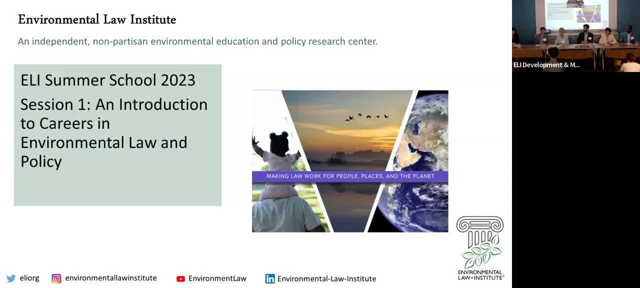 Environmental Law session that you're all at now. We'll also have a Land Use and Energy Law session in person on June 22nd And then at the end of July we'll have our Hazardous Waste Insights session in person. The rest will all be online. So every Thursday, except for June 29th. 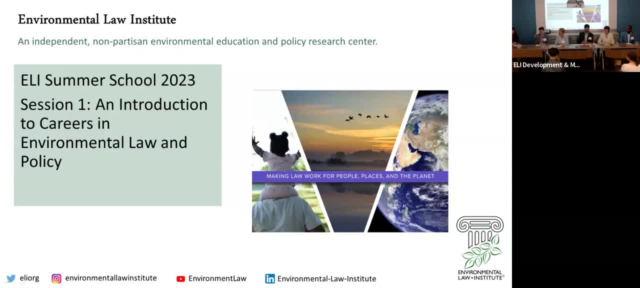 which we're taking a break that day. So please register on ELI's website for the rest of them. If you're interested, we would love to have you. Our other five sessions, the ones that are offered via webinar, will be recorded and posted to the website, as well as our in-person sessions. So 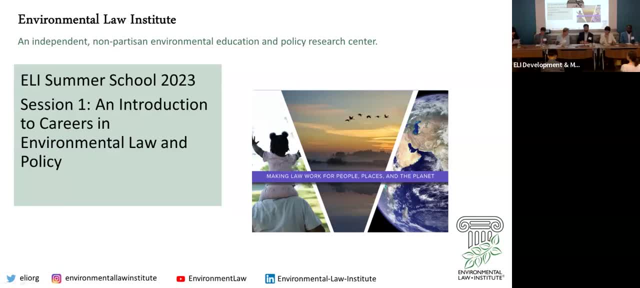 if you can't make it to one, feel free to watch it back later, And all the sessions are free, but please do register so we know that you're coming and seeing us. So thank you so much for joining us today And we hope that you get all of the relevant information for them. 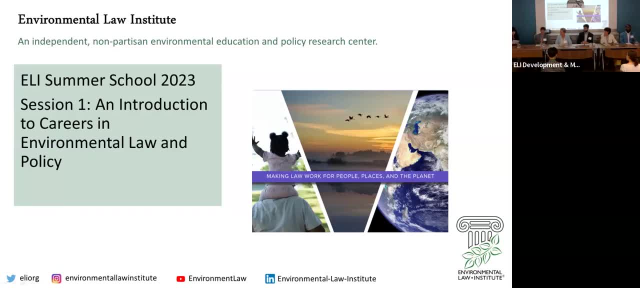 So now we'll go ahead and kick off our first session of Summer School. So today's session is an introduction into careers, And we have a wonderful, wonderful group of leading experts here to tell you about their journeys in environmental law and share advice with all. 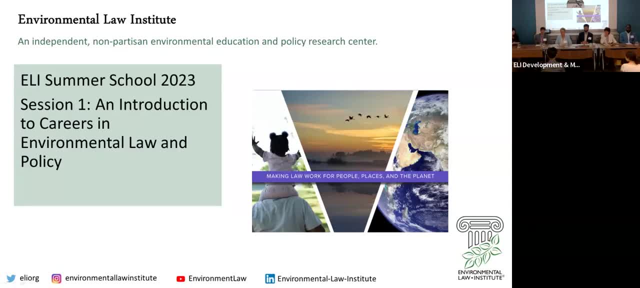 of you. This will be more of a roundtable discussion format, So I'll be leading a discussion, We'll hold time at the end for audience questions, So please think of questions, And then we'll ask you at the end to raise your hands and bring a microphone around. 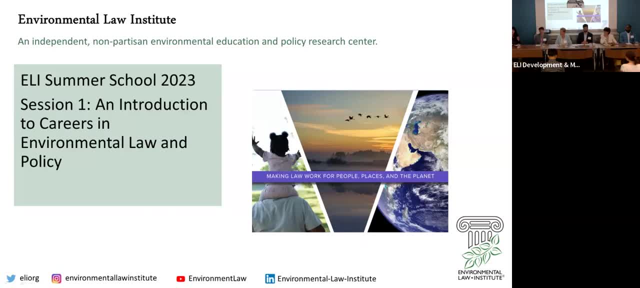 and we will try to end a little bit early so that we have time for networking as well. If you'd like to speak with our wonderful panelists today, So that'll go ahead and get started. I usually read introductions at the start of each session of Summer School, but given today's topic, I'm going 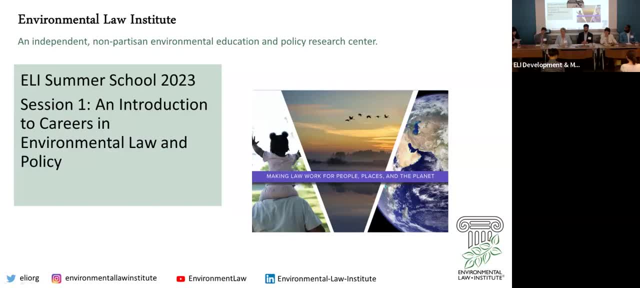 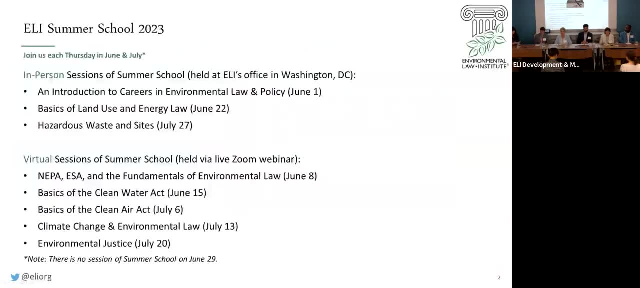 to let our speakers introduce themselves. So our first question is: could you please introduce yourself and tell our audience about your career journey so far? What made you interested in pursuing a career in environmental law? And we'll start with Jared Page, the staff attorney here at. 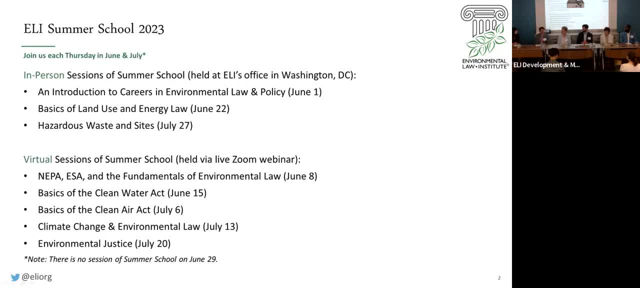 ELI, Hi everybody, So glad to have you here And it's a pleasure to be able to speak with you today. As Madison said, my name is Jared Page. I'm a staff attorney at the Environmental Law Institute. Just briefly, the Environmental Law Institute, Research and Education Institute, looking at 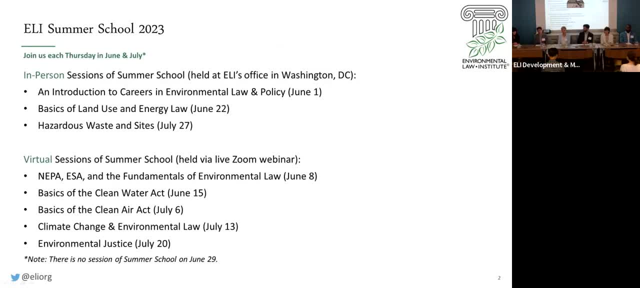 solving tough environmental problems with innovative solutions. So how did I get my start in environmental law? How did I make my way here? It's a somewhat circuitous path. I think there's some people who sort of manage to find out what they want to do when they're five years old and 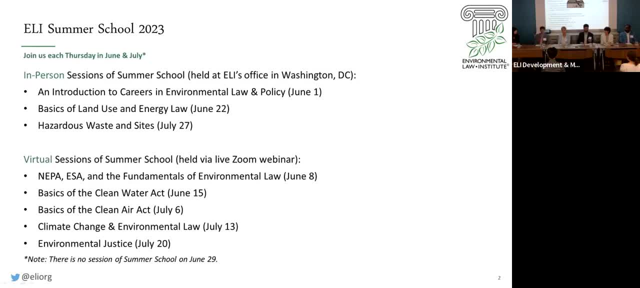 sort of pursue that with steadfast determination all the way through their career. And that was not me. I actually grew up wanting to be a dentist of all things, And my first day of college advising, they laid out what classes I was needing to take to become a dentist, And I 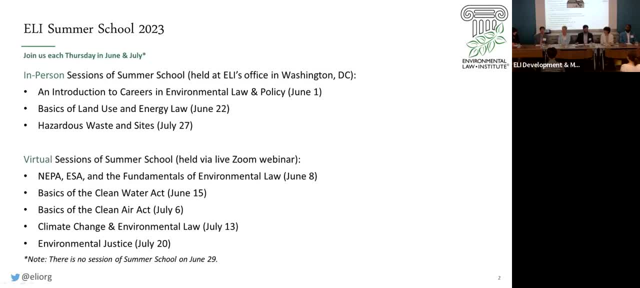 immediately decided to switch to history. So you can see how sort of tightly I held on to that dream. So, growing up I had sort of always been interested in the outdoors. My family took a trip up to the Lake Superior, Michigan every year and I always had a sort of close connection. 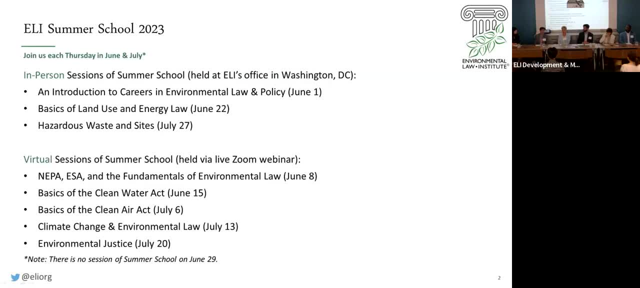 with the wilderness. But I found myself in history. So taking classes in University of Wisconsin was my way to art history. actually Graduated with a degree in art history decided I wanted to sort of pursue a graduate degree in that topic. That was sort of the best way to find a job and 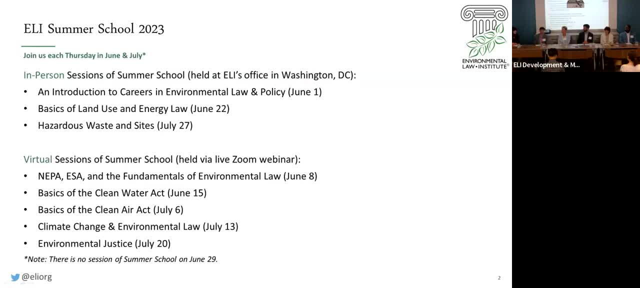 a career with that major. So I did that. I spent two years getting a graduate degree from the University of Kansas in art history, studying Dutch art of the 15th and 17th century. I know you're all thinking, okay, well then how does he figure his way into the environmental law? 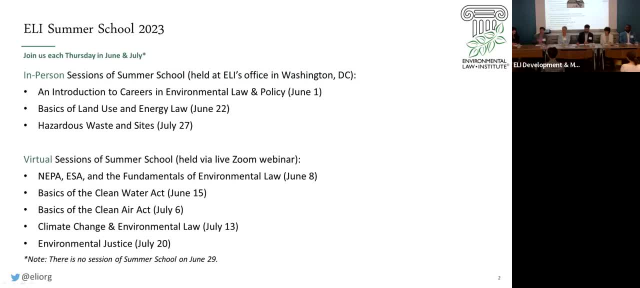 Well, that's a great question. I think that's a great question. I think that's a great question. So I moved out to Washington DC and I got a job, actually just two doors down at the National Geographic Museum, And so that was a way to sort of use some of my skills and knowledge that I had. 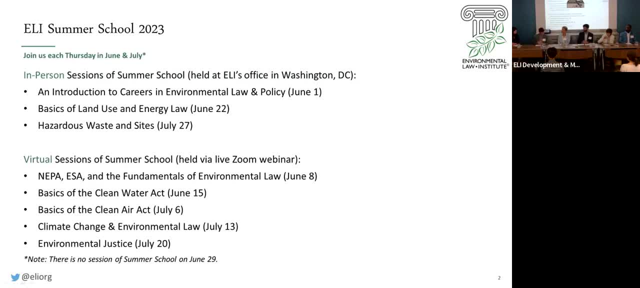 learned in art history but also marry it with some of my interests in the outdoors. But I worked there for about four or five years and kind of made my way maybe to the top of where I could in my trajectory. So I was like: well, what else can I do? 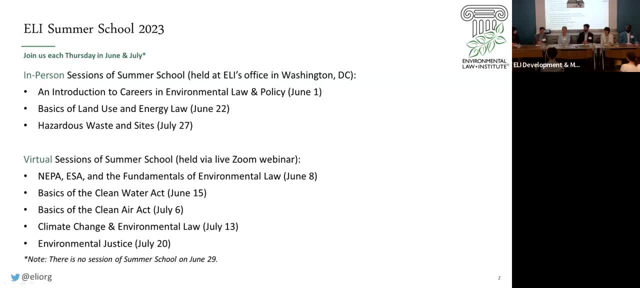 if I want to do something else with my career and with my life, And I had been reading a lot in the National Geographic magazine about climate change. I was aware of that but knew it was a sort of pressing issue of our time And so decided to go back to school and sort of do something with the 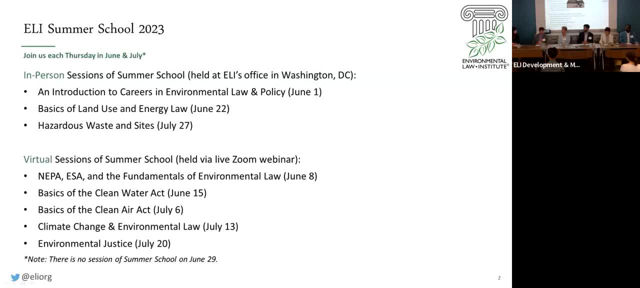 environment. But I didn't know what that meant yet. So I actually went back to the University of Maryland to get a Bachelor of Sciences degree to sort of get some of that science coursework that I had immediately. I immediately dismissed my first day of college and that was really. 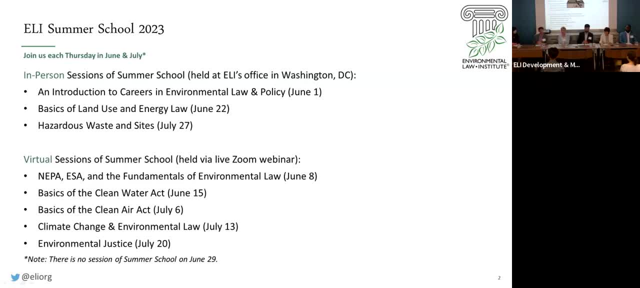 formative. So at the University of Maryland I sort of got in touch with a few professors there who helped crystallize my thinking around what I might want to do in the environment And I had never considered law or law school or being a lawyer as something I'd be interested in. 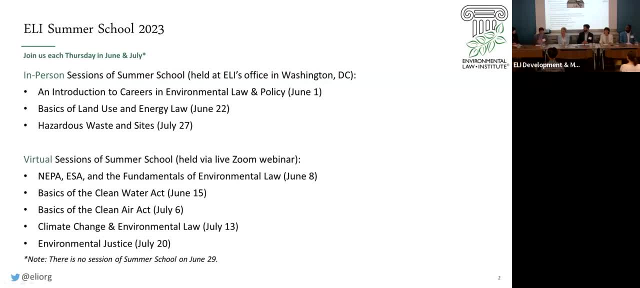 No lawyers in my family hadn't been exposed to you know the law at all. But I realized after talking more to some of my professors and who became a mentor to me, that policy and law was a really good way to sort of maybe achieve some of the things I was hoping to. 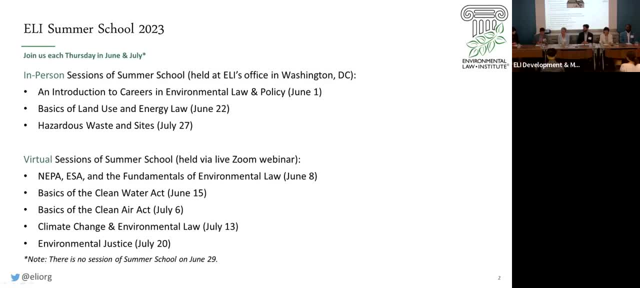 achieve with my interests, And so I finished my Bachelor of Science at Maryland. I took the ELSA and applied to law schools. I went to GW- just you know- here in town and lived there with a dedicated Dannemann program, and you know what did I look for in law school. 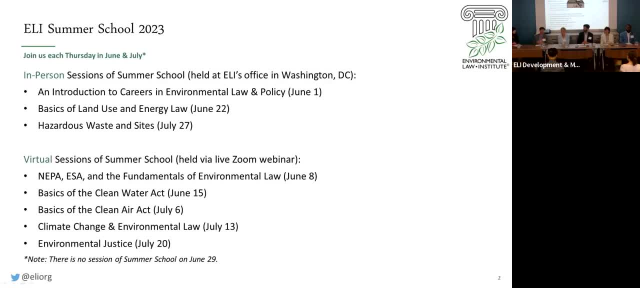 Well, I trained for the ELSA program and then, you know, I happened to be a law student for the first year in high school And then I was able to study law. So there's a lot for a law guy to do there, but it's pretty much as simple, as kind of you know one thing you have to do. 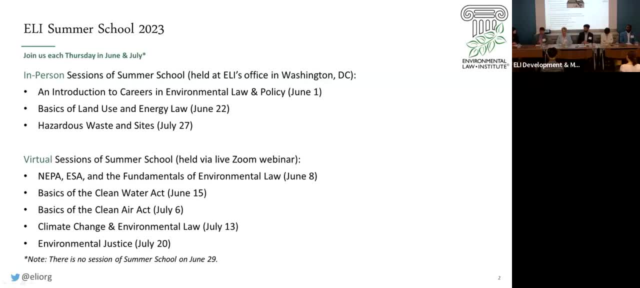 in law school, Then I got a from one of my professors there at Alabama And then I got into law school atnesota and I'm now an alum at Minnesota. but I've been teaching law since I got my master's degree at University of Maryland and so I'm really 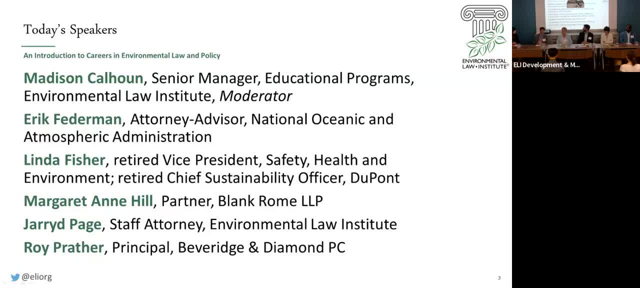 excited about law as a profession- Environmental Policy Act. I also sort of took advantage of all the externships that were available in law school and actually did a clerkship here at the Environmental Law Institute between my second and third year of law school, And that was really when I knew. 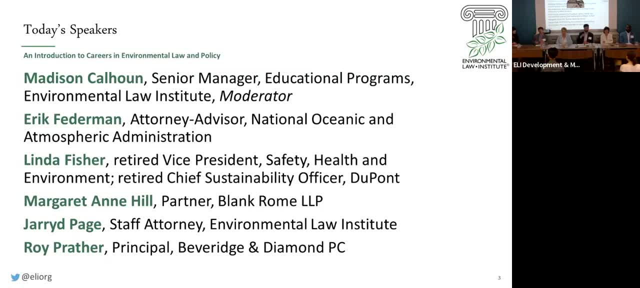 Environmental Law Institute was the type of place that was doing the work that I wanted to do, And so, after law school, applied for a fellowship here at ELI, got the fellowship and then sort of continued on as a staff attorney, And then I've been a staff attorney here for almost three years. 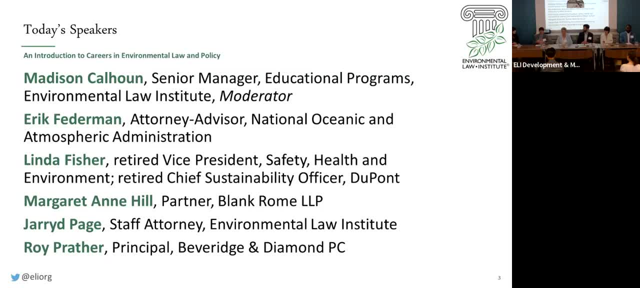 And here at ELI I work on several projects, both domestic and international law. Sort of the largest project I work on and the one I spend most of my time on, is the Climate Judiciary Project, training state and federal judges about climate science. 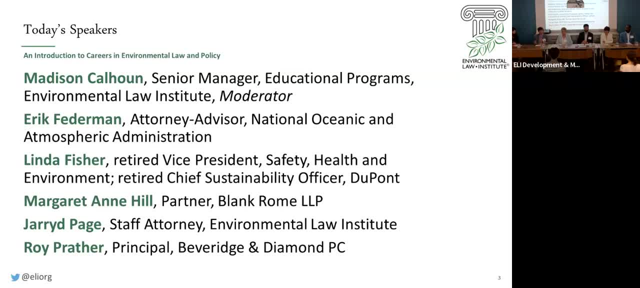 and the law. I also work on issues of coastal resilience, natural infrastructure and climate win intelig spending, And I've been a little bit more involved in the industry, And so I've been working with Velocity and Know И, as well as Southwest fossees to 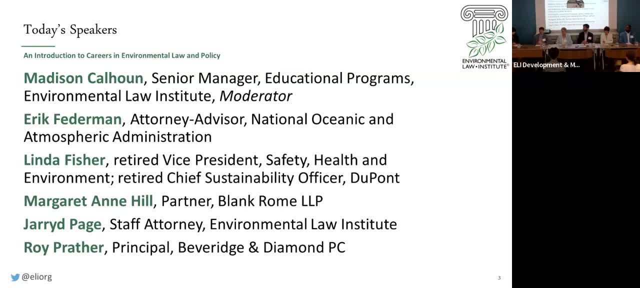 and public lands resource management. So a long, circuitous route, but I'm really excited to be here and to talk to you all today. Thank you so much, Jerry. Our second speaker today is Margaret Ann Hill, who's a partner at Blink Room. 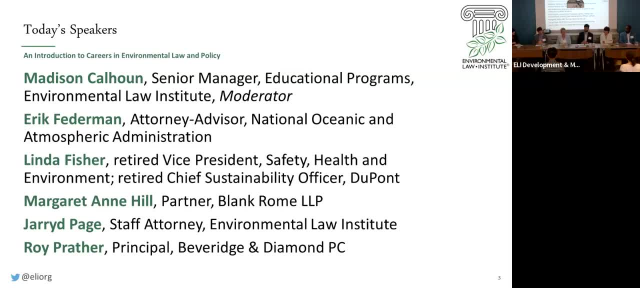 Or Blink Room, so I'll hand it over to you. Good afternoon to everybody. Also a pleasure to sit here and talk to you about environmental law. I've been practicing now for a long time- for 39 years- in environmental law and have done pretty much almost everything. 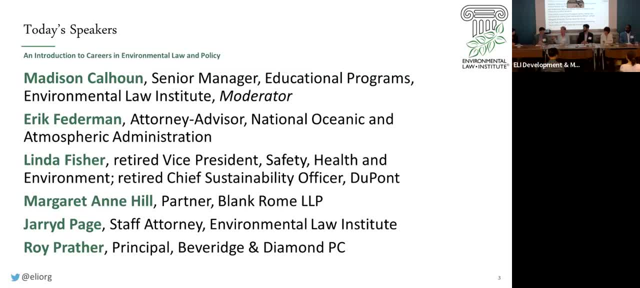 you can do in that area. Like Jared, it was interesting hearing your story. I also have a very circuitous route in that, similar to you, I didn't know anybody who was a lawyer growing up. I didn't have anybody that could mentor me. 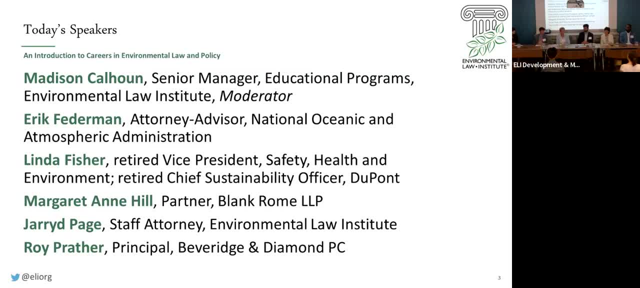 I did know that I was interested in law For some reason. watching television, whatever, it just seemed like: oh wow, that looks pretty interesting. Didn't want to be a dentist, but So anyway, went to college, got out of college, 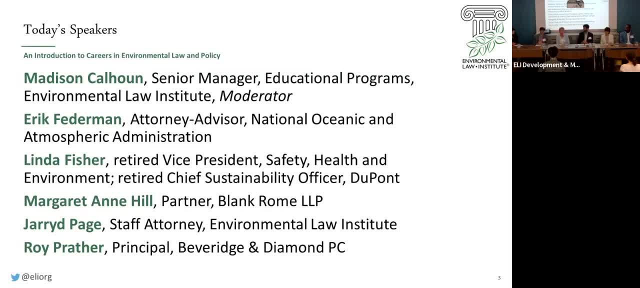 And at that time wasn't really sure about going to law school. So I ended up going to graduate school in Northeastern in Boston and got a master's in political science and was also trying to figure out: okay, now where do I go from here? 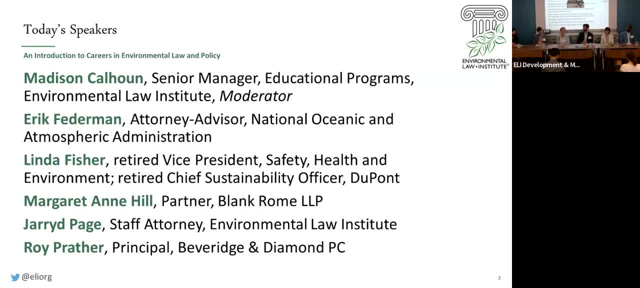 And at that time a former oil corporation- you may have seen the signs around for it still because somebody bought the name to it. They divested some time ago- but a company by the name of Gulf Oil Corporation. They operated in Pittsburgh. 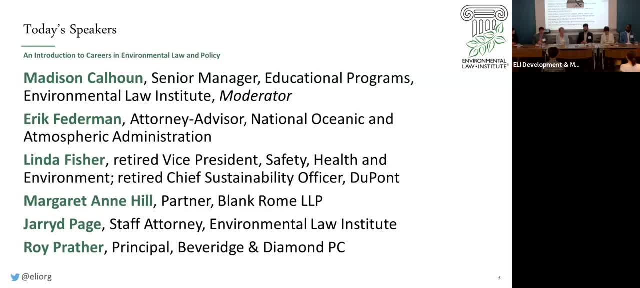 They were headquartered in Pittsburgh. And after getting my graduate degree, I decided that I was really interested in working for an international company, because I was interested in politics, government relations, international relations And since Gulf was located all over the world, I thought, wow, that'd be a great company to work for. 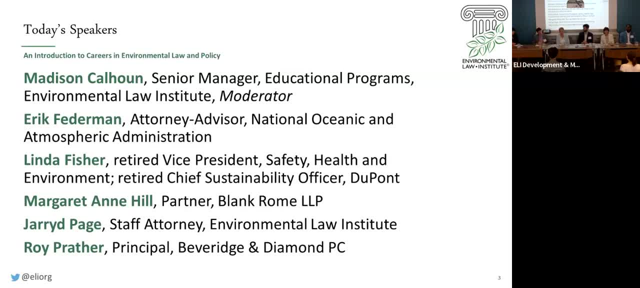 And they happened to be hiring at that time. So I applied for a position there and I ended ultimately in a really unique position. not intending to have this position, but it was really unique in that I was on the floor, the senior executive, where basically what I did- 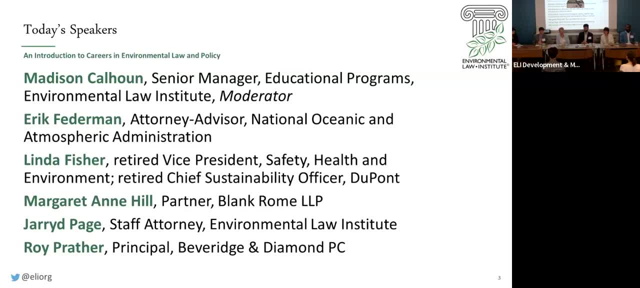 and three other people that work with me. we evaluated what to do with assets worldwide, basically looked at corporate strategy. I happened to be assigned to two what they call strategy centers, which were subsidiaries. The one subsidiary was Gulf Oil Exploration and Production. 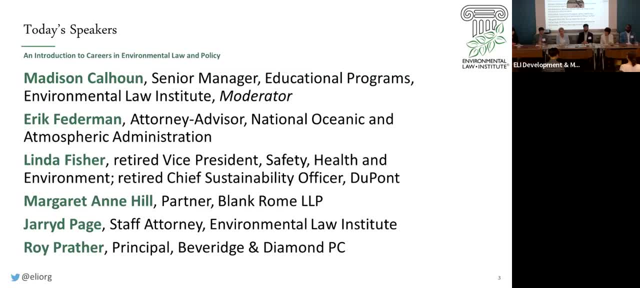 And the other one was Gulf Mineral Resources. So totally involved in activities that relate to environmental law and to environmental regulation. So I became immersed in understanding about everything with respect to environmental law, because obviously that's going to impact a corporate strategy, For example. back then, 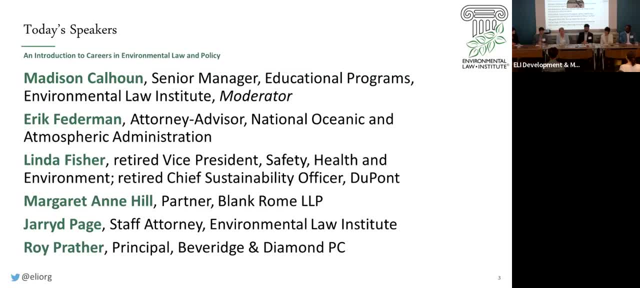 one of the things that I was very involved with was offshore oil leasing off the coast of California and working with some of our state and federal lobbyists, not only in California but also here in the district, in terms of things well, for example, bills. 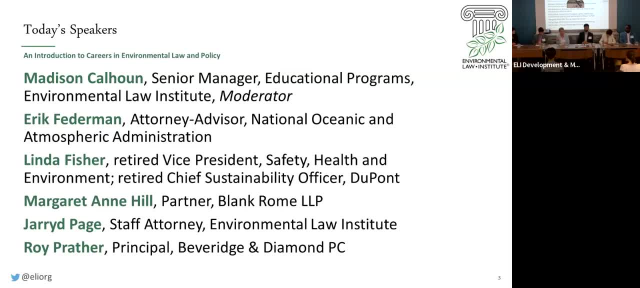 rodders that were being added onto appropriations bills to stop offshore leasing. So it was really everything and anything. And I also got involved in nuclear energy because Gulf did have a nuclear subsidiary at the time and they also had uranium mines, they had coal mines. 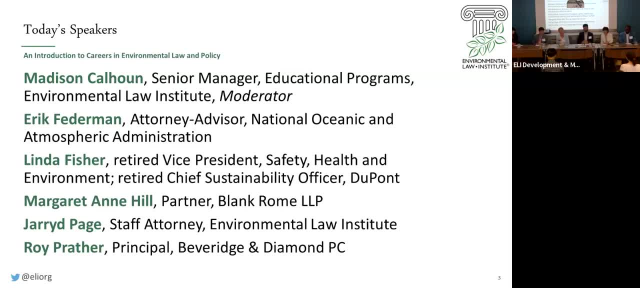 So there was so much stuff going on with respect to environmental laws that I realized I definitely had an interest Now. concurrently, what I didn't mention was I started going to law school at night. it was a full-time evening program at the Duquesne University in Pittsburgh. 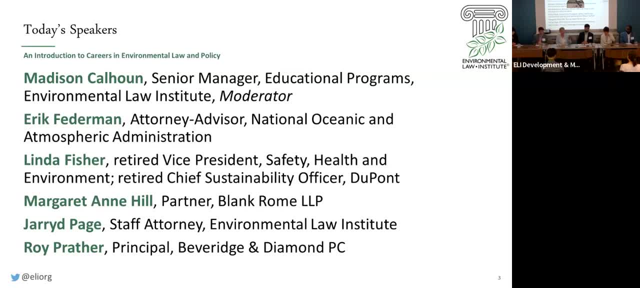 in Pittsburgh. So as I was working at golf in that area and the corporate strategy group and learning law, I thought, wow, this would be something I'd be interested in. Golf actually fell apart, The first oil company to do so- one of the big majors anyway- back in 84. And their 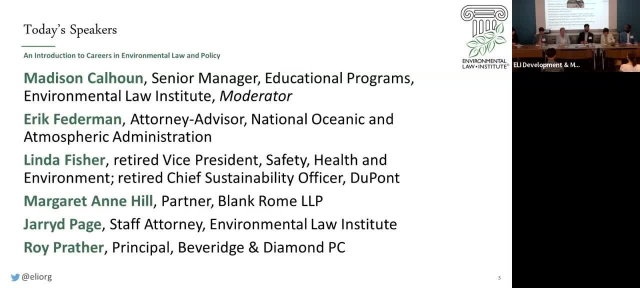 assets were sold off to Chevron And I ended up trying to figure out: OK, now where I've been here for eight years Now, what do I do? So the Department of Justice, of course, was taking off in terms of enforcement of environmental laws at that time And they were hiring here in the 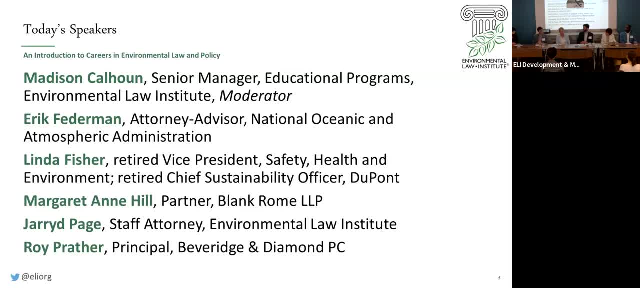 district. So I was hired by the Department of Justice. I came down here and I worked for several years at the Department of Justice And the interesting thing there is, first of all, for anybody that's interested in practicing environmental law, great opportunity at DOJ. 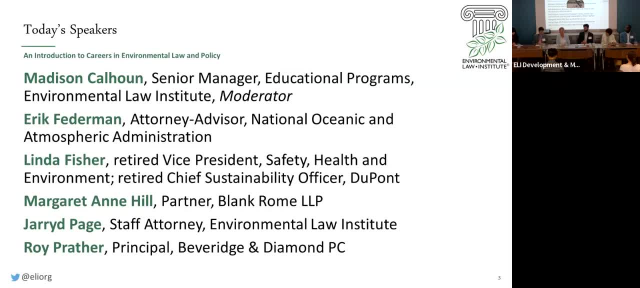 because you really do everything and anything And all the government agencies are your clients, So EPA would be our client, Department of Interior would be our client, Et cetera. So that was really a fascinating time, And while I was at DOJ I was given the 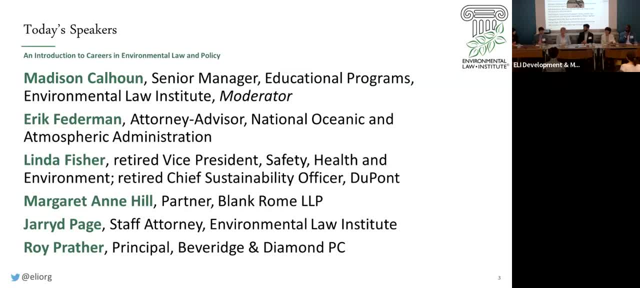 opportunity to do appellate court arguments, appellate briefs, work with the Solicitor General's office- what we refer to as the SG's office- in terms of preparing cases to go to the Supreme Court. Also, I got a chance. you're not supposed to when you're at DOJ, but I was up on the hill a. 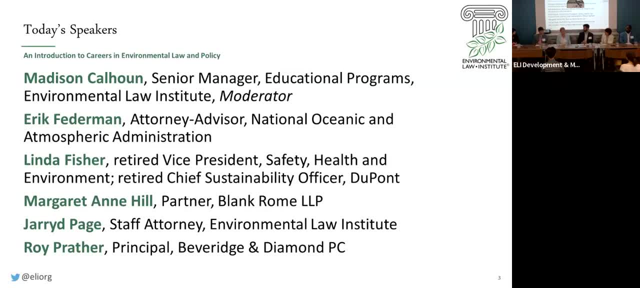 lot trying to make provisions to the Superfund statute at that time- The amendments to Superfund in 86. So I was just doing bobbing basically on the hill and doing a lot of other work, policy work- to a DOJ Decided that I wanted to pursue more litigation than what. 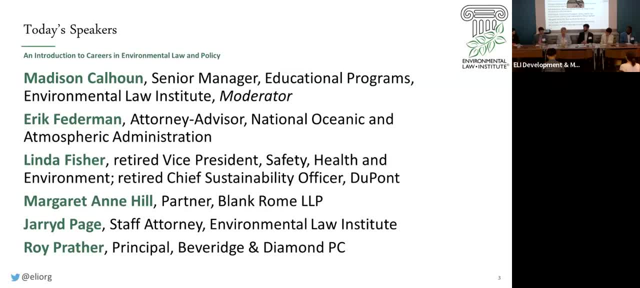 I was actually doing. I was doing some litigation, but I wasn't doing as much as I wanted to, So I went to a private firm here in the district and then ultimately worked here for about in a private firm for about 12 years and then ultimately moved up to Philadelphia to work for. 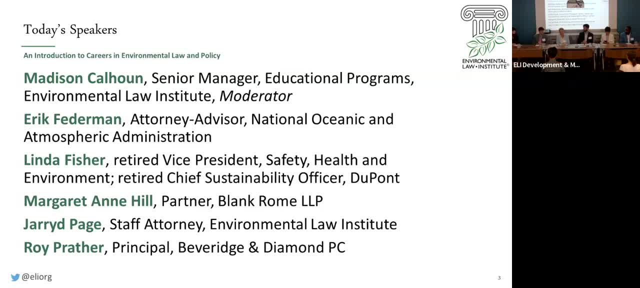 Blank Room And I've been doing pretty much everything and anything in environmental law- And you'll probably hear everybody talk about it today- but it encompasses many different areas. So some of the backgrounds from what I've been doing- transactions, litigation- 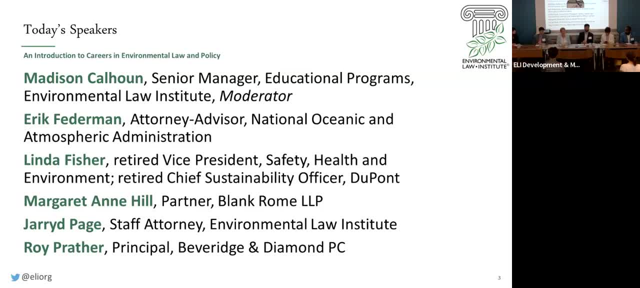 compliance work, and you know I was still doing some lobbying for some time, but that's how I got to where I am. Thank you so much. Up third is Eric Fetterman, who's an attorney advisor at the National Oceanic and Atmospheric 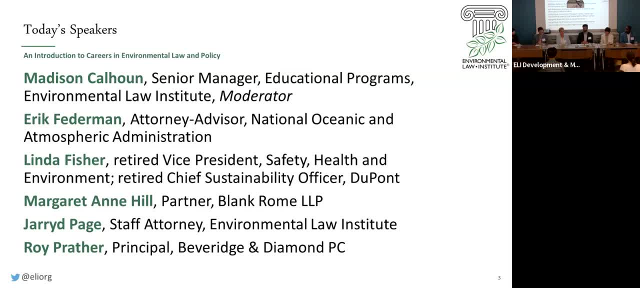 Administration. His name is Noah, and thanks a lot to you. Yeah, thanks and hi everybody, I'm really excited to be here with you today. Like Madison said, my name is Eric and I'm a lawyer at the National Oceanic and Atmospheric. 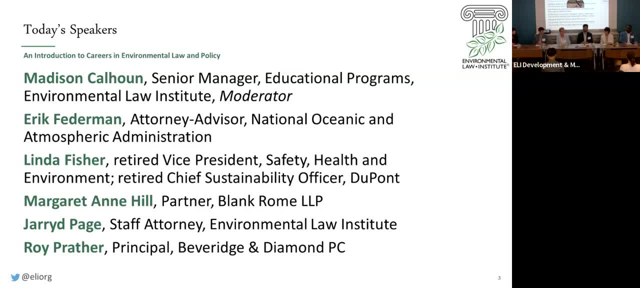 Administration's Office of the General Counsel. I'll talk a little bit about how that organization's structure, I think later in my introduction. but I've been there about three years. I also had kind of a circuitous, aimless path to the law. I thought I'd have a unique story up here, but I guess it's the. 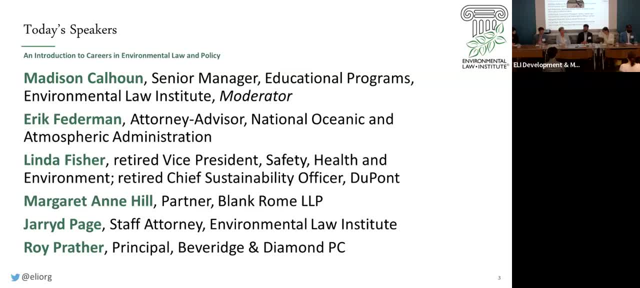 norm. Like well, unlike Jared, I didn't know what I wanted to do when I went to college, but I found myself studying history and classical literature. So I did a lot of like Greek and Latin and Roman history And graduating I decided I wanted to pursue a graduate degree, maybe be an. 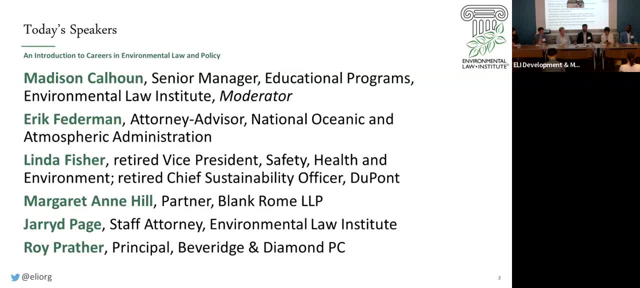 archaeologist. But I spoke to a lot of people in the field and they said that I should take a couple of years and make sure that's really what I wanted to do. So after college I taught English in Spain for a couple of years- kind of sit and think about my future- And during that time decided. 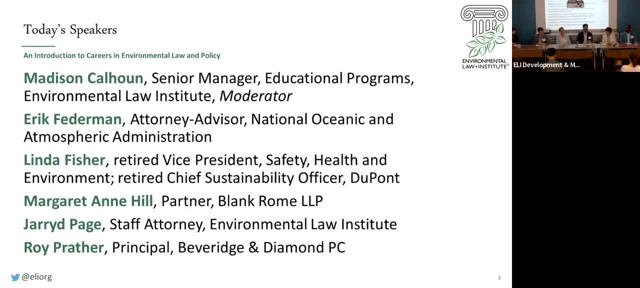 that I wanted to do something with my career that gave me the opportunity to have more of an impact on the current day, And I think I was resigned to the law. given the skillset that I developed in college, It seemed like the only thing that I could do, with kind of the emphasis on research and writing that. 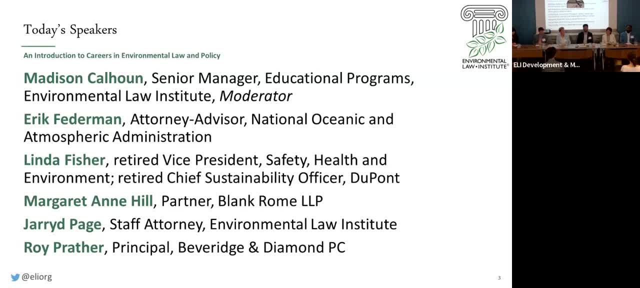 I developed. So after those two years I decided to apply to law school and was lucky enough to be accepted to Harvard. So I started law school in 2015, and even then didn't really have a clear picture of what i wanted to do with a law degree, just that i wanted to be in the public sector somewhere. um, 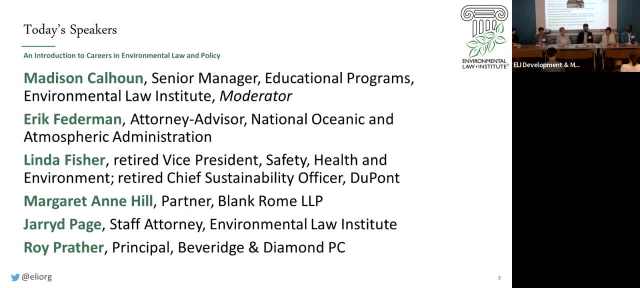 very quickly, though. after i started, i realized that environmental law was really interesting to me, and it and it gelled with personal interests. like jared, i also spent a lot of time in the outdoors as a kid and was passionate about conservation and natural resource management. um, and as i started taking classes on environmental law, i one learned that i really liked the people. 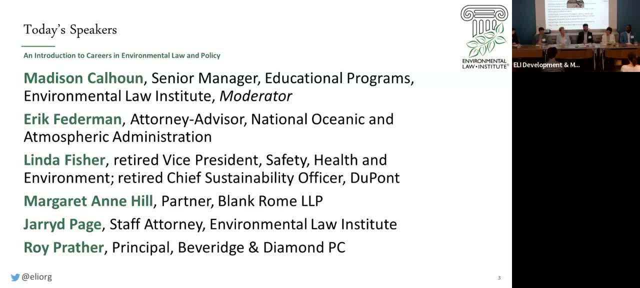 um, that i was taking those classes with and that that were teaching them um, but also that i found the subject really stimulating and that it was something i found compelling. so in law school, i tried to take all the classes that were available to me, um, in environmental law, including administrative law, um. 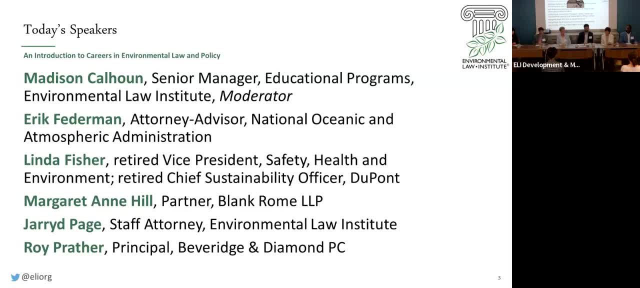 and i also, um, really tried to prioritize kind of experiential learning, so i was able to spend some time in clinics in law school. um, uh, both. there was an environmental law specific clinic that i spent a semester in, but harvard also had a food law and policy clinic that i spent some. 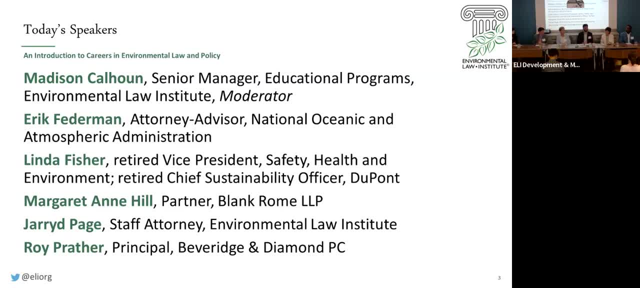 time in um which had a lot of crossover with environmental law and environmental justice. um, i spent my first summer- well, i spent both summers interning um at non-profits. uh, the first summer in philadelphia for an organization called the public interest law center of philadelphia, which is kind of a small regional impact litigation shop. 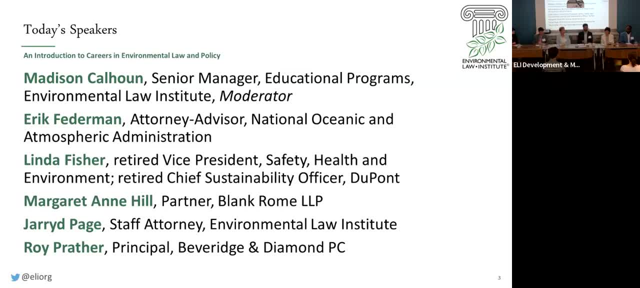 that does do some environmental justice work, but does a lot of other stuff as well. um, and then my second summer i spent with earth justice, um in their northern rocky's office in bosnia montana. i also did kind of a mid-semester externship with the department of justice's. 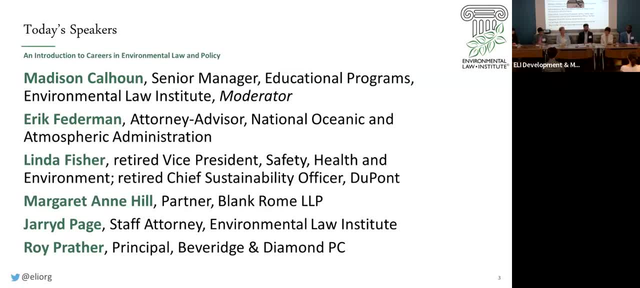 environment, natural resources division. um, let's see, i graduated in 2018 and didn't have a job. well, i did have a job. i didn't have like a career job. i clerked for two years, first um on the supreme court for the state of alaska and then for 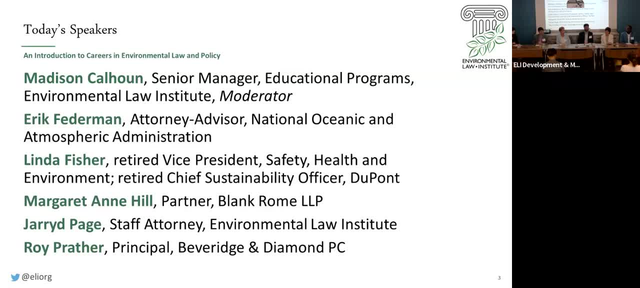 the district court in anchorage. so i had two years in anchorage, um, and then i had to start thinking about kind of where to go. after that. i knew that i wanted to do environmental law in the public sector. but, um, maybe we'll cover this later. but it can be a little overwhelming and hard to find a. 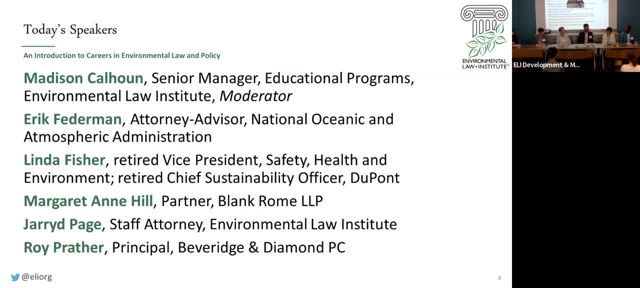 job, um, so i applied all over the place, inclusive to doj, which did not accept me, um, and ended up actually being referred to NOAA's Office of General Counsel by a professor that I've taken classes with, And I didn't know a ton about NOAA. although, living in Alaska, I had started to 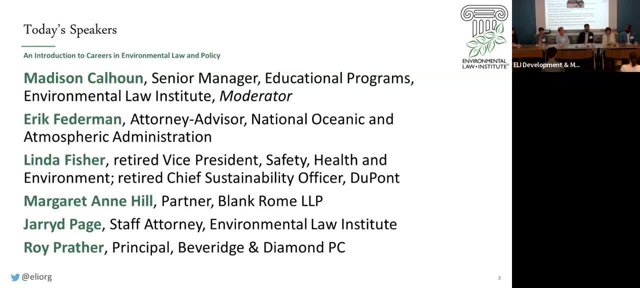 appreciate how big of a role the agency has in many things, including fishery management, which is a big issue up there, and kind of weather data, weather forecasting and climate study. So I was accepted into NOAA General Counsel's Honors Program, which hires people either straight out of 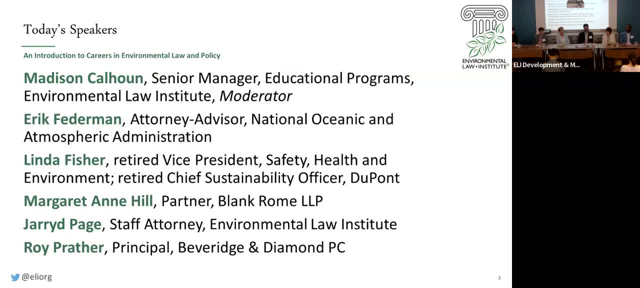 law school or a couple years out of law school, like me, who had clerked or had other fellowships, And the way the program is structured. well, let me take a step back. NOAA's a really big organization. They do a lot of stuff. They're a bureau of the Department of Commerce, so they're not their own. 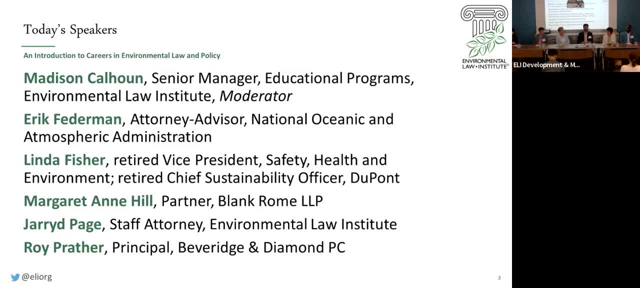 agency, But NOAA itself has a super broad mission. I don't even know all the things that they do. It ranges from fishery management to weather satellites And the Office of General Counsel to track. that is very broad as well, and it's split into 13 different sections. 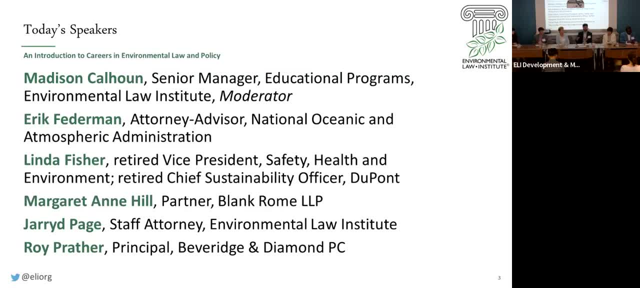 each of which works with its own set of kind of NOAA program clients. The way that the Honors Program is structured: when you're hired into the organization, for the first 18 months that you're there you do three six-month rotations. 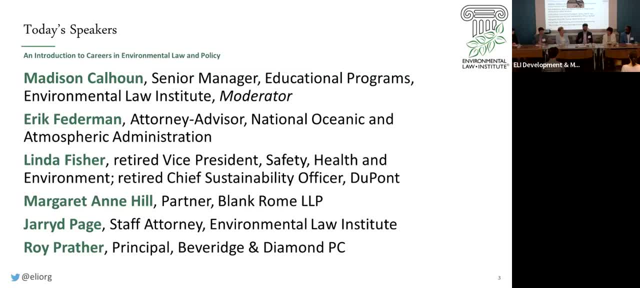 this all sounds very complicated in different GC sections. So over the course of those 18 months I spent time working with the National Marine Fisheries Service, which implements the Magnuson-Stevens Act, which is the big fishery management statute. 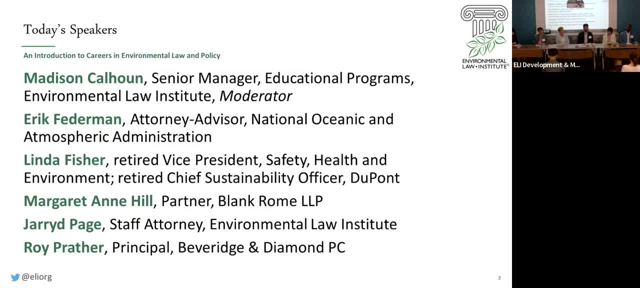 and also implements NOAA's responsibilities under the Endangered Species Act and the Marine Mammal Protection Act. I also spent time with NOAA's GC's international section, which kind of represents the whole understanding of theグر черкbé renown map, represents the whole agency on any number of international law issues and also supports NOAA's participation in international treaty bodies like the International Maritime Organization. 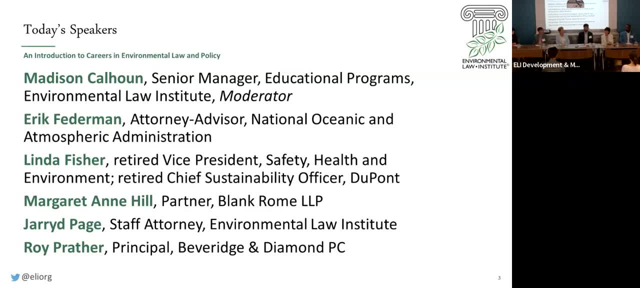 And I spent time also with the oceans and coast section, which is where I was assigned permanently and where I work today, which primarily advises the National Ocean Service, which itself has a bunch of program offices and has a very broad mission, but I'd say the client that I spend the most time working with is the Office of National Marine Sanctuaries. 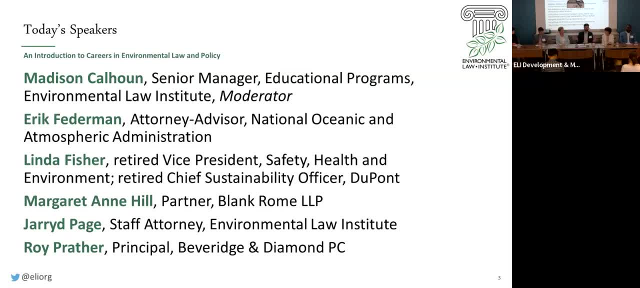 which administers kind of a system of marine protected areas across the nation, And a lot of really interesting legal issues are associated with that. So I'm excited to talk more about that, I think, later and to share my story with you all. 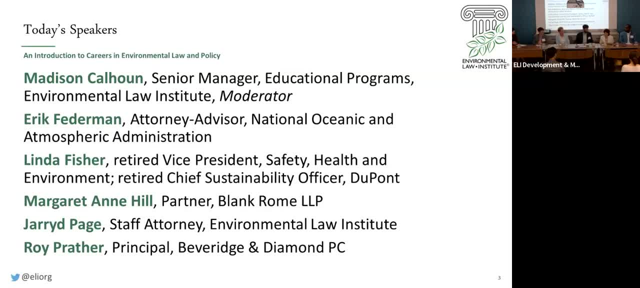 You are getting a very broad view of career paths. I'll tell you that right now My name is Linda Fisher. it's also a pleasure to be here. I graduated from Miami of Ohio, also a history major, and loved policy and politics growing up and came to Washington and got a job on Capitol Hill. 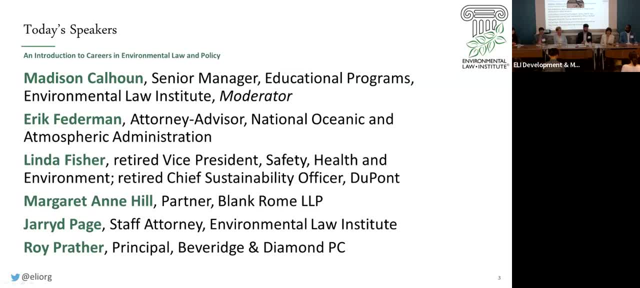 And I did that for five or six years and realized that to advance my career I needed to go to law school. But I was also, as so many staffers on Capitol Hill are was bitten with a political bug and thought I might want to run for Congress. 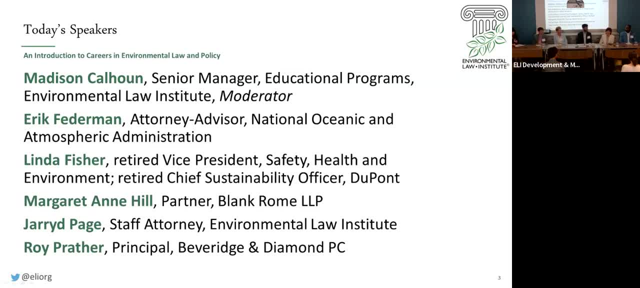 So I went to Ohio State, which is my- Columbus is my hometown- Worked on a couple of local campaigns while I was going to law school and realized I loved public policy but I hated campaigning, And so I graduated. we're going to talk about networking as part of the panel. 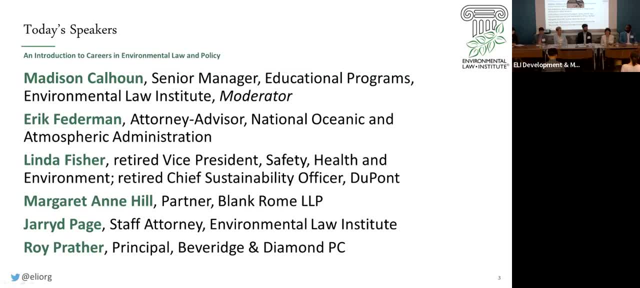 and had a job with a small company, A small law firm in Columbus, Did not get- I was a clerk. I did not get a full time job because- wait for it- I was a woman And they weren't hiring women at that point. 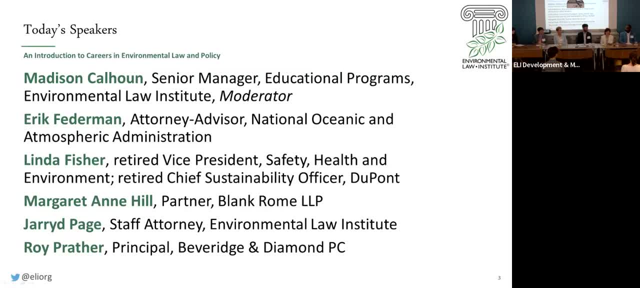 So connected back up with an old boyfriend in Washington and he said: I think I know of an opening at EPA. EPA had just let a lot of political people go. I had Republican credentials and they were looking to hire people And I took the job at EPA. 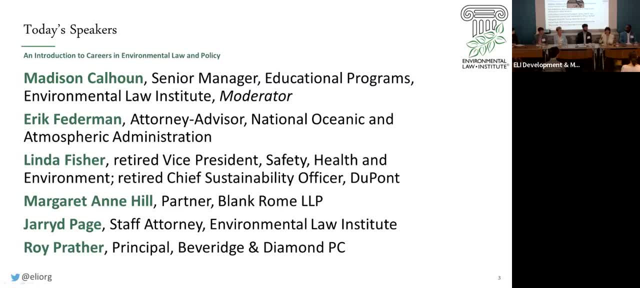 I had not. I had an introduction to environmental law working with the Energy and Commerce Committee, but I hadn't come out of law school with any classes, Partly because the laws were so fresh. they really weren't teaching a lot of environmental law at the time. 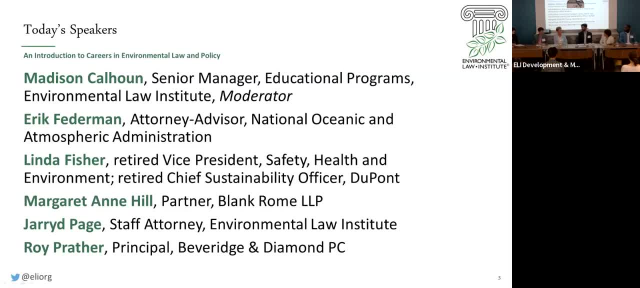 Like Peg, and I finally figured out where I knew your name. It was working on Superfund amendments in 85 to 87 or 86. I was chief of staff to the administrator of EPA and I did a lot of legislative work, Spent two years with her colleagues at the Department of Justice pushing amendments through the law through the Congress, which I think really set up the practice of environmental law for years to come. 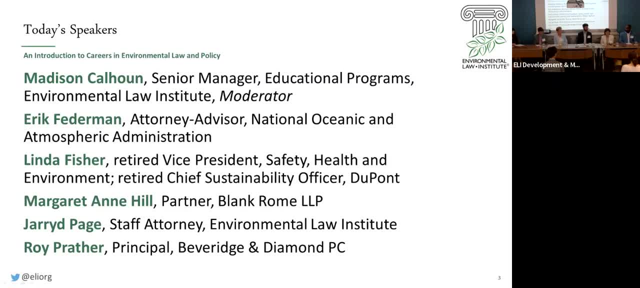 I stayed at EPA, the Republicans continued to win the administration. So after being chief of staff, I ran the policy office For a couple of years. then I became the assistant administrator of- at the time it was called the Pesticides and Toxic Substances Office. 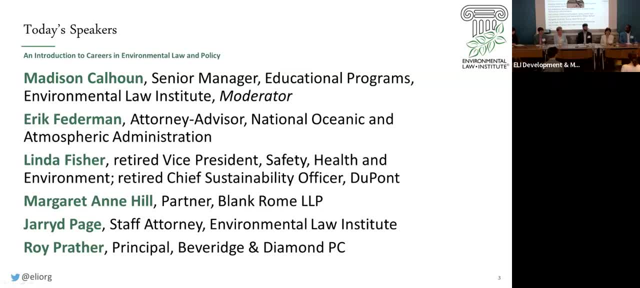 And then the Democrats took over and I spent two years at a law firm because I decided I really did need to punch the ticket for the career path I had started out in. While I was at Lake Menloikens, one of my clients was a lawyer. 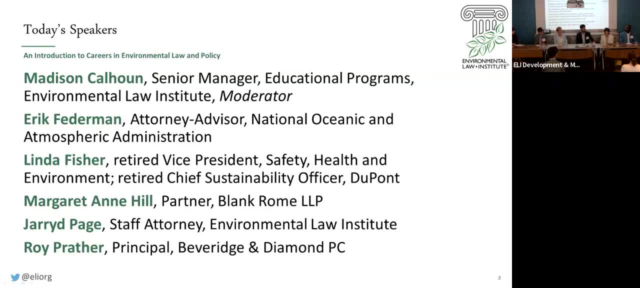 He was a lawyer And he was very well-known in Los Angeles. So one of the things that struck me when it came to the DHS program was when my clients approached me about coming to work for them. It was Monsanto and I was hired to run their government affairs program. 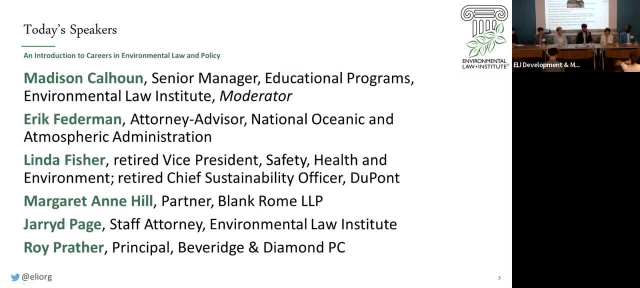 I then left Monsanto- They merged with somebody- and it was a good time to leave- And got hired back when George W became president as deputy administrator at EPA. I left after two years and took a year off, spent some time with my kids and got approached by DuPont. 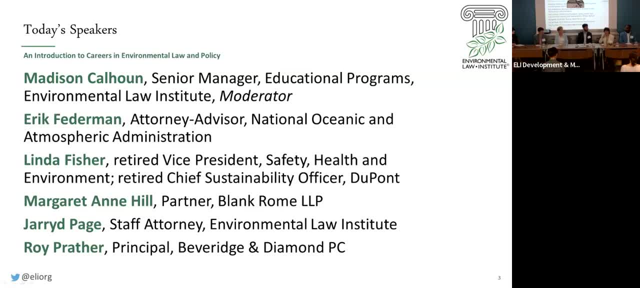 And at DuPont I was hired as, according to Headhunters, I was the first chief sustainability officer at any Fortune 500 company And it was fun to be in kind of a path-breaking role in corporate America. I also ran the safety, health and environmental programs for DuPont, as well as the sustainability programs. 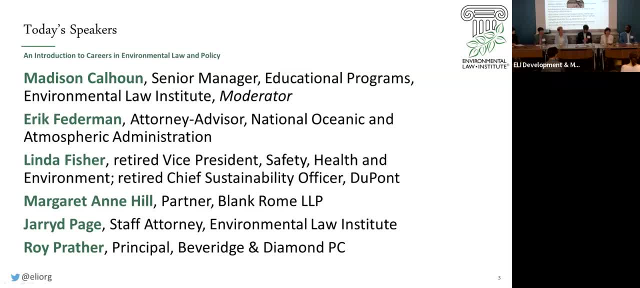 I retired from there about five or six years ago and have been serving on boards of directors ever since. So kind of a checkered path in environmental law. Somebody asked me the other day about administrative law and my experience with administrative law And I laughed and said I never took. it was actually the dean of Ohio State Law School. 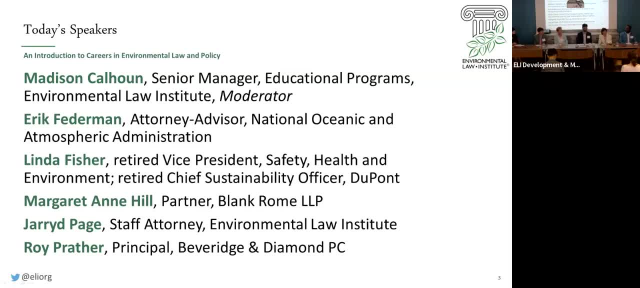 That's his area of expertise And I said: you know, I did a lot of administrative law- writing laws, reading regulations, signing off on things- but I never took admin law. I learned it on the job, So thank you. 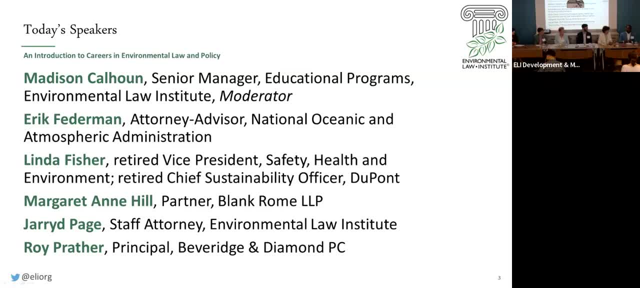 Do you have a normal path? Relatively speaking, it's a straight shot, Or at least to the law, but not necessarily to environmental law. So good afternoon everyone. My name is Roy Frazer. I'm a partner at Beverage and Diamond, which is the oldest. 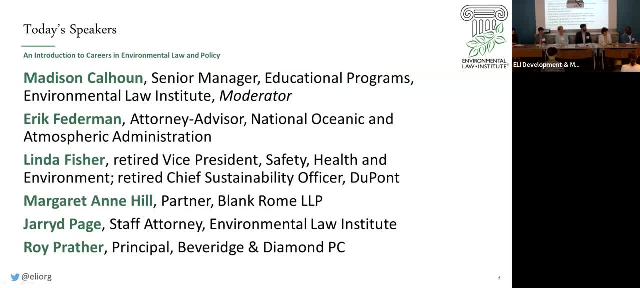 And largest law firm dedicated exclusively to practicing environmental law, So it's all that we do. In terms of my legal career, however, basically I knew I was going to be a lawyer, probably by the time I was in high school or something. 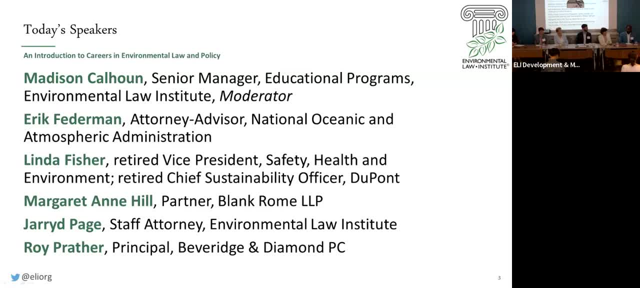 At least that's what I had in England When I went to college. I went to the University of Pennsylvania and was an international relations major, which was basically history, economics and political science, So A little bit of a trend there. but coming through university I basically had already determined I didn't know what I'd be doing. but I just liked the idea of the law because over the course of college it became clear to me that it touches everything. 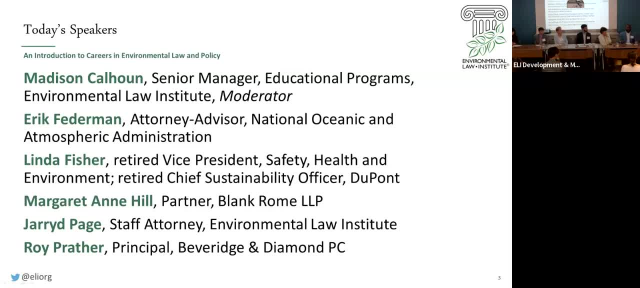 And so, even though I didn't know yet what I wanted, I knew I'd be able to find something that fit my interest, And so I went directly from undergrad to law school. I attended Georgetown, And while there I did not take a single course on environmental law, even though it has an entire environmental law program. 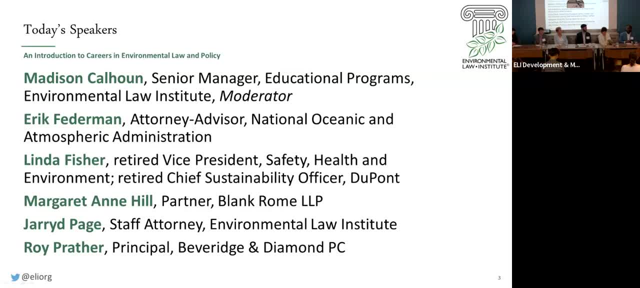 I did take admin law So. but basically I knew from that experience after spending a summer at the public defender's office in Atlanta, which is where I'm from originally- that I did not want to do criminal. And then I spent another summer at a law firm in Philadelphia that I enjoyed a great deal and they gave me an opportunity to 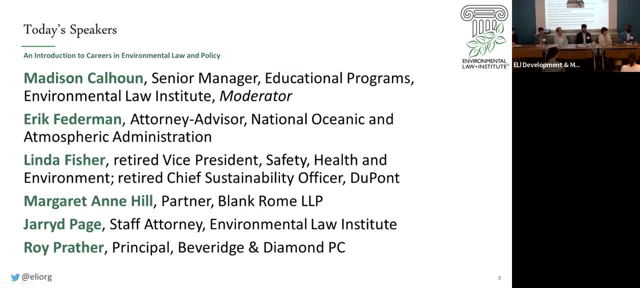 I started to kind of experience a wide range of things And I realized I definitely want to litigate. And so, knowing that- and it being 2008, and basically the economy was crashing and they were still willing to hire me, I basically held on for dear life and jumped to Reed Smith in Philadelphia coming out of law school. 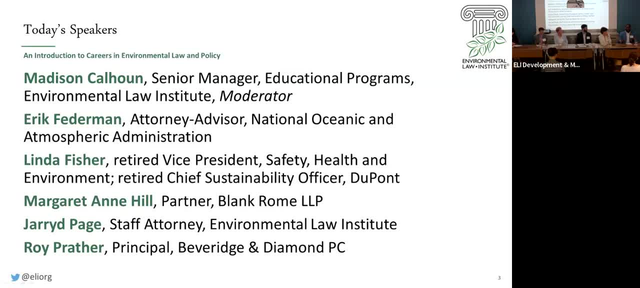 When I went there, I went into their commercial litigation group, which is basically just the litigators for the entire firm. So I did everything. I did labor and employment. I did business, intellectual property, I did no environmental. Well, now I had one super fun case, but I was. 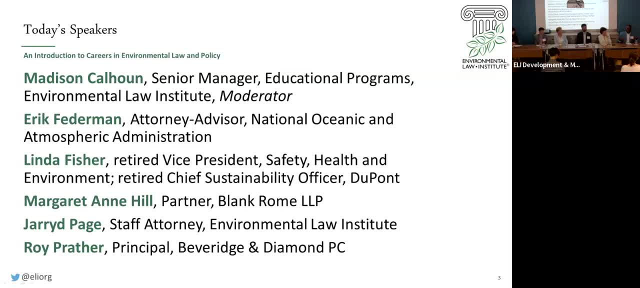 so junior that I only did like some very limited research And so I just didn't get a real good exposure to it, but got a ton of litigation experience And ultimately after four or five years I relocated to Baltimore area because my wife was doing residency at Hopkins and realized 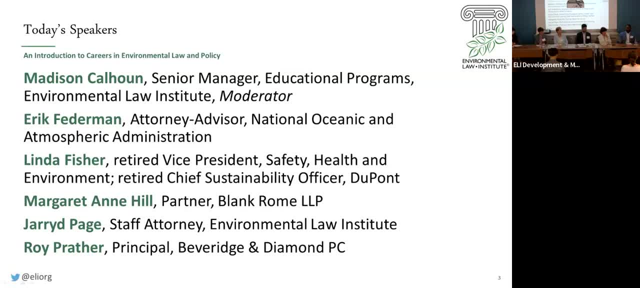 I wanted to specialize more. I didn't want to just do every other kind of litigation you could think of- and started thinking about what I actually had an interest in specializing in, And I had been doing a lot of patent litigation at the time, Mind you, with no science background. 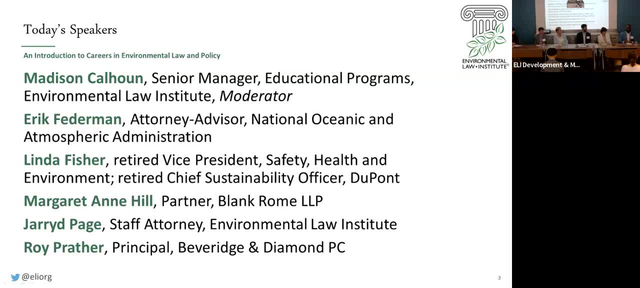 whatsoever. I actually avoided taking math at all while I was an undergrad- music theory, which was the hardest class I ever took, So it was a terrible idea. But basically I just started asking around and the people mentioned networking before, but talking to people in various 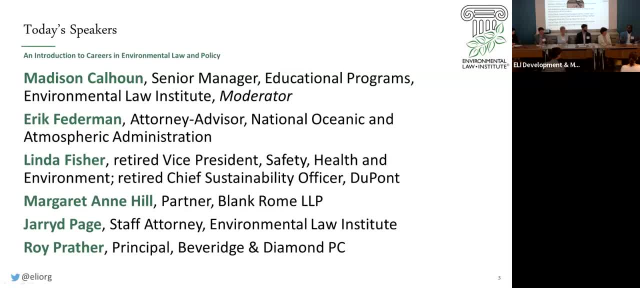 capacities And I realized in the patent litigation that I did what I enjoyed the most- and maybe it's because I didn't have a science background- is I was the person who worked with the engineers and translated to the judges, because most of the time those people were political science. 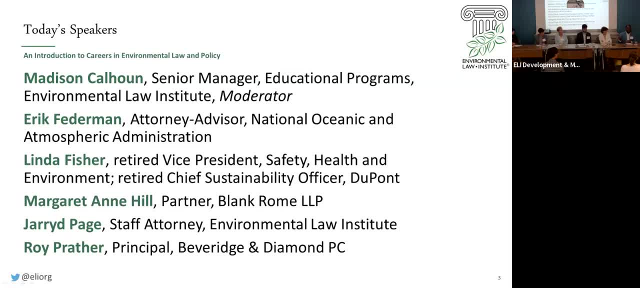 and history people right. So I could take that very complicated computer science or chemistry issue And, after a lot of studying, finally say: I think I have a general idea how this works and then explain it to them. And after talking to a wide range of folks about what I might be able to do, one of the people I spoke 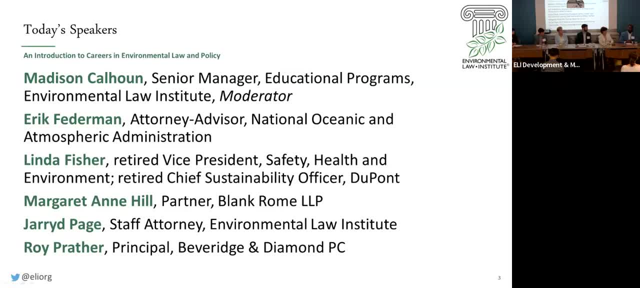 to was the chair of Benrington Diamond at the time, Ben Wilson, And basically he said we actually have a need for some associates with a lot of litigation experience. Would you be interested in environmental law? I hadn't really given it much thought, So he gave me some readings. 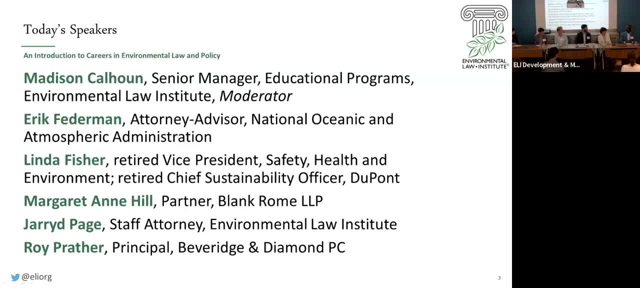 He said here: read this: Here's the kind of things that we do. Let me know if you have an interest. And so, basically, after looking at the cases reading, more cases reading I generally had awareness of, as everyone generally does like, climate issues, issues related to scarcity. 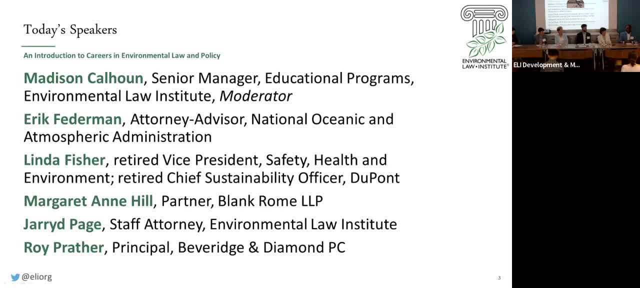 issues related to drinking water, right, Like. I had visibility of those issues but never really dug into them. But what really stood out to me was two things. A lot of the litigation that I had done largely involved fights about the moving money, right, Who's going to pay this other person money because business didn't go the way? 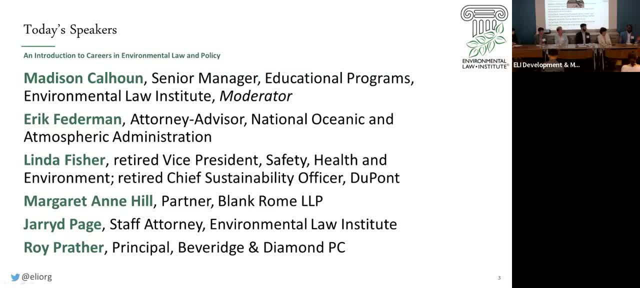 they planned, Who owes who what, That kind of thing. And which is fine, Don't get me wrong. But in terms of like broader impact that you might have with the work you do, sometimes it can be a little bit limited, right, And so in the environmental context, it gave me this opportunity to kind of 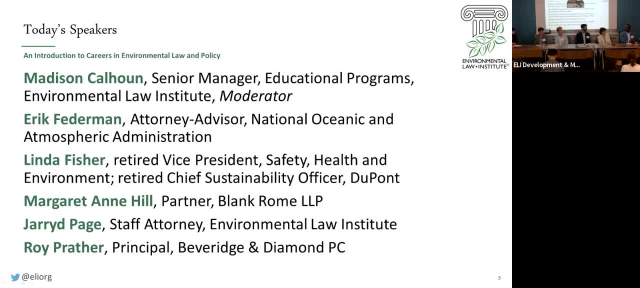 marry the technical piece of things that I really enjoyed with the intellectual property work that I was doing and do work and advise on. So part of what I learned is that it was really easy to have a good connection to people's lives. It wasn't as easy to say for me as it was for most people, but it was just you know. 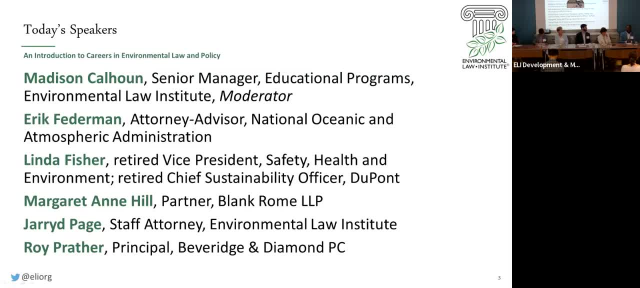 that there was a deep, deep connection that really made that connection pull me forward. My name is John R. Like I said, I had worked for the Cleaner Act for a year and had very few key statements and very few things coming, but I had very few issues that I could see a direct 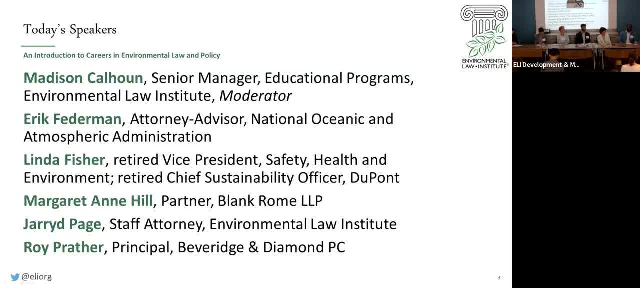 talking environmental um, or even just happy agency to touch right. so, uh, i joined beverage and diamond and have basically been practicing there for the last nearly 10 years now. um became a partner there. maybe after four or so years i was finally able to tell people that i was an environmental lawyer. 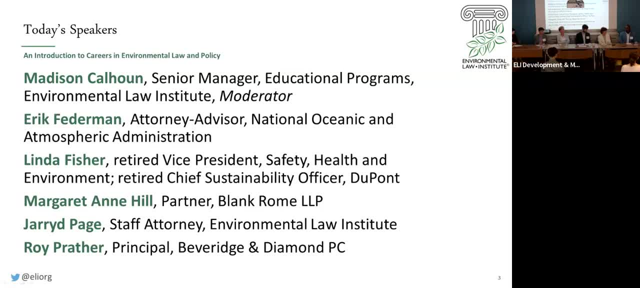 and actually be confident in saying that. um, and since then, my practice has been not just litigation but expanded to include um, you know, compliance counseling, which i get a lot of um interesting exposure to. i mean within probably a couple of weeks of being at beverage and diamond- i was 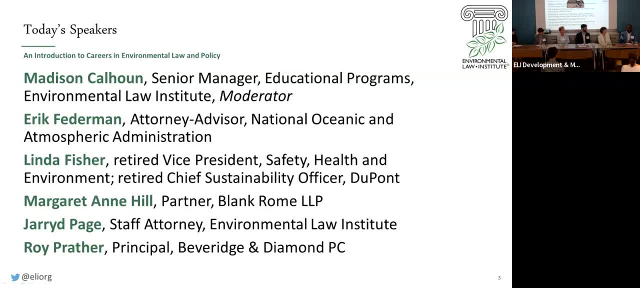 in maryland at a paper making facility, like with a hard hat and boots, like walking through, and they're showing me their process and how they dispose of their waste and you know what, what things they're going to need to factor into the renewal of their- you know, discharge permit like. 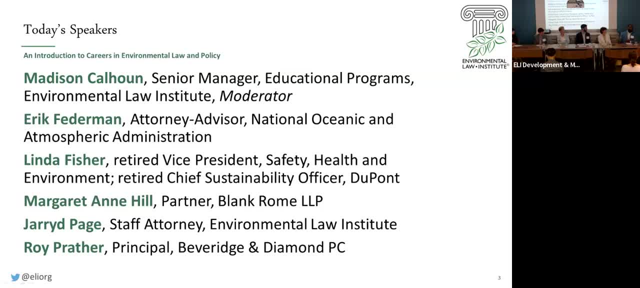 all these things. so it's always something new that i get to learn and then, at the same time, also be in the room to help weigh in on really critical issues, both for their businesses, for municipalities and for the people that live in the vicinity of where they operate. um, and on that last piece, my practice, i'd say, over the last five years or so, had really 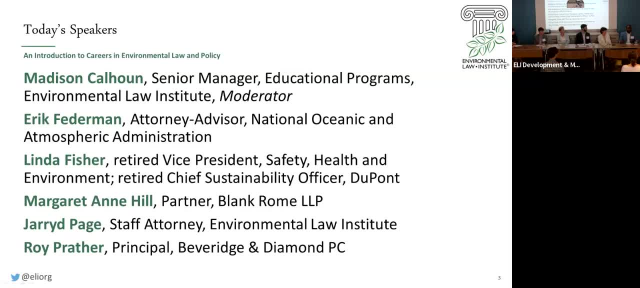 expanded on that compliance piece to really focus heavily on environmental justice right um which, for me personally, had a connection just with respect to issues that my own family faced, being in mississippi and other locations um, and so it offered a great opportunity for me to um advise, raise the visibility of certain issues that, you know, many times organizations have 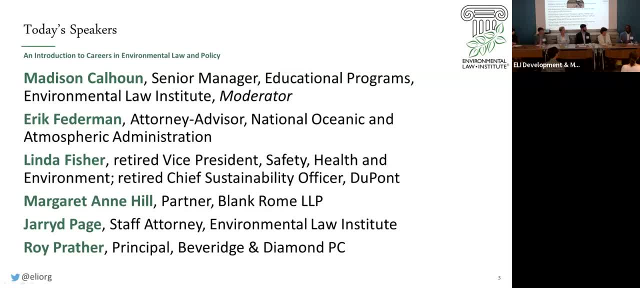 considered or factored in, but not always necessarily with the lens. that, i think, captures some of the nuances that are necessary to really make sure you're effectively addressing concerns of the community where you are, because there's no one-size-fits-all as it pertains to a lot of those. 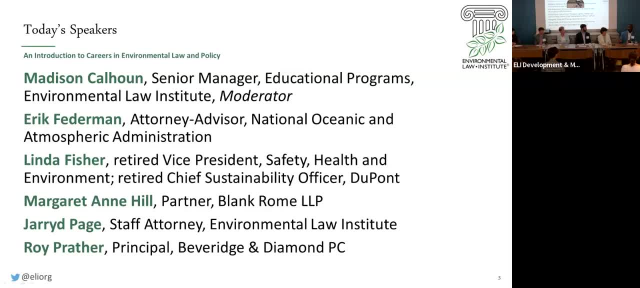 issues, um, and that led to me also going and teaching a course at georgetown on environmental justice, and so i've kind of come full circle and it's really just been an amazing experience. thank you all so much for sharing your journeys. i think the audience can tell how. 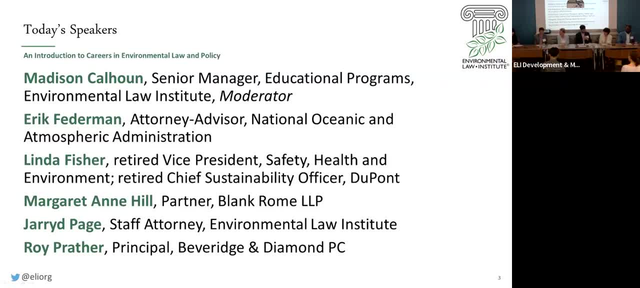 many different paths there are into environmental law, um, and so now we'll kind of move on to also all the many um different things you can do while practicing environmental law and how varied it is. so could you all speak about um your own experiences with environmental law in general and how you're 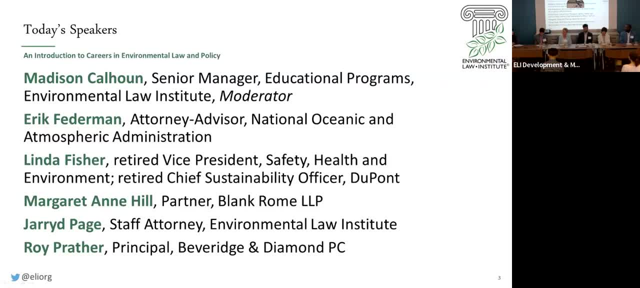 able to do that, and also, what's your experience teaching environmental law in georgetown? um, as a what a typical day at your job looks like. in any order, I'll jump in Only because I went back and I was looking at my. one of the things you have to do as an attorney at a law firm anyway, is you. 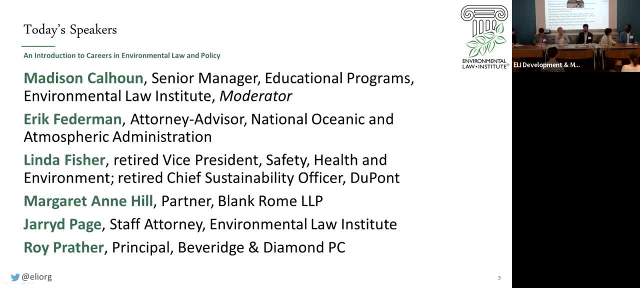 have to keep time. Really, you know, bothersome, but it's important because you have to build clients and that's how the firm makes money. So, in any event, I went back and I was looking at my time sheet, because I know I do a lot of different things during the day And I was 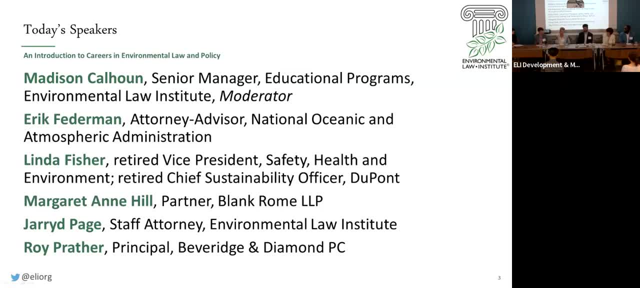 thinking, you know, if I could explain to you what I what a typical day might look like in terms of what I might do. Can't mention any client names, obviously, but I just went back and I looked at May 1.. What did I do? I negotiated a feasibility study language under Superfund. 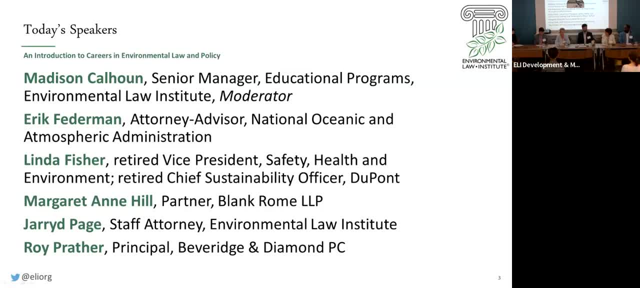 with EPA Region 2 regarding a Superfund site up in upstate New York. So it's a site that's been going on. literally it's been contaminated for 50 years, but the claim has been going on for about 25.. We just got to the point where we're actually. 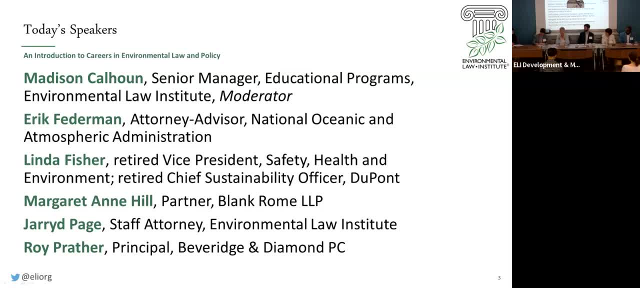 we're actually negotiating a feasibility study in order to get to what they call a record of decision, which means or tells you exactly how you're going to clean up the site. So those negotiations have been fairly intense, So I did that. The next thing I did was I've 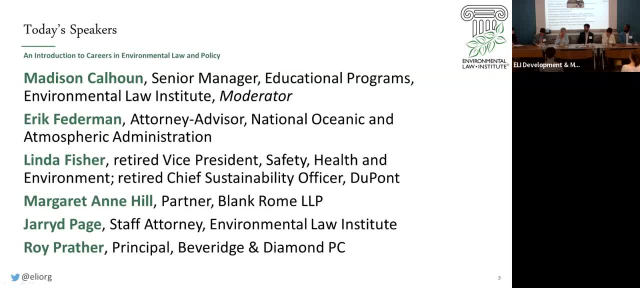 had been working with some consultants in terms of properties in California about trying to figure out how are we going to sell those properties. The properties are contaminated. So working with engineers, consultants, trying to figure out what's the strategy we're going to use in the 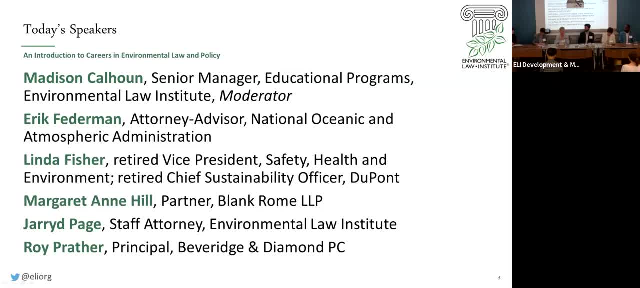 transaction in order to sell these properties on the on the sell side. What's going to impact the buyer? What is the buyer going to be concerned about? What are we going to do to preserve the value of the property and minimize the risk to the seller? We're representing the seller, So 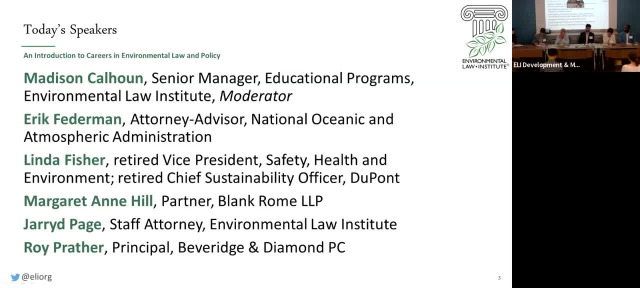 those were further discussions with engineers, consultants. I was also negotiating with New York State Department of Environmental Conservation, which is New York's EPA, on a site in the Kilvan Cull which is a very contaminated river. in terms of environmental conservation, which is New York's EPA, on a site in the Kilvan Cull which is a very contaminated river in terms of environmental conservation, which is New York's EPA. on a site in the Kilvan Cull, which is New York's EPA. on a site in the Kilvan Cull, which is New York's EPA. on a site in the Kilvan. 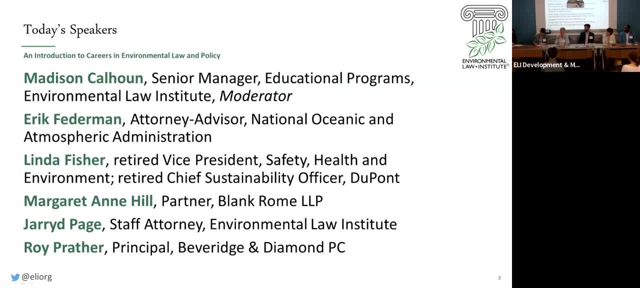 In terms of cleaning up sediment in the Kilvan Cull And also you know the legitimacy of that. Is that really something that we should be doing in this? you know, from my perspective, in this posh stamp sized area of a harbor and an entire river where there's a lot of activity's going on. 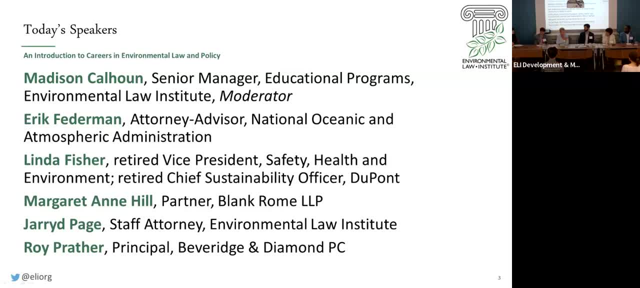 and also a river that was impacted significantly by Superstorm Sandy, So that was the only thing I did. We also represented a couple of lettuce companies which we think environmentally friendly lettuce company it's. it's all organic, um. however, that day i was trying to come up with some resolutions for wastewater treatment, because we're having issues. 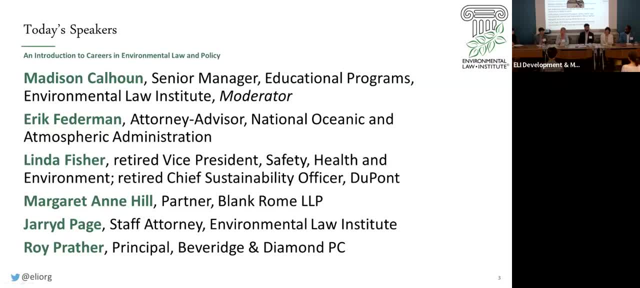 in terms of nutrients, um, that are generated as a result of lettuce production, and trying to figure out how we're going to manage off-site wastewater. uh, because right now, where we're discharging into a publicly operated treatment works, they're claiming that we're impacting it. so i work with. 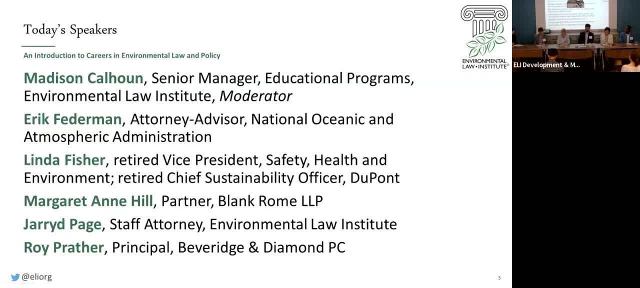 lettuce companies on various sites around the country. um also working with um osha negotiating with them on a parking garage collapse in new york city, um, which came down. unfortunately, someone died during the collapse. uh, there's now an ongoing osha investigation, so i worked on that. 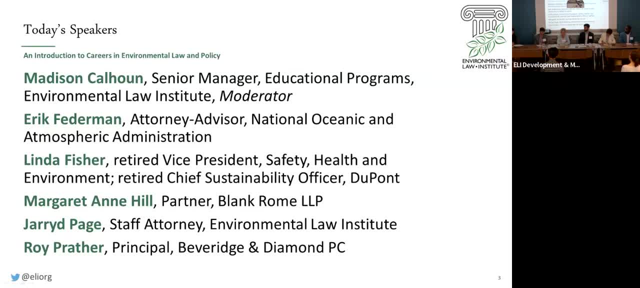 um, i also worked on a portfolio transaction involving a number of sale properties uh in new york state and finally, i was negotiating consent order agreement with the department of environmental protection of pennsylvania uh having to do with uh, the clean air act and petrochemical facility. 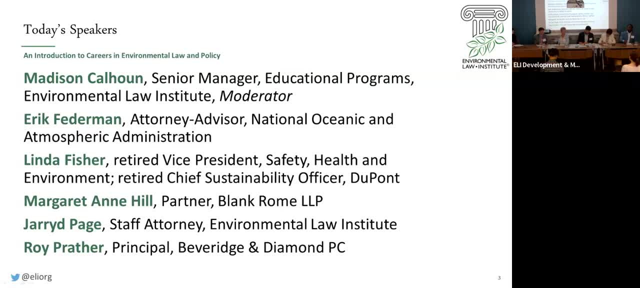 and flaring where they flare, basically excess gases, and flaring acts acts as a safety device. so that was just one day in my life. that was may 1. the thing i wanted to express. i was listening. everybody here is uh. from my perspective, one of the things i love about practicing environmental 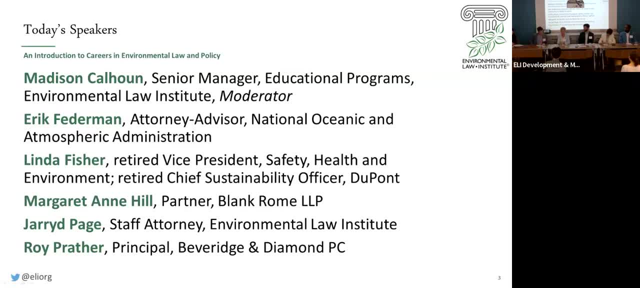 law and doing these things? is that, um, you know i represent industry, obviously, but i also represent municipalities and counties- is that when someone comes to the state and comes to you with an issue, whatever it might be the transaction or negotiating with the state, they have a problem and you need to think about that as a lawyer or if you're going to be a? 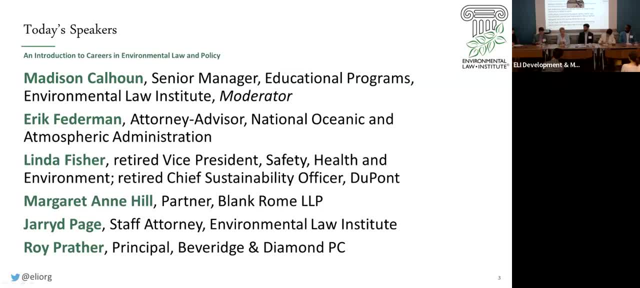 lawyer. someone has a problem and they're coming to you to help them resolve that issue and that should be taken very seriously by you. that someone is looking to you to to help them, it's like you know it, you know- i'll just analyze it- when you were, you know, a kid, you know going to your your. 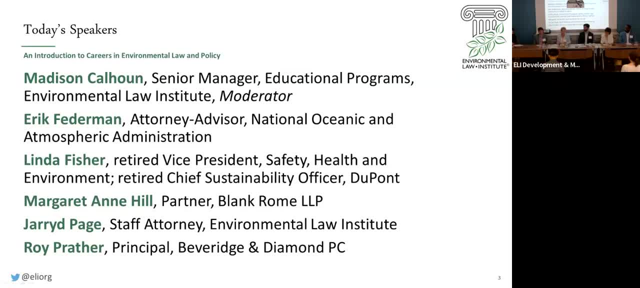 teacher, your mom, you know i have a problem. can you help me? i'm going to help you, i'm going to help you. help me how to resolve this. so it's a really big- uh, we'll just say- burden- but at the same time, it can be um amazingly rewarding to know that you're helping a client resolve some issue. 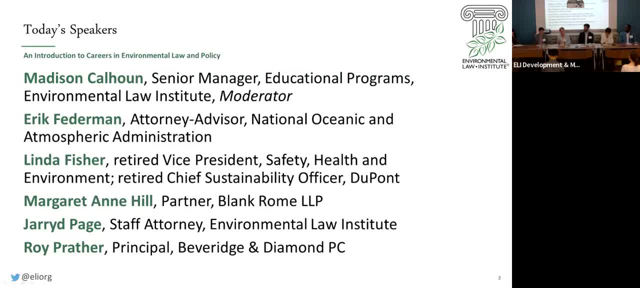 so that's the thing i enjoy the most is working with the clients and knowing that they're coming to me and they're trusting to me. you know, hey, help me. i need help with this. how do we resolve this? how do i get this, this property, sold, or how do i get this site cleaned up? and it's an. 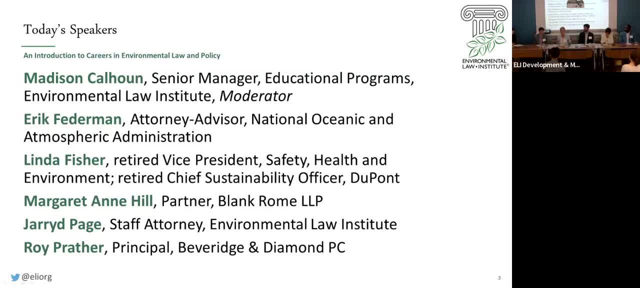 ongoing process, because none of well everybody on this panel will tell you you're going to have to do that. so at the end of the day, you have to work with the client to solve the problem. you can't be positive, you can't do this, and so you know i do want to be positive and i'm very proud of this. 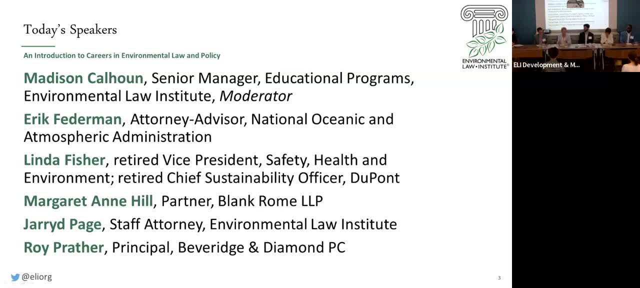 um and i've been working with the client for five years and you know i i'm proud of the um, the, whatever the time frame was. i'm proud of the work that they're doing with this and i think that's really important. so it's not something that we're going to over and over again and i'm not sure if 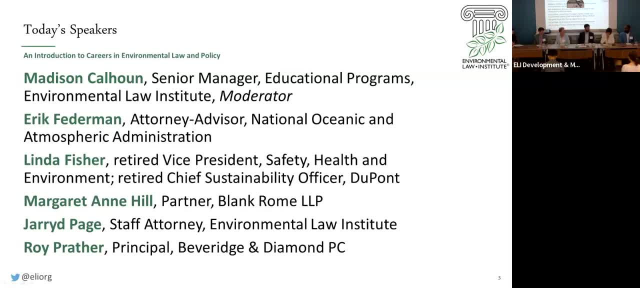 that's really what they're doing, but that's part of the process that i would encourage you to make in terms of your involvement with environmental law. i know that it's never like. you know it begins today. many different jobs, that that typical day uh was different, but they had certain things in common. so 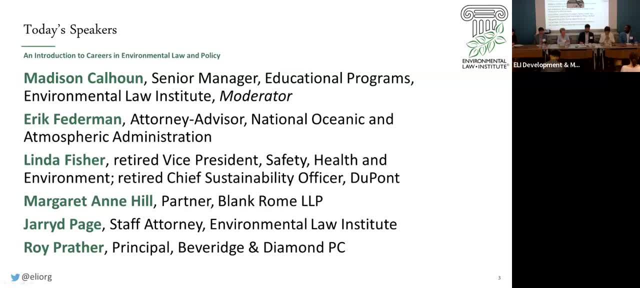 that's kind of what i the way i thought, uh, about approaching it. so at epa, um and erica, talk about whether it's the same. at noah, we used to joke about the fact there is a conveyor belt of issues that are coming at you. so the clean air act, the clean water act, super fund, the 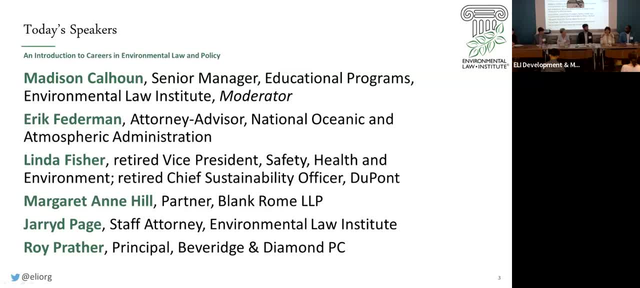 pesticides laws are loaded like with issues um rulemakings that have been mandated, um lawsuits that have resulted in something being remanded back to the agency, um controversial permit issues um that are coming up. there's just a conveyor belt, so every administration comes in and talks about what they're going to do and then they get hit with. the conveyor belt dictates what. 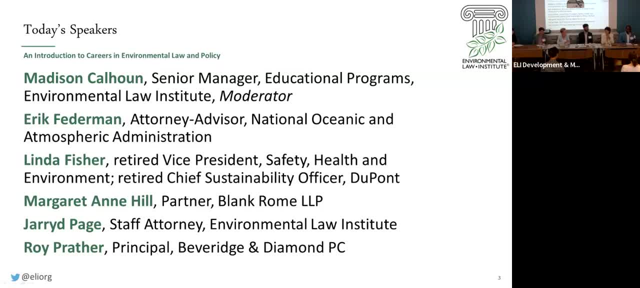 they really are going to work on. well, i was expiring. i ended up working on superfund 24: 7 my first couple years at epa, because that law had to get reauthorized. um. so so that conveyor belt presents difficult and controversial issues and um, at least the level i. 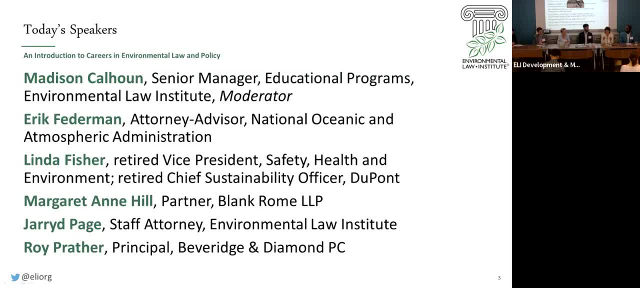 was at in the agency. i spent a lot of time meeting with people who had or would be affected by those issues or those regulations, and the one thing i learned- and i actually learned on capitol hill- is everybody has a voice and everybody has to be heard, and when you stop, 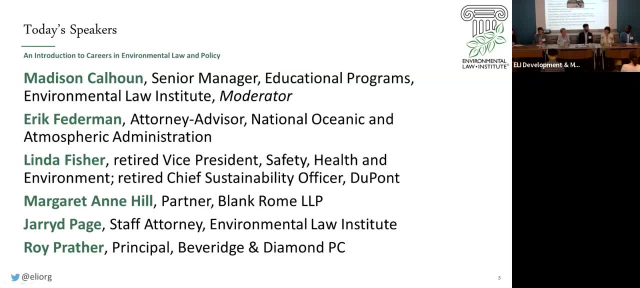 listening to people, two bad things happen and nothing good happens. the first bad things that happen are: you don't really know where your- uh allies are and where your adversaries are on an issue, because you haven't listened to them, um. and the second one is: you know, you learn a lot. 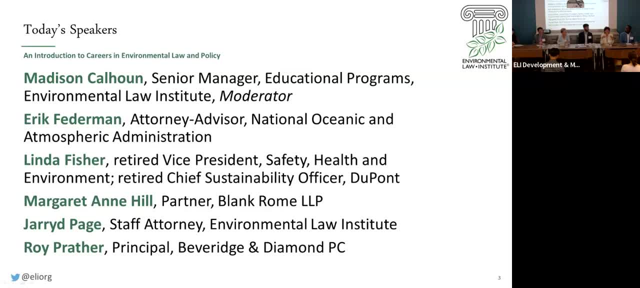 um that maybe what you thought isn't actually what is, and? um so i spent a lot of time meeting um with people, with corporations, with ngos, um, a lot of time on the hill talking to members of the congress, um within the administration. somebody once said the 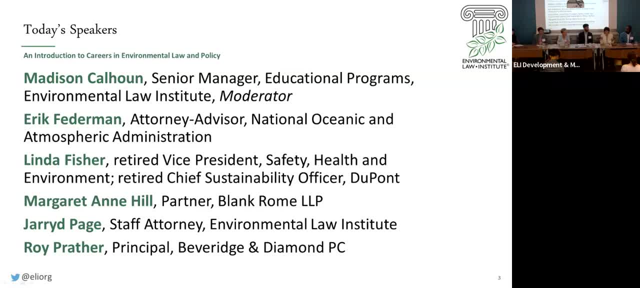 environmental laws are the most significant economic laws in america, and they are right, because we affect every municipality, every company and citizens every day. and so you gotta, you gotta, really factor all of that in um to the decision making of starting back in the rule making making process, and you have to be sure, as a senior leader, that you really are getting. 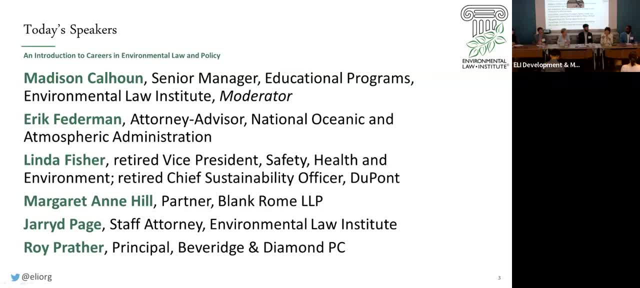 all sides, even within the agency. epa is not a model. if people don't- and this is a good thing- they don't see all the issues the same way, so you have a lot of internal debate and i think it makes for stronger rulemaking. my time in portland, america, in many ways, was quite similar. i worked 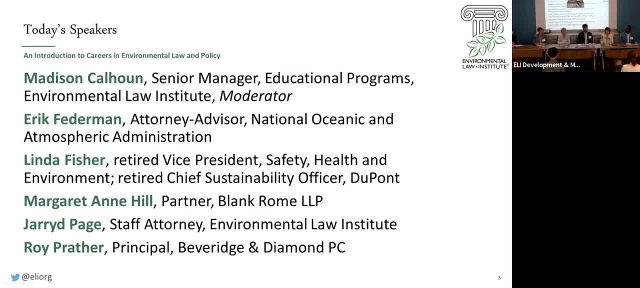 in companies that cared a lot about public policy. i worked in companies um. you might not necessarily agree, but really did care about compliance, being in compliance. They were there to use science and innovation to bring products to America. Getting in compliance was something both companies felt was mandatory. 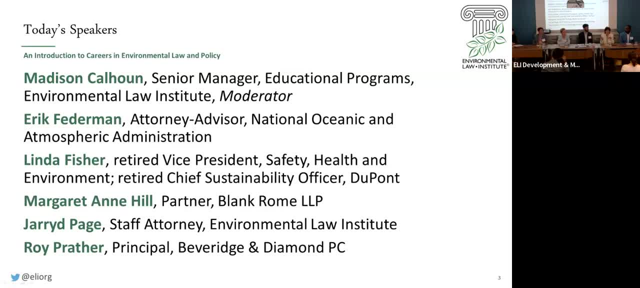 Their business was to create and sell. Their business was not to pick fights with the community or to have plants that weren't in compliance, And so I had an opportunity in corporate America to really help shape what was our approach going to be on controversial issues. 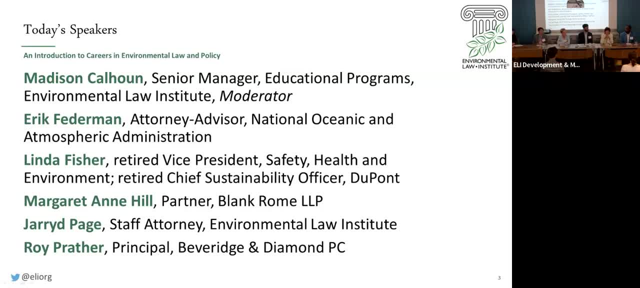 And those were everything from biotechnology at Monsanto to climate change at DuPont. DuPont had, long before I got there, brought the substitutes, had made CFCs. Montreal Protocol phased them out. They brought CFCs, They brought second, third and I think they're now on a fourth generation of refrigerants. 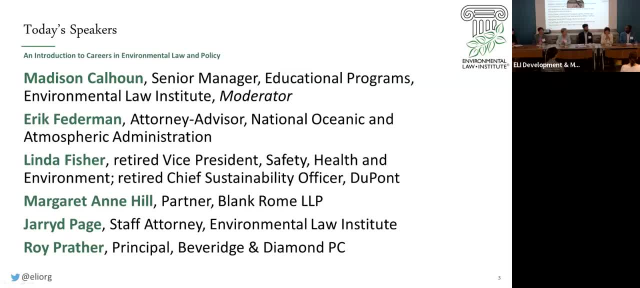 and new chemistry that is significantly improved over what CFCs were right. And so, as a part of that process, how does a company engage in a constructive way with government? I have watched a bit with horror to go from being the first sustainability officer. 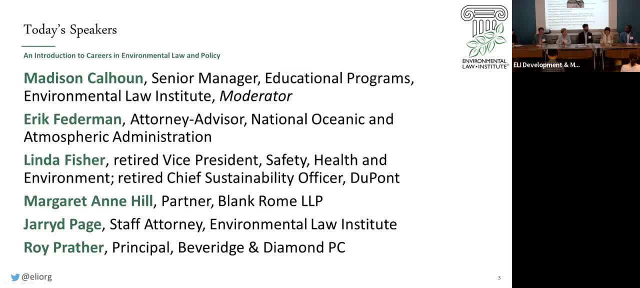 to now finding the anti ESG attitudes. I mean, you know, how did it happen that Republicans in Congress are telling CEOs they don't know how to run the business? They used to tell CEOs: go run your business. Now they're telling them don't go run your business. 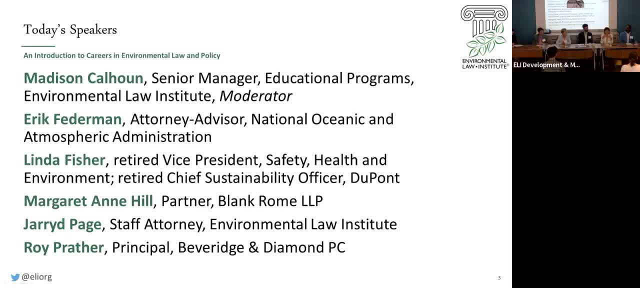 So in any event, I digress. But as a chief sustainability officer, I really had an opportunity at the highest levels in the company to say: these are controversial issues. Where are we going to be on them? Are we going to be part of developing solutions? 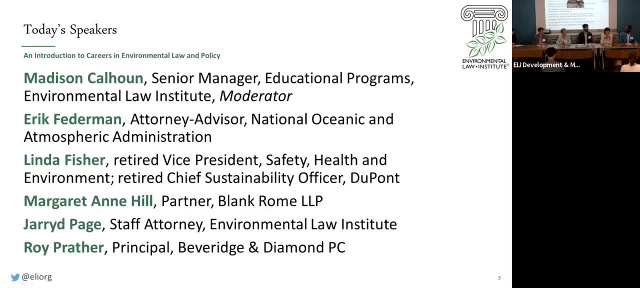 Are we going to be fighting those solutions And my background? more often than not I could push the company in the right direction. So, again, very public policy oriented positions And, as I think everybody here will say, the environmental issues are what makes them interesting. 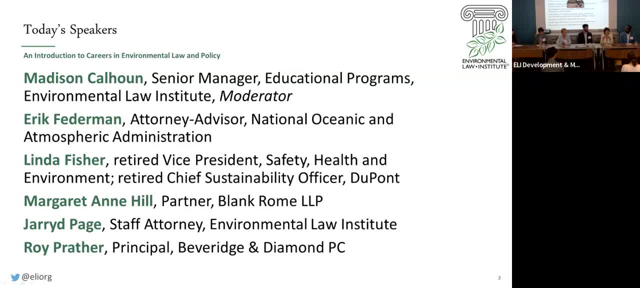 is their complexity and their importance to people, And I found that In both my time at EPA as well as my time in corporate America, And it's kind of the role I serve as an advisor. when I'm on board, I can go maybe the different government perspective. 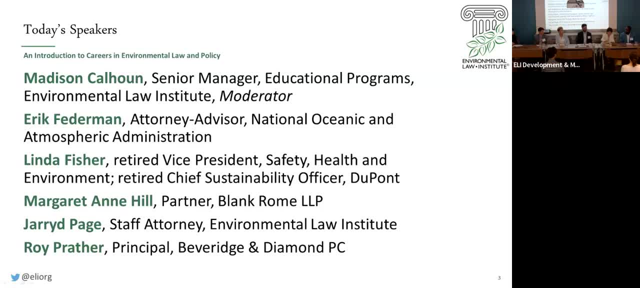 And I'll say, you know, I'm still relatively new in my career, So I don't have the benefit of being able to look back over a long and accomplished stretch of work and talk about, You know, talk with that kind of a perspective. 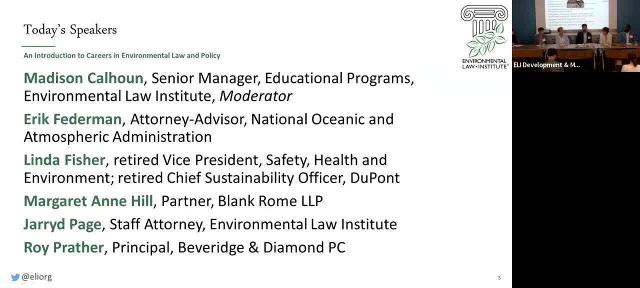 So maybe I'll try to just hone in on what the day-to-day kind of legal tasks that I work on are, And, like others up here, my days are varied. I wouldn't say that there's any kind of typical day or thing that I do. 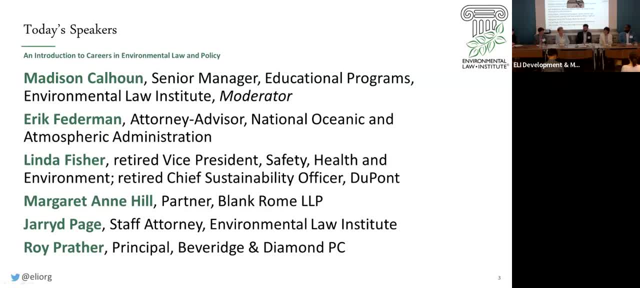 And unfortunately, or fortunately- I don't have to build my time, So I couldn't look back. Oh, fortunately, Fortunately, yeah, I don't live in six-minute increments, So I didn't have the benefit of a timesheet to look back on and see what I'd worked on. 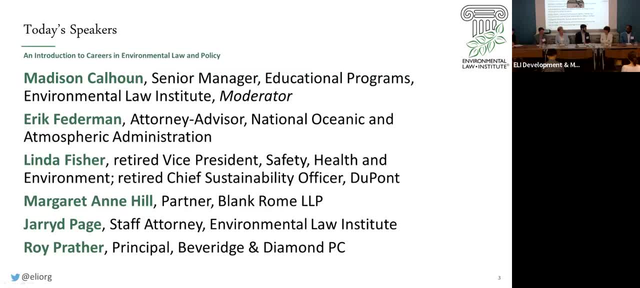 But I would say broadly. you know, the conveyor belt is a nice metaphor. My agency clients have a lot of priorities. There's a lot of things that they want to do. Sure, they come with problems that I have to help them resolve. 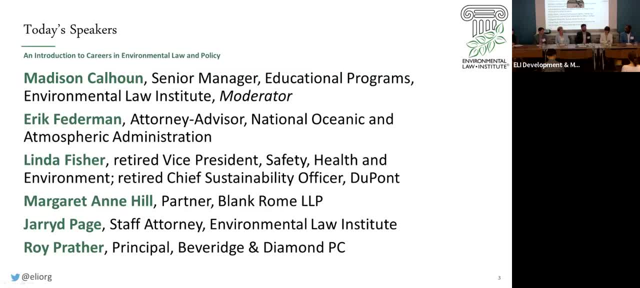 But they also have kind of prospective things that they want to achieve And I think my primary role is to help them achieve those goals, To help keep- I don't know how to work that metaphor in- But to do it in a way that's legally sufficient and complies with all of the web of laws. 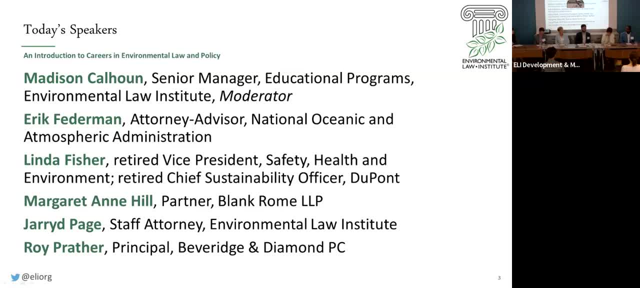 that NOAA, as a federal agency, has to comply with. So you know, on a given day I can work on kind of short, one-off projects If a client wants to enter into a contract or an agreement with somebody else, whether another federal agency or an external party. 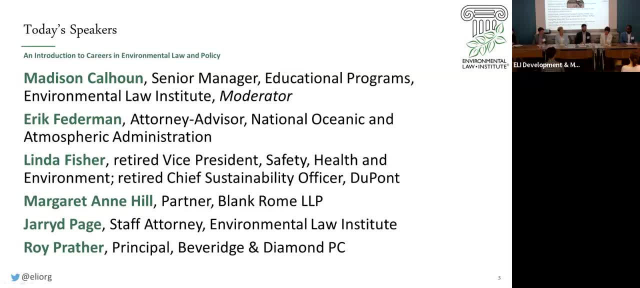 to help achieve their mission. I help draft and review that agreement. If they need to respond to a FOIA request, I get involved and I help you know, identify responsive records, identify potential things to redact, help process the FOIA request. 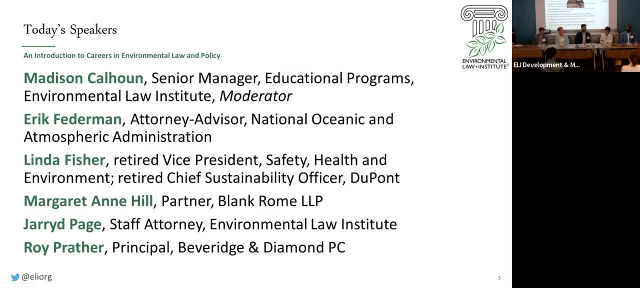 But I also get to work on kind of long-term programmatic projects. I mentioned that I work often with the Office of National Marine Sanctuaries. They're in the process right now of designating six new sanctuaries across the country. 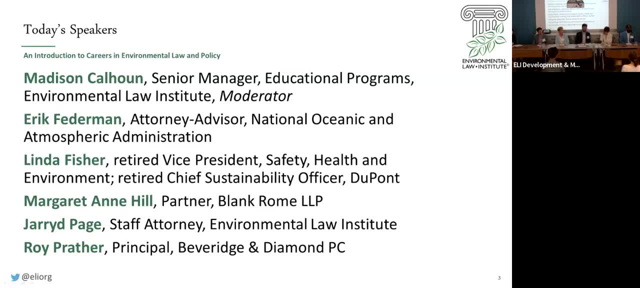 And the lawyers in my office are very involved in those efforts. They're years-long processes And you know we're involved every step of the way, whether that's helping to draft or review the environmental planning documents that are required under NIFA to ensure. 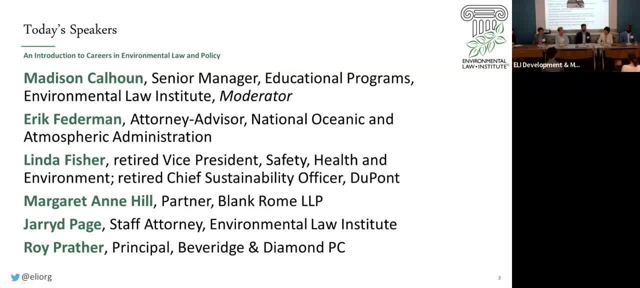 that there's compliance And we're working with the Office of National Marine Sanctuaries to ensure that there's compliance with statutes like the Endangered Species Act and the Marine Mammal Protection Act, which NILA implements but also has to comply with that kind of the rationales in the administrative. 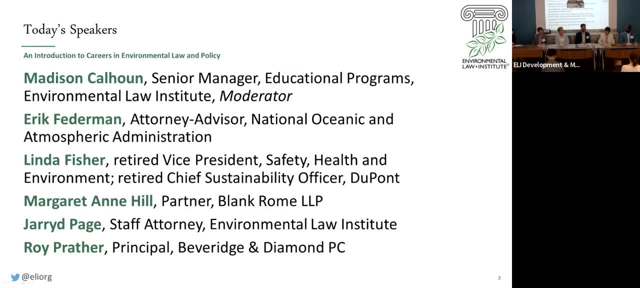 documents and records that we're producing, you know, are strong enough to hold water under the standards of the Administrative Procedure Act, trying to ensure compliance and minimize litigation risk on these kind of long-term projects. Day-to-day that can mean kind of focused review of big documents. 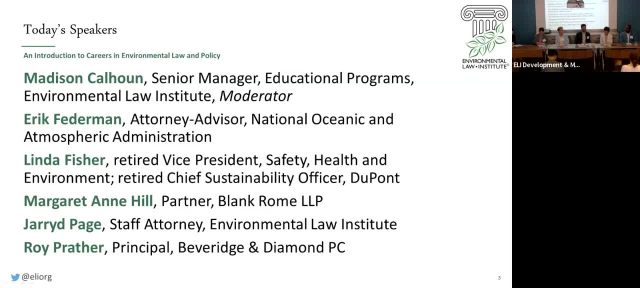 I can spend all day sitting in my office reading an environmental impact statement. I can spend all day on calls with clients fielding questions that they had prepared me for or not prepared me for, and that come up in the moment. I spend time briefing people within my office. 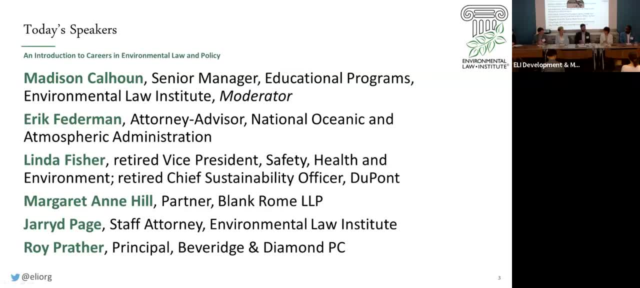 I spend time with the agency, whether on the policy side or kind of on the legal side, to help elevate things, and I spend time helping to represent my agency in either interagency forums or I participated, for example, in a public meeting before the public. 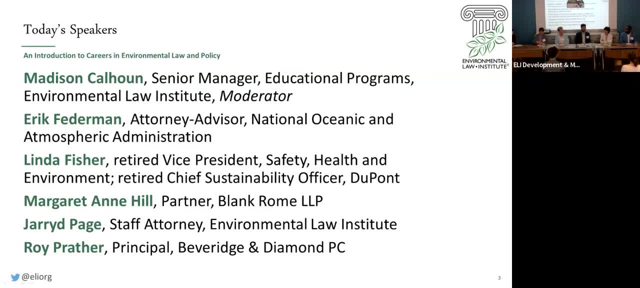 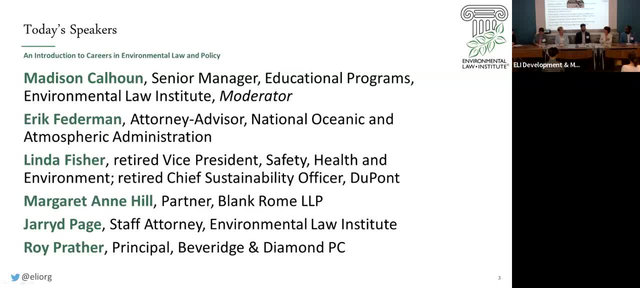 And so I work with programs like Congress to provide input on bills that are, you know, that relate to NOAA's mission and are in committee. So with my clients, I work to provide- we call it- technical drafting assistance to help mark up laws based on our experience implementing them. 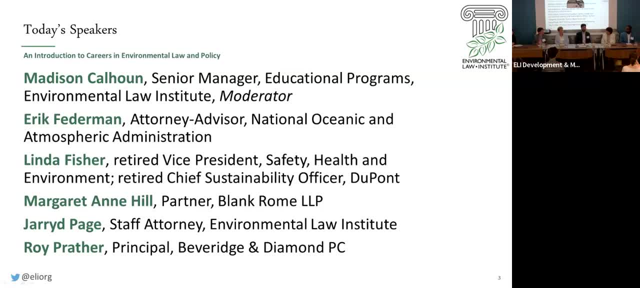 It's really varied work. There's a lot that goes on and every day brings something new repeat, and Peg covered so much in her day I do like maybe half. I don't believe that, But a typical day for me it really does depend on the issues of that particular week, month. 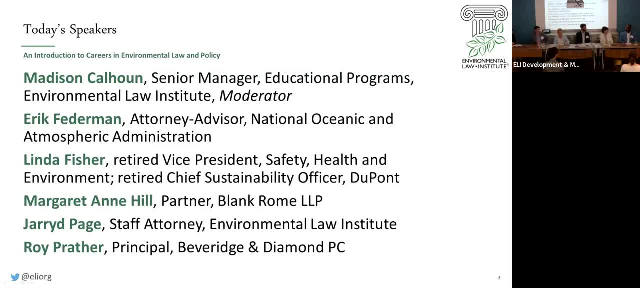 Litigation. you usually have a set schedule that everything needs to happen, so that'll dictate what I'll be focusing my time on. So what I'll do instead is contrast my typical day right now versus when I was more junior at an associate firm, because it was a little bit cleaner back. 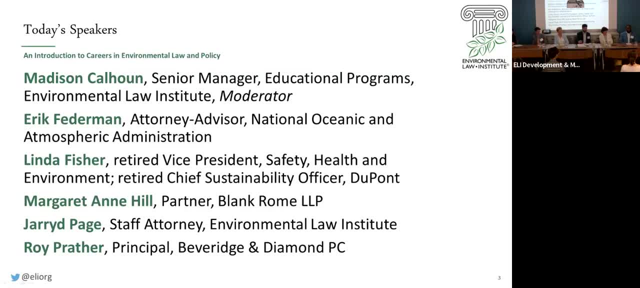 then. Then it was researching, preparing memos or drafting up legal documents for litigation or reviewing documents. It was pretty relatively straightforward. Every now and again appear in court- not frequently- And as I got more senior and was dealing more directly with a lot of the clients that we work, 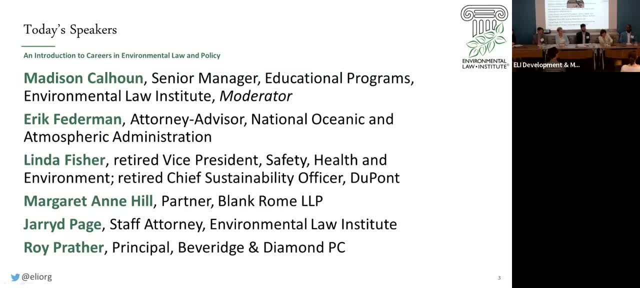 for then it shifted and I spend a lot of my time- really most of my day- in meetings talking through issues advising on strategy related to a project that's being developed and how they're going to approach concerns related to environmental justice issues. 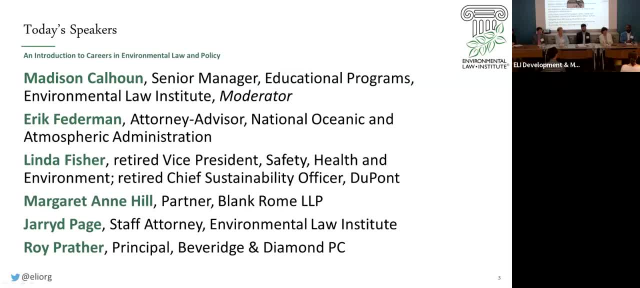 or concerns related to, And then at the same time, jump to another call where we're talking about a property that's being sold and there's been an assessment of the property and what does that mean and does additional investigation needed and what are the implications of doing the additional? 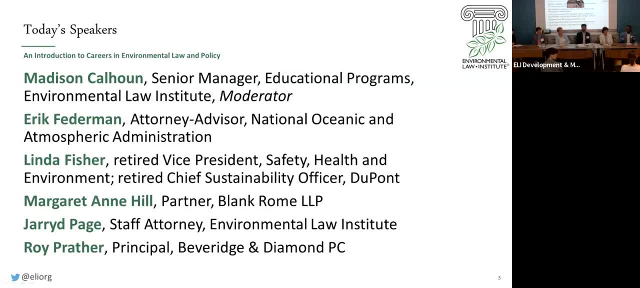 investigation, all of those tricky issues, And then, if there's very hotly contested litigation going on, it could just be in the weeds, drafting motions and responding to briefs, or just talking to the client or opposing counsel and arguing with them about how we should resolve it. 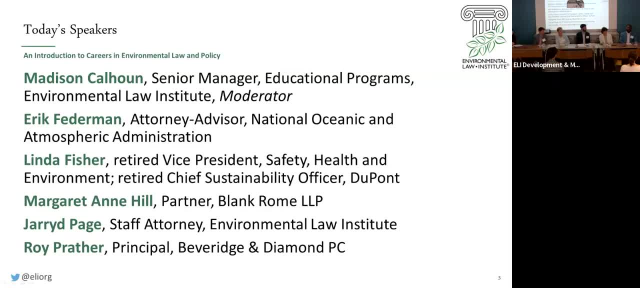 It really does vary. The only thing that's consistent is at the end of the day, I record my time And it's the worst part of the day. No, I'm just kidding, But the variety is again. I said it before: 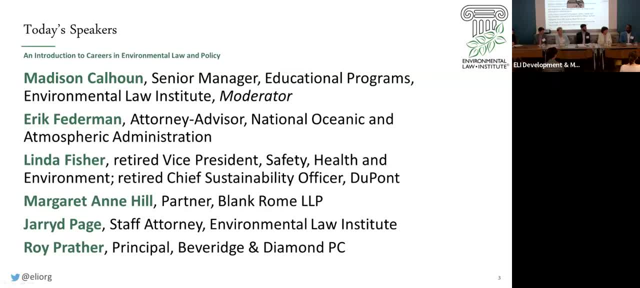 I think the beauty of it. but what you can pretty much guarantee is that you will spend a lot of time reading and you will spend a lot of time writing. So if you are interested in the law, whether you're doing what we do or as a lawyer in general, 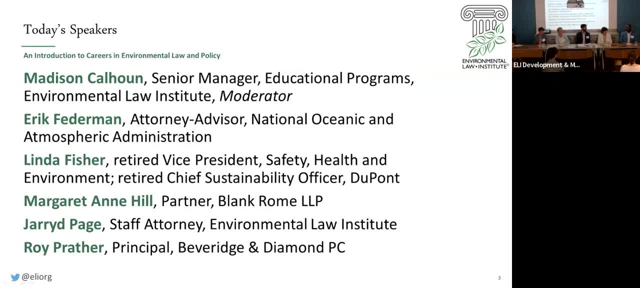 that's going to be the vast majority of time you spend, with certain exceptions. If you are in court every day, kind of working for a prosecutor's office or a public defender, they'll spend maybe four days out of the week just on their feet in court dealing with various things. 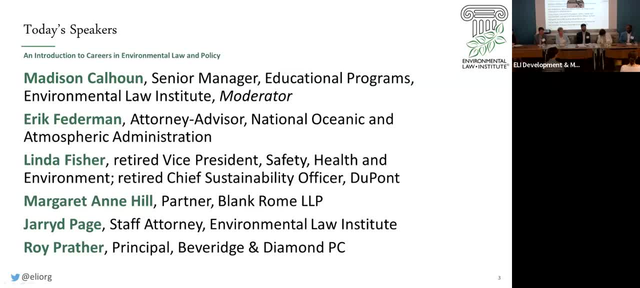 But then they have to go back and do a ton of reading and still do a lot of writing too, So that'll color maybe your view of where your interests might lie. A lot of overlap in my- actually my- typical day with everything that's been said at a research and education institute like DLI. 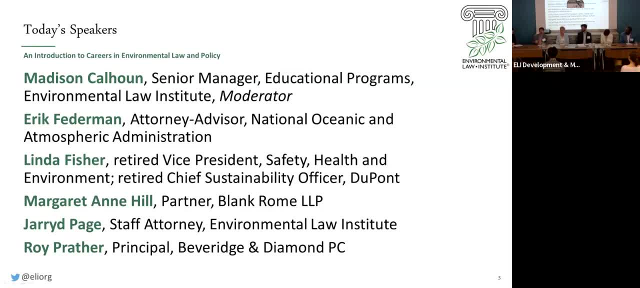 I think, upfront, no, two days are substantively the same, So there is always something that's changing. And the other thing is this is a really fast-moving field- environmental law- And so you're always sort of trying to keep up. 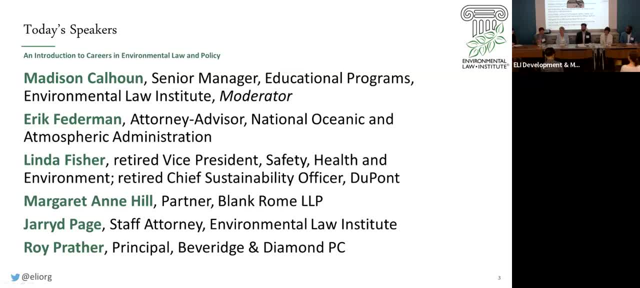 Or you're trying to keep up, Or you're trying to keep up, Or you're trying to keep up Or catch up with what's going on. So, in terms of what I do in a typical day, practically I'm indoors, I'm in my office and I'm at my computer. 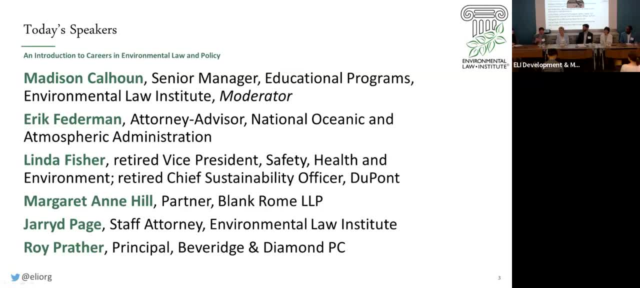 And I'm on my web browser and I'm on my Microsoft Word document almost every day doing something. And what does the research and writing look like here at ELI, For example, this morning I was The research I was doing involved reading court cases. 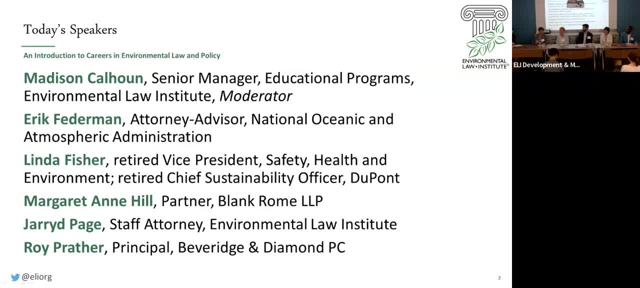 So I was reading a case relating to trespass on public lands in Wyoming. I was reading a case related to A climate case related to climate change. I was reading the sort of proposed changes to NEPA- the NEPA amendments- in the new debt ceiling bill. 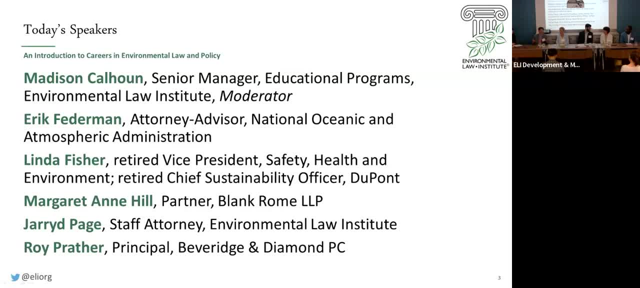 So it can involve a lot of things, And I was also reading news right, Trying to keep current, find out what's going on, see what developments are going on in environmental law. What does the writing look like here? It really ranges. 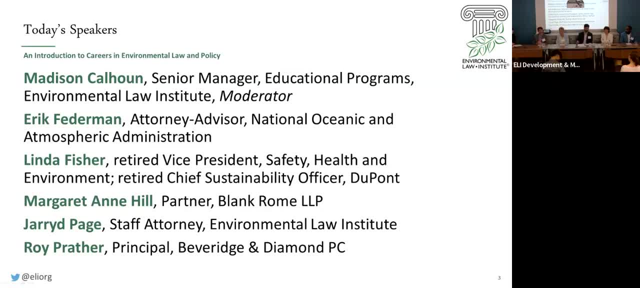 So I was working on. Just a couple days ago I was working on a blog. So we have a blog here at ELI Vibrant Environment, sort of keeping track of what's going on in the fast-moving world of environmental law. 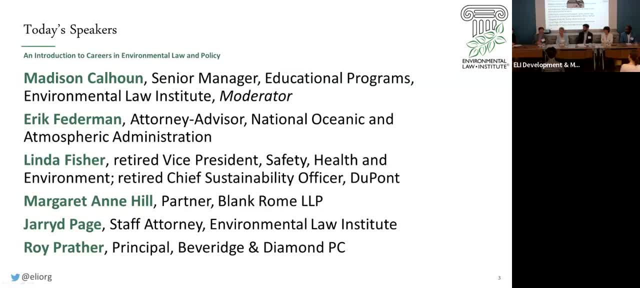 And that was on action that BLM had taken- A proposed rule related to sort of conservation and climate resilience on public lands, And that's for a general audience. I might also be working on a report, for example, on climate litigation for the Climate Judiciary Project that is aimed at state judges. 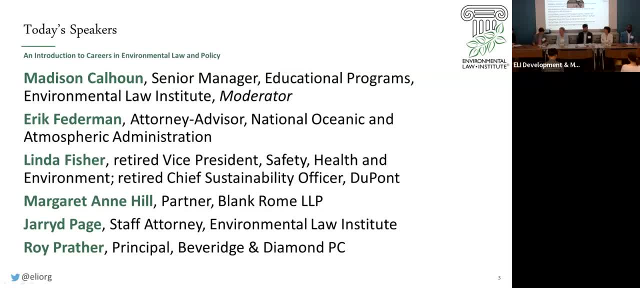 You know, judges in state courts, So writing for a much different audience. So really it really varies. I also spend my time doing presentations And that includes, you know, for internally, for staff, on something like what the NEPA amendments look like. 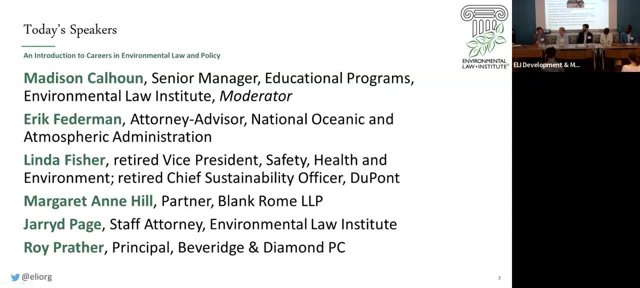 Which I'll be doing this afternoon at one of our meetings, Or engaging with folks like you who are interested in environmental law, Or external partners who want to know about how a particular environmental law is going to affect an issue That they have. One of those things might be compensatory mitigation for the Clean Water Act. 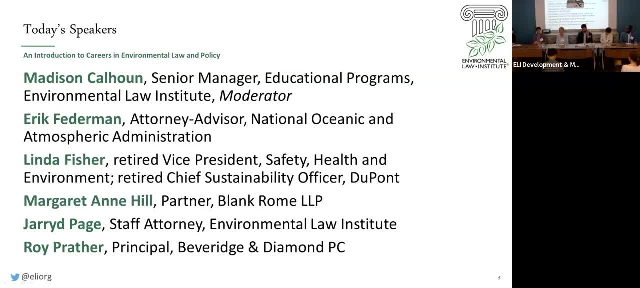 Which I just did a presentation on a couple of weeks ago. So, again, super varied, I think the other thing that you know- I don't think got mentioned, but that I do spend my time doing- is is just thinking. So environmental law is complicated. 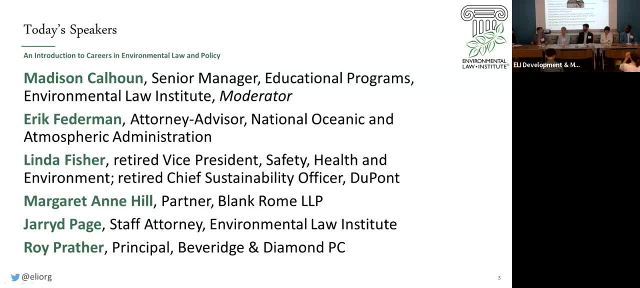 And I think it was you, Eric, who said- the web of laws that are involved in environmental law, And it is really true, And so taking time to think and think creatively is an important part of our jobs as well. Thank you all. 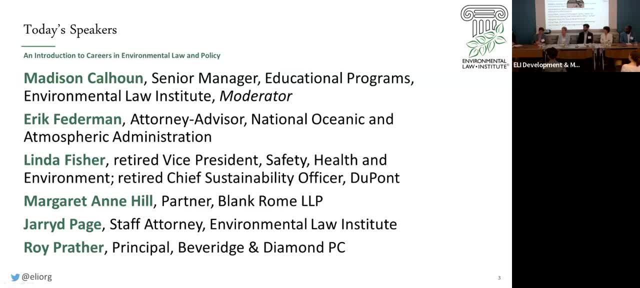 And kind of going off of that. I think a lot of people go to law school thinking that they'll be in court every day, be litigating. So how many of you go to court and how often do you go? I'll just start that one and say I never go to court. 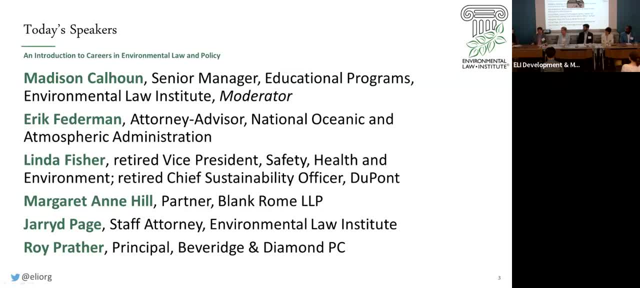 So a couple of the things that ELI doesn't do. We don't do any litigation, We don't have any clients like a typical law firm, And you know we don't go to Capitol Hill and do any lobbying either. So I spent three years at ELI and zero days in a courtroom. 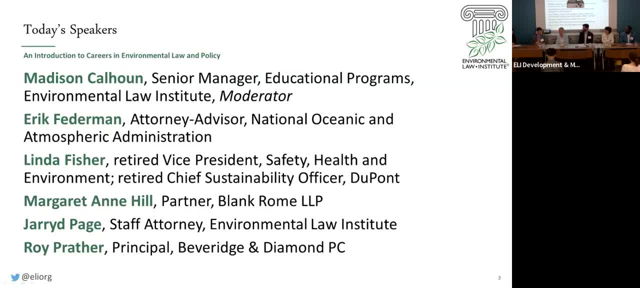 We occasionally get into state and federal court just because there are clients who feel that it's worthwhile pursuing litigation with respect to. Usually, it's a matter involving the cleanup of a contaminated site, because that's where there's a lot of money involved in terms of what's going on. 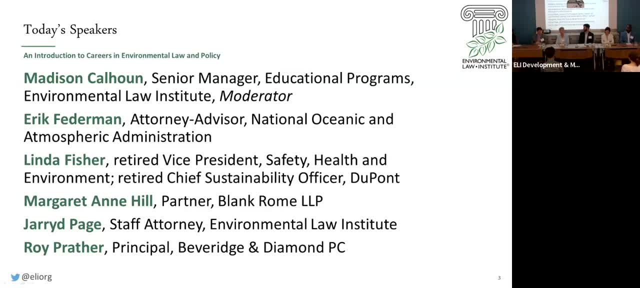 Take to remediate a site. So that's usually where you get involved. Could be a private party action where you know a neighborhood, or some citizens feel that somehow they've been impacted by the operations of a client that you work for, Or it could be the government, or it could be another party that's suing you, that's trying to figure out how to how to winnow down their costs in terms of the allocation what might be needed to remediate a site. 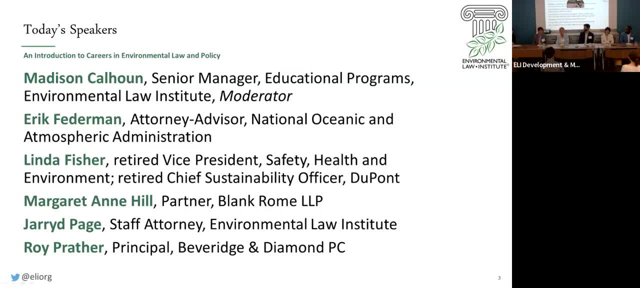 So we do have those kind of cases. The one thing I'll say is that on the enforcement side- the one thing that I've learned and have stuck to throughout playing car practices- You really don't want to argue with the government in terms of like going to court. 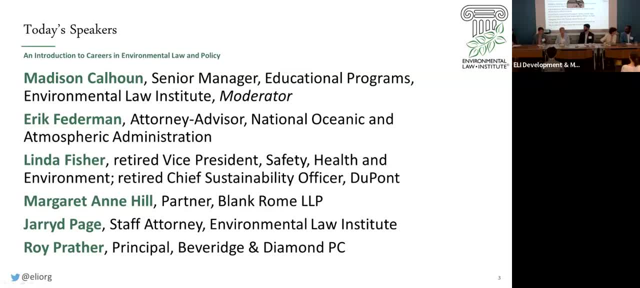 You want to sell your cases, So that's one of the things that we do. We do a lot of enforcement work all across the country And usually those are the cases that you want to sit down with the government. You want to understand. 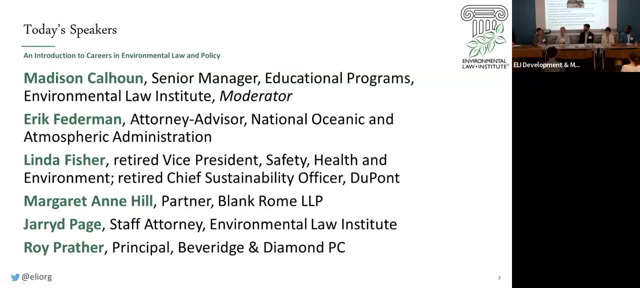 Exactly What they think that you did in terms of violations and how to resolve it. So it's not a court action, but you know it can feel like that, just because you know there's a lot of what we say, discussion and negotiation over interpretation of laws. 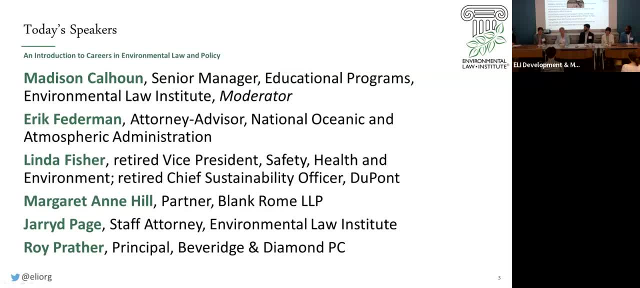 But when it comes to environmental cases, the other thing that I have learned over the years is that typically, trying to present an environmental issue to a jury or to a judge with respect to amazingly complicated laws- Which environmental laws are- Your chances of winning are not high. 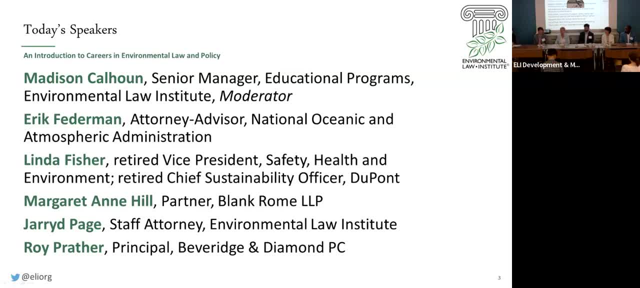 I mean it is up to try to explain, And I'll just give you an example: Years ago, when I wasn't involved, the court action I was at another law firm. We were representing an airline and it had to do with the shipment of hazard materials. 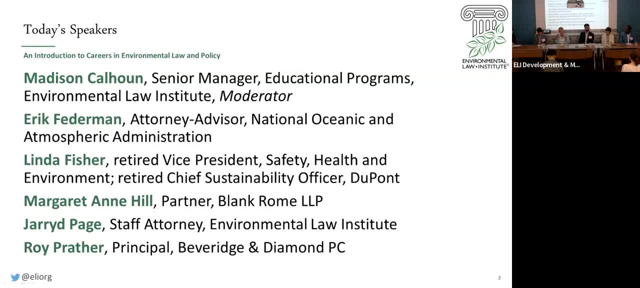 Now, hazard materials- for those of you who don't know, are basically products, Has a struggle, Has a definition under the Hazard Beat in Tr Jur cosine Act and it is which essentially is the Department of Transportation responsibility, But in any event, some hazardous materials. it was a pesticide that went on a plane. 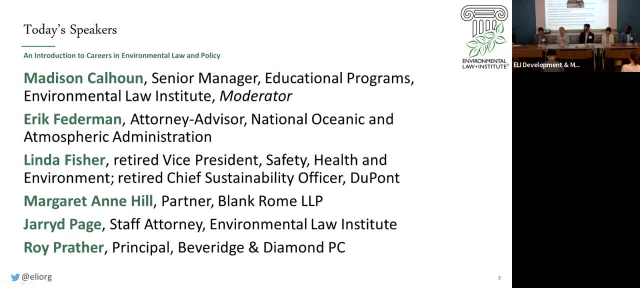 wasn't supposed to be on a passenger aircraft, was supposed to be in a cargo area cargo aircraft. Anyway, somehow somebody tried to get it on a passenger aircraft. It basically fell all over the tarmac and everybody was trying to clean it up. 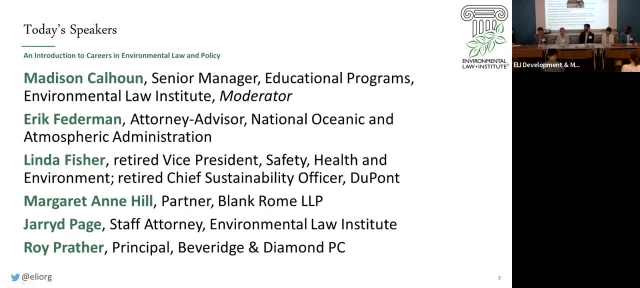 And this company got pursued by the United States Attorney's Office And that was one time, I remember, where the firm I was working with- we decided, like you know what: we need: to try to pursue this in court in terms of defending ourselves, because we didn't really do anything. 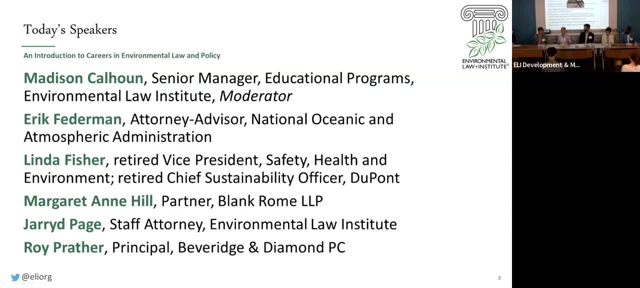 The passenger basically submitted this to the you know the agent ticket agent, and they just put it on the plane. Nobody knew that it was pesticide. So we actually did one of those mock jury trials And I just remember the result was we lost our shirts. 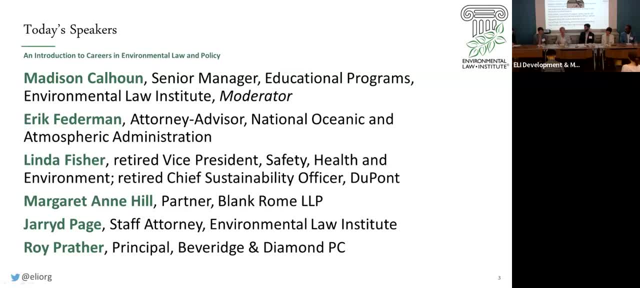 And we just knew we had to try to resolve this with the government in some way. But that's one good example I can give you with respect to environmental cases. And I would say in my younger days if I was a DOJ, of course you do go to court, whether it be trial court or trial court. 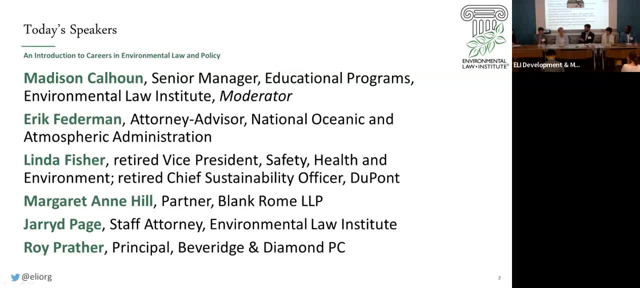 Yeah, I don't go to court. DOJ litigates for me. If my agency clients are sued, DOJ is the, you know, goes actually into court for us, But I do. my office does work closely with the department. I work with the Department of Justice when our agency clients are involved in litigation. 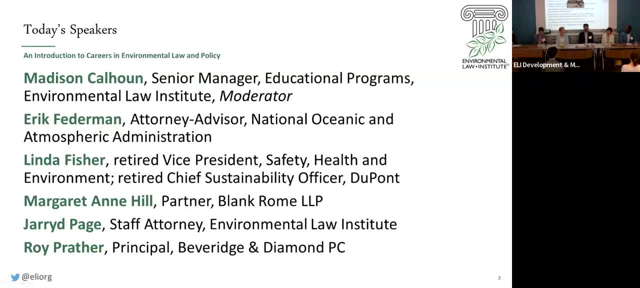 So, even though we don't go into the courtroom ourselves, you know we will review, provide input on and sometimes even draft or assist in the drafting of filings or motions that go to court, Primarily to make sure that our, the statutes that our clients implement, are characterized, you know. 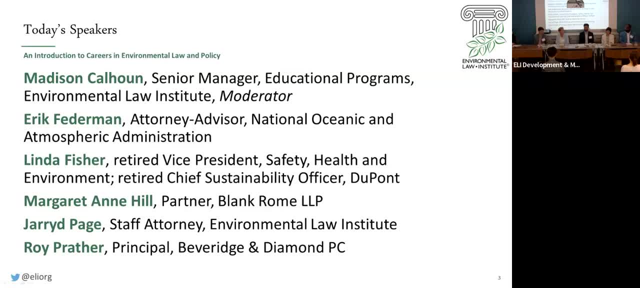 correctly and in a way that aligns with their kind of priorities And goals, because while DOJ is the expert when it comes to motion practice and you know whether to move to dismiss or go to summary judgment or whatever, you know they may not spend a lot of time with especially the more esoteric laws. 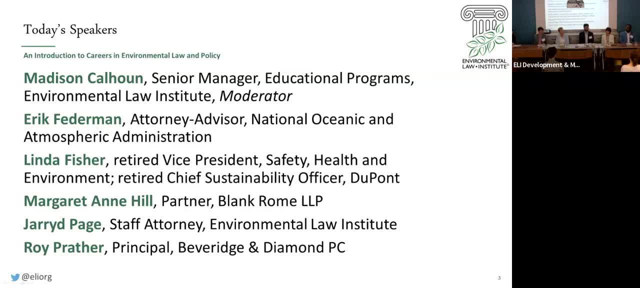 like the Coastal Zones Management Act. So we assist, you know, just in making sure all the filings hold water. Something else that I do, which I didn't expect to do- Yeah, Yeah, I think it's really important to do- is have a role in administrative appeals or proceedings. 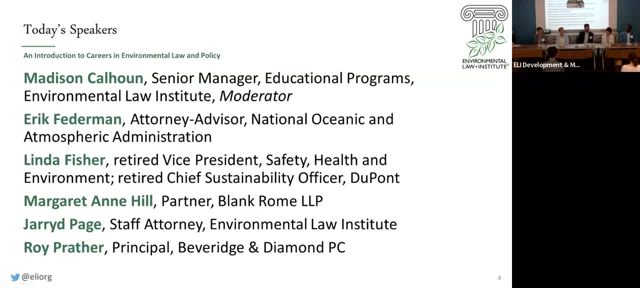 for administrative law judges within the agency. So I kind of always thought of litigation as occurring in courts, with judges and juries or no juries, but kind of like the traditional Article III federal court or a state court. But there are some things that are decided by the, you know. 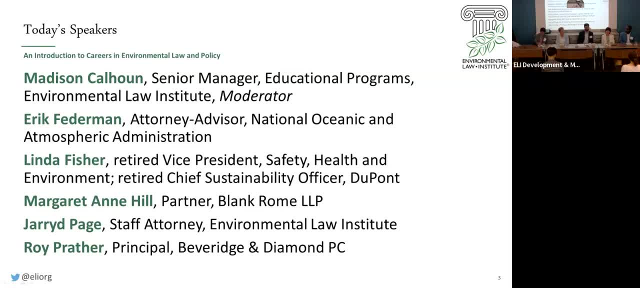 by administrative law judges within agencies, which can then be appealed to. you know the more traditional courts, But, for example, NOAA has an Office of Law Enforcement that has the authority to enforce violations of things like the Magnuson-Stevens Act. 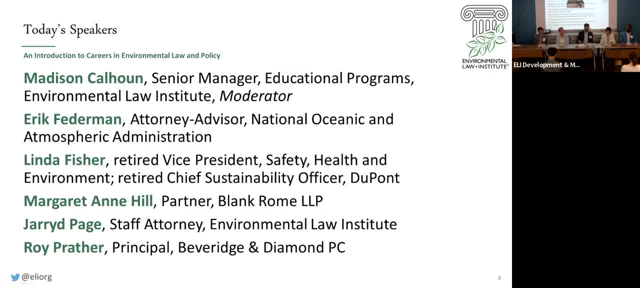 So somebody is fishing in violation of one of the fishery management provisions that's applicable to them. NOAA's office of law enforcement- there's a you know it's you know kind of you know enforcement- can issue them a citation, seek a fine or even bring them into an administrative. 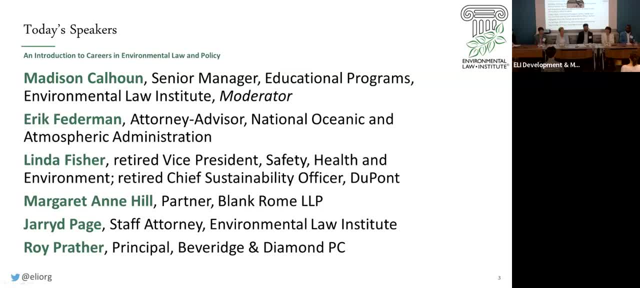 law judge proceeding. so there are attorneys in my office who basically act like prosecutors for the office of law enforcement. i'm not one of those people- that's not the work that i do- but sometimes if those cases are appealed they. they can be appealed either to the NOAA administrator. 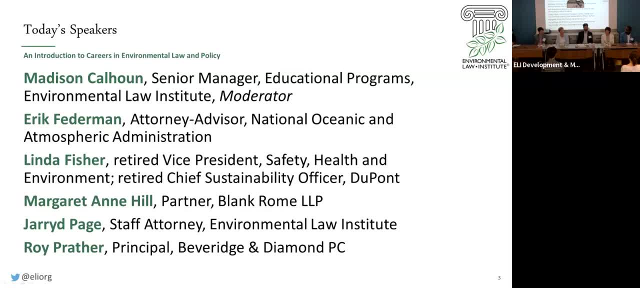 or to somebody like the general counsel of NOAA and my office- and i've done this a couple times- kind of acts as a law clerk for the agency decision maker. so, um, unlike the prosecutor, the defender, we don't kind of make an argument on one side or another, but we 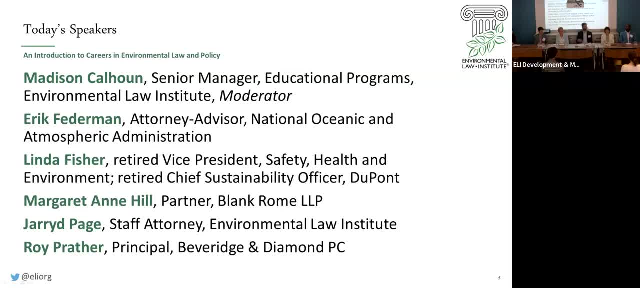 we look at the briefing that the parties have submitted, analyze it um, assess it under the governing law and then make a recommendation to and potentially brief decision maker, whether that's the administrator, um or some deputy um, some really interesting part of my work again that i didn't expect and i don't think fits into kind of the traditional. 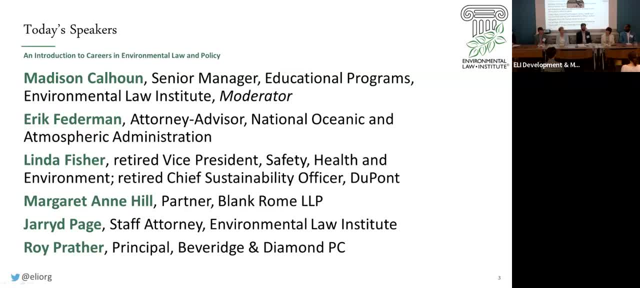 litigation framework that you might think of, um, when you think of lawyering. so the path not taken. uh, when i went to law school, i thought i'd be a litigator and ended up at us environmental protection agency, where i had the opportunity, over the course of my career, to testify in front of. 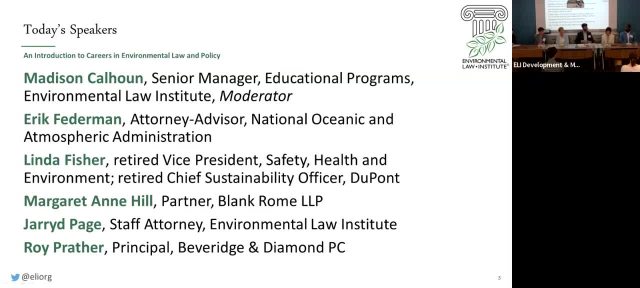 congress probably 40 or 50 times, and at the first one, testifying. when you're from epa and you testify in front of congress, it's quite controversial because the democrats don't think you've done enough and the republicans hate you. and so i stand. you know i go up and i sat there and i thought to myself: so this is. 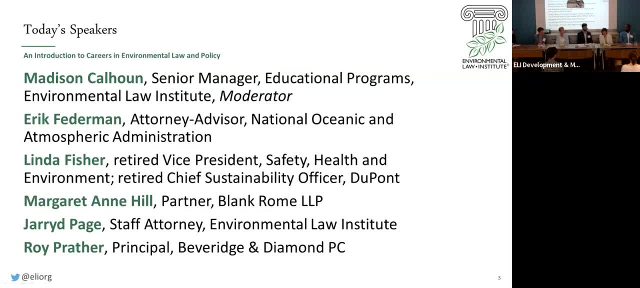 my form of of litigating in in front of a jury, in front of a judge, but it's it's taking a different form. it's a controversial issue in front of congress. so at epa and uh, in corporate america, i was. i was never in court, but i do think those testimonies are about as um close as i could come. 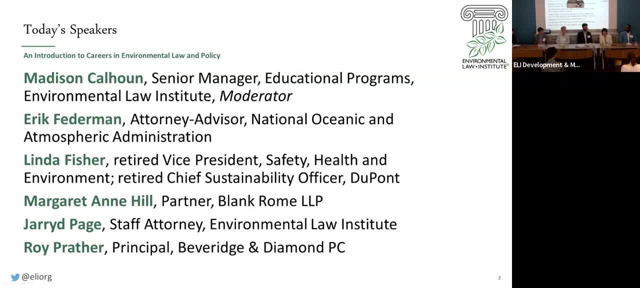 to having the moot court experience within a different branch of government. i might actually suggest that might be a little bit more difficult, honestly, than what i do. so i i go to court a lot, just not physically. so i'm constantly filing things with the court, constantly communicating. 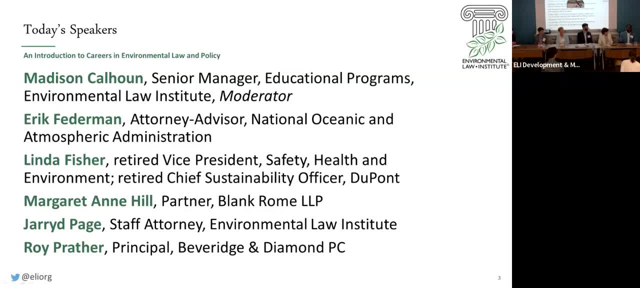 with the court, um, but actually appearing in front of the judge- and these days too, with modern technology and ability to do things remotely, i'm actually physically present in court, much less than, uh, than i used to be really. it comes up for my practice in really one of three contexts. so if litigation where you have 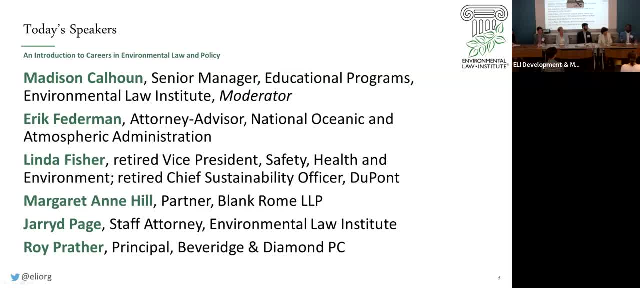 enforcement, which peg has already told you, is always going to be a bad idea to try to kind of fully litigate that um, most, in most instances. so, even if it there is litigation that gets filed, you're working on trying to let's resolve this, because if we have to go in front of a judge or a jury, 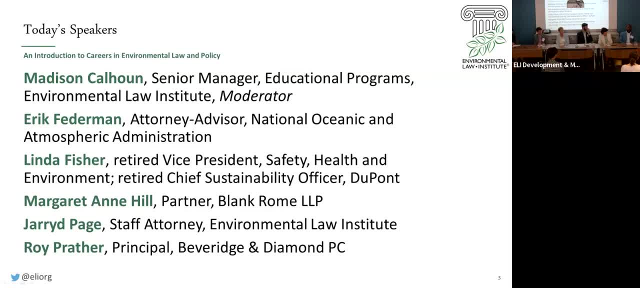 it's probably not going to be great trying to explain it, um, but also in the context of citizens. so you know, clean water act, clean air act, safe drinking water act, you know all those statutes have provisions that allow individual citizens to sue for violations of those laws, particularly 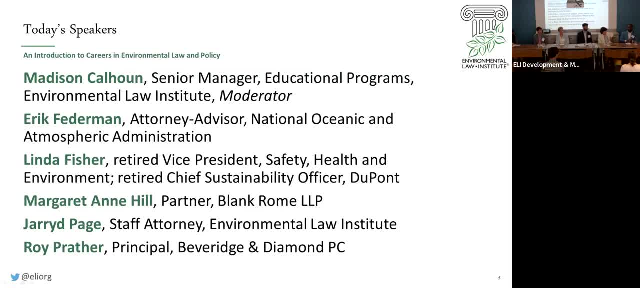 if they believe that the agency responsible is not acting sufficiently right. so um, when that occurs, it's similar to an enforcement action, but it's an individual who's suing, so i will be involved in defending that in terms of showing why they were complying with their permit, or you know what other. 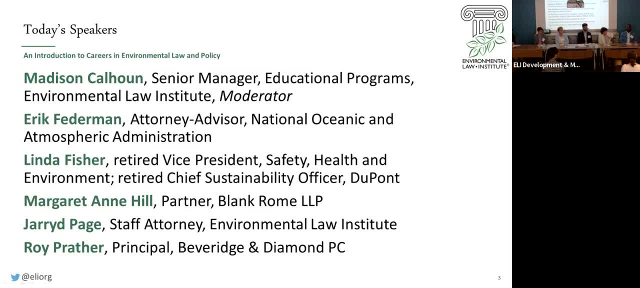 whatever other issue gets addressed and kind of tangentially related to that, there are just tort suits in general where people are essentially alleging some kind of common law claim related to trespass or nuisance or things of that nature, sometimes class action. it just varies depending on the type of issue, and so i think that's something that's important and i think that's something that's. 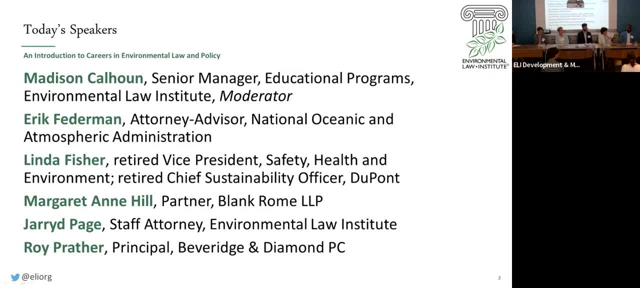 important and i think that's something that's important, and i think that's important, and so we'll be in court um litigating those issues as well. um, and really the last um- so i said three, i guess was four- um the last uh kind of example is um business disputes, right where you could be working. 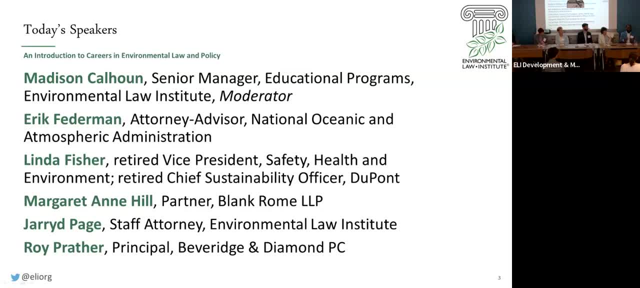 with um, a vendor, and they somehow mishandle something, and so there's an environmental component to whatever went wrong in the contractor. they were installing or constructing something and didn't follow the necessary regulations, or i'm defending someone who was alleged to have not followed the necessary regulations. it really. 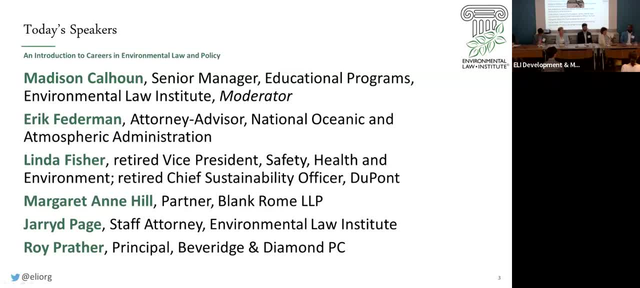 just depends um. but all of those circumstances wind up with me being in state or federal court or in some instances in administrative in front of administrative body. so, um, the variety is nice, but generally speaking i'm still not physically in court, except for very, not unique, but i'd say um. 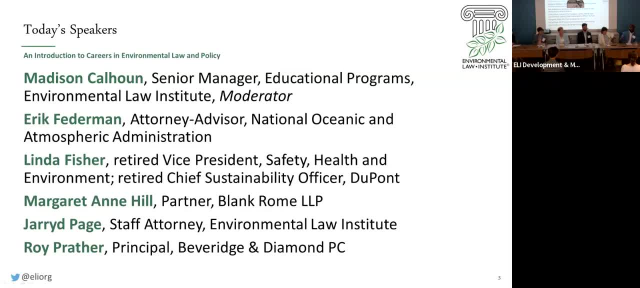 limited circumstances. so if we're, the judge basically wants an argument over a promotion. so you appear to make the argument and i'm just saying that's just one of the differences between a judge and a lawyer and, um, i think that's just the way that law is, you know. i think that if i'm, if i'm doing, 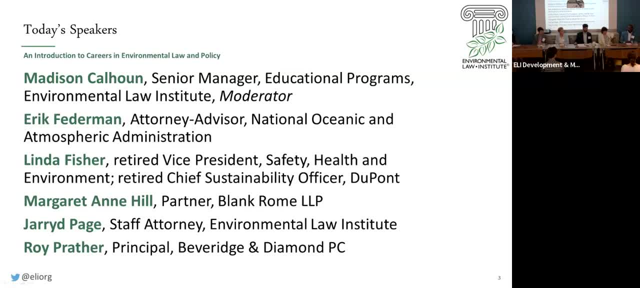 some kind of a trial which in you know the private sector. that's almost always an effort to avoid, if you can, um, because it's so unpredictable how a jury may may decide things, and usually i can't even count the number of times that i've gotten to the day of picking a jury or the day before. 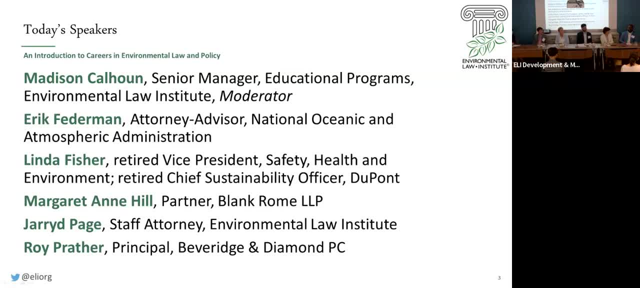 the trial and finally everyone just says, hey, let's not do this, we should, just we should set it and it clients. it was very unpredictable, sometimes successful, sometimes not, and the reasons for it can be things that you would never even anticipate, even though you thought you had this. 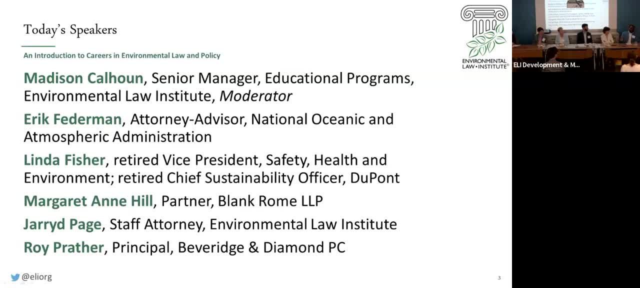 great story to tell and you had these experts that were going to explain all these complicated scientific issues and all those things flew right over their head and the only thing they focused on was that first thing that they heard on like day one of testimony where someone said: well, this: 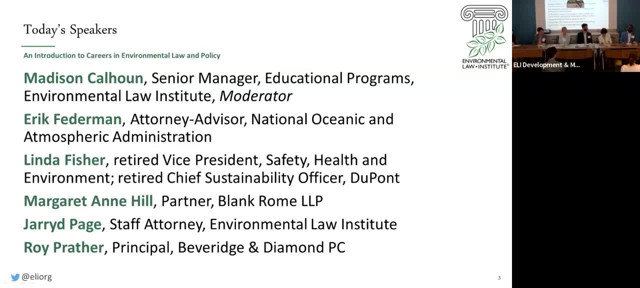 person you know ignored that they were supposed to do x, y and z. on this day it's like, well, that person did that, i won't get into anyway. um, that, that's kind of the extent i should say of the court appearances. another thing that can really vary in environmental law is clients whether you 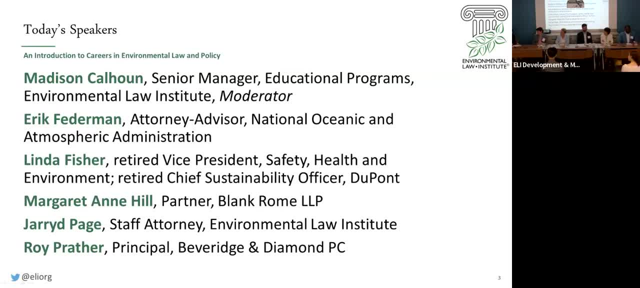 have clients, what type of clients you have, um how much you're doing with them. so how many of you all have clients, and what are ways that you help your client first? um, well, i'll, it's a quick, quick and easy one. yeah, we don't have clients um so. 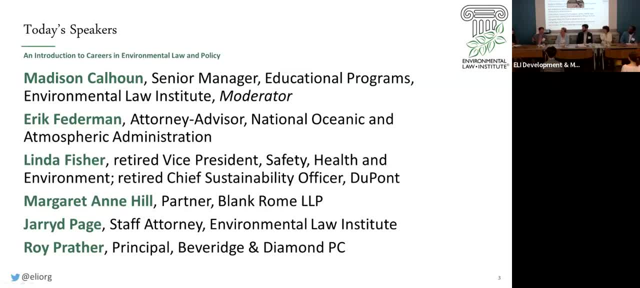 pretty straightforward. i don't worry about trying to help clients, but but i i mean sometimes at eli we talk about sort of the environment being our client, and so you know, we're always sort of trying to do the best, obviously, research that we can for the environment, but we don't have clients. that's a full sense. well, i have a lot of different. 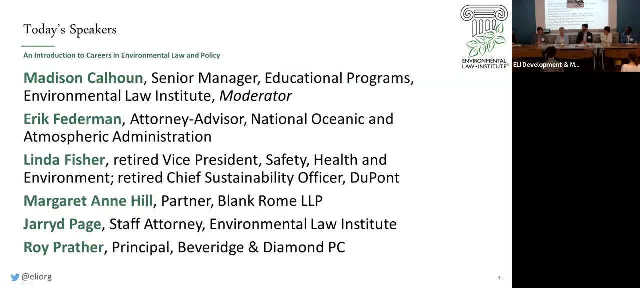 types of clients. i have what you would consider the typical industrial clients- chemical companies, refineries, manufacturers- and i have a lot of different types of clients. i have what you would consider the typical industrial clients- chemical companies, refineries, manufacturers- and i have a lot of different types of clients. 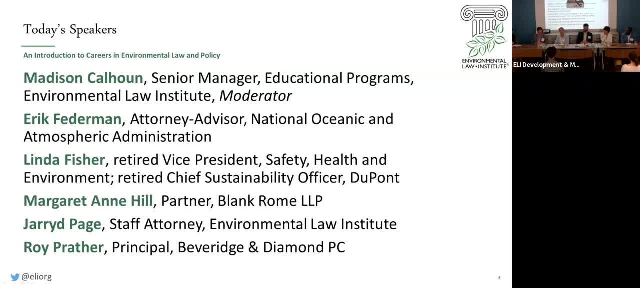 um, both domestic and international. but then we also have clients that are municipalities and counties. we have real estate developers, uh, we have just uh individuals that have issues. uh, you'd be surprised how many just people you know- mom and pops- who have an issue with an above ground tank or an underground storage tank because someone delivering fuel. 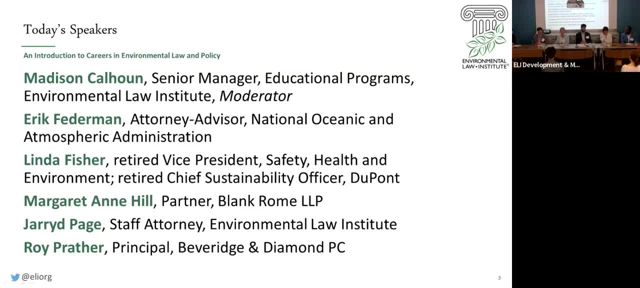 will did something inappropriate. so we have a lot of different types of clients that are. we have a lot of those clients too, um, so the clients really vary, but i would say for the most part, um, they're either companies, uh, or they're either developers or they might be private equity funds. 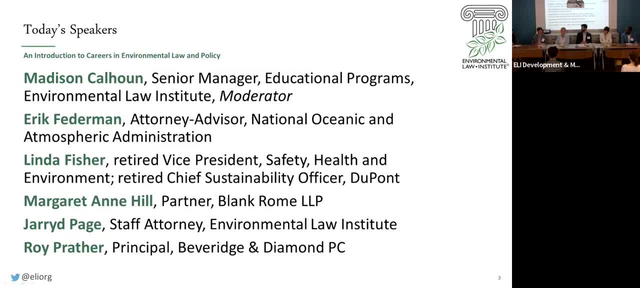 as well, because we do a lot of transactions at our firm um in environmental law, and when you do transactions, typically what you're doing is you're represents- representing someone- either buying or selling an asset, or buying or selling membership shares or stock shares in a company, or buying or selling. 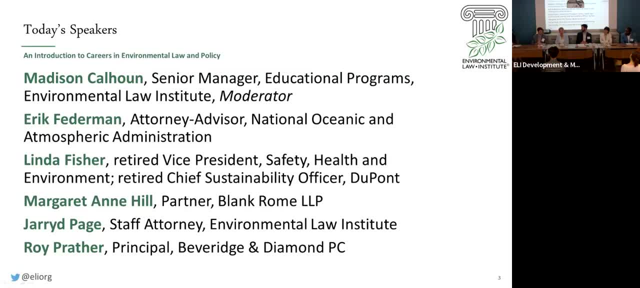 property. so we that that really does vary in terms of who actually comes in the door on those deals, and we also represent a lot of lenders as well. so a lot of the big banks you know in terms of, you know, when they loan money, they want to make sure that whoever they're learning money to is complying. 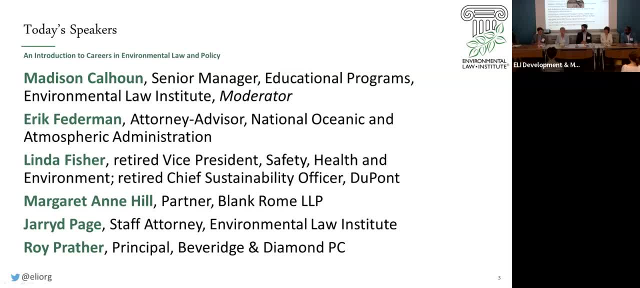 with environmental laws. um, so the credit agreements are written off such that you know there's an obligation to comply with the law. and and one thing that, uh, just going back, wanted to point this out- linda mentioned this and you were mentioning about your former companies that you work with. is that one of the things? 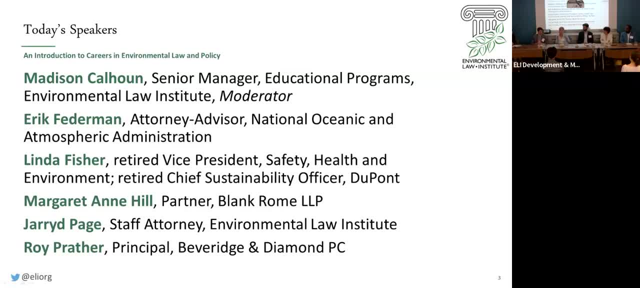 that about industry that you may not be aware of because you know- not trying to politicize anything here, but in terms of where you sit on the fence- um, most of industry that comes to us again with a problem, um, it has to do with trying to understand how to comply with environmental law. so we 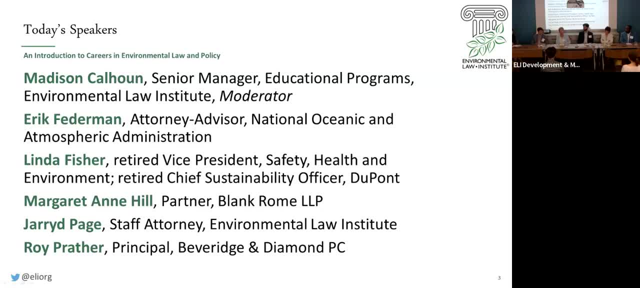 mentioned, for example, compliance counseling, and linda mentioned that you know the clients really try to figure out how are we going to do this, because there's so many things that are happening in the industry, so just imagine a company that's basically looking at a company that I don't know. 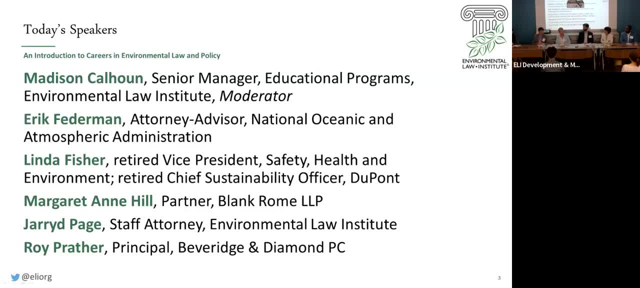 but i don't know what to do with you know they haven't done anything right, they're not doing anything right, and they're not doing anything right. they're not doing anything right. so they're trying to understand. well, I see this is a clean air act. I'm not exactly sure how I'm supposed. 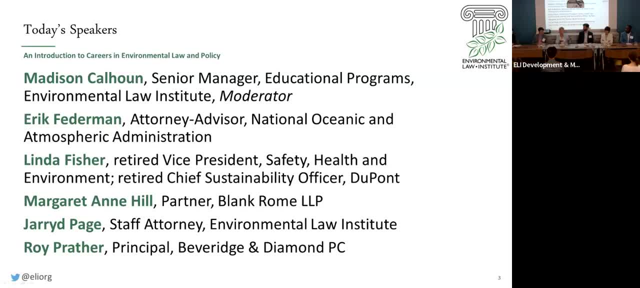 to do this, or I want to modify my permit. what do I need to do? so there's a huge undertaking by a lot of people in a company that come to us or trying to figure out. okay, I'm trying to figure out. There's so many walls out there and regulations. they don't want to miss anything, but they're. 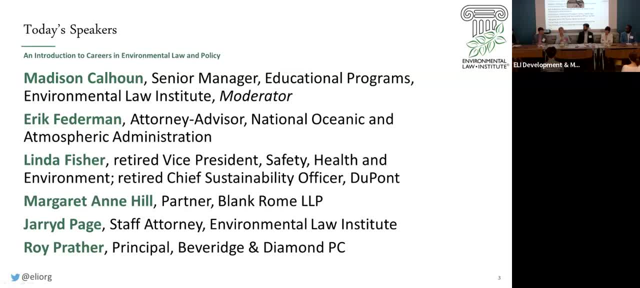 not sure exactly how to include an environmental compliance program to achieve compliance. So a lot of times that's why they're coming to us. I just wanted to emphasize that, that I know sometimes everybody thinks well, industry's bad, but that from my perspective what I'm seeing the most part is somebody going to 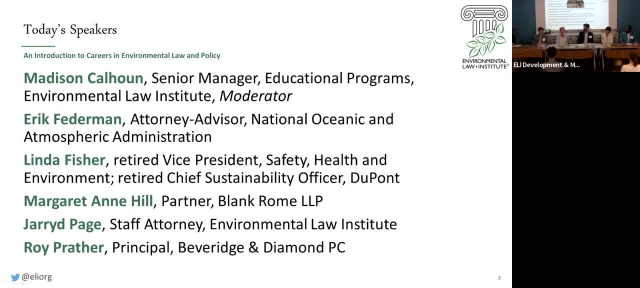 me and saying I don't know how to comply with this. could you tell me exactly what I need to do? Or they might say I need to report something to the government because I have violated the law. How do I go about reporting? sitting down with EPA or state government explaining to. 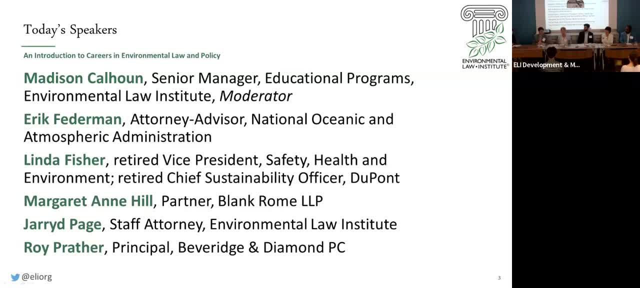 them what happened and then trying to pursue corrective action. So just want to throw that out there. Interesting, I do work with clients every day. My client agency is NOLA, like I've been talking about, and I think maybe something that's. 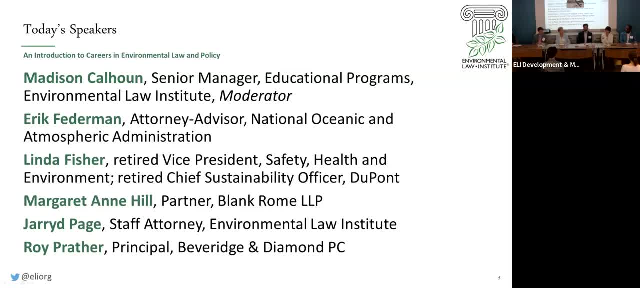 unique. What's unique or interesting about government service, at least compared to the private sector, is that my clients- one- never change, I always have the same client. and two, their legal counsel never changes, so they can't hire me. 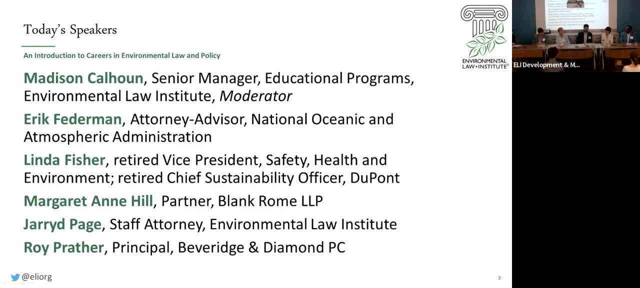 And I would say kind of. I talked about my day to day, I think a little bit in the last part, but at a big picture level, everything that I do is client driven. Everything that I do is in response to something that my clients want to do. 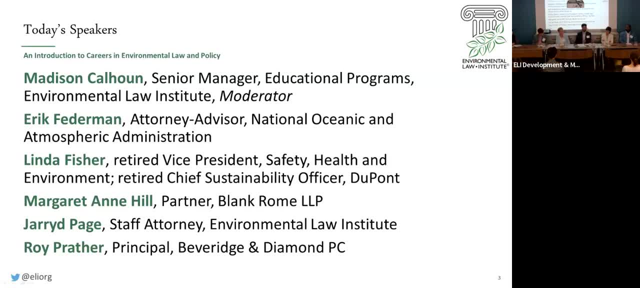 And, like I said before, you know, I think my job is to help them implement the things that they want to do in a legally sufficient way, So that, you know, includes compliance, maybe in a different way than in the private sector. 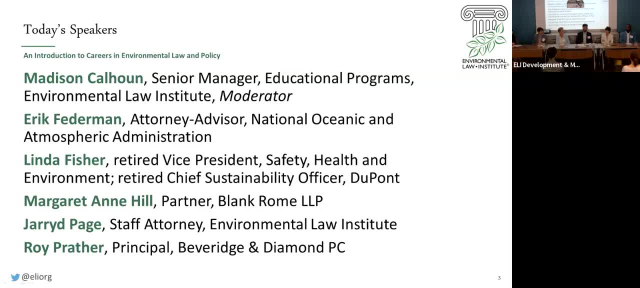 but making sure that they comply with all the federal laws that they have to comply with as they do things, helping minimize their litigation risk as they do things And helping them interpret their own authority. So not only the things that they have to comply with, but also like what is it that they're? 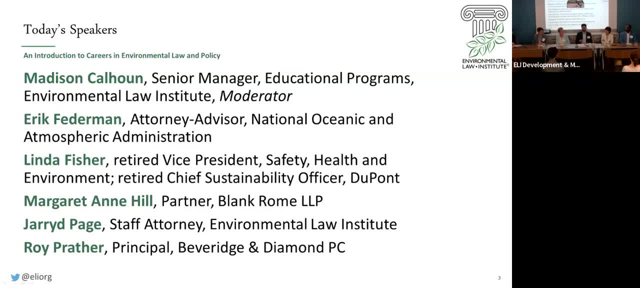 able to do? How far does the law go? How broad is their authority under a given statutory provision? So I work really closely with my clients and it's something I really enjoy. So I only practiced for two years But I think, following on Peg's point, a lot of it is problem solved. 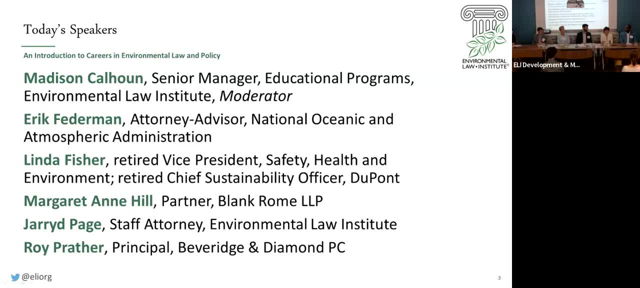 Easy stuff Companies can do themselves. They've got a lot of very good engineers, unless they're small and then they need outside counsel to help them. But it's also: how do I solve kind of unique problems? Clean Air Act is going to make me put very expensive control devices on four of my facilities. 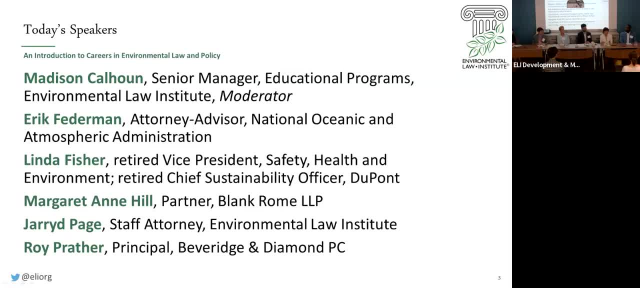 but one of them I'm going to close down in three or four years. So do I really have to invest? Yeah, Is there a way we can negotiate some other? can I put more restrictive controls on the three plants we're going to keep operational and let the other one go? 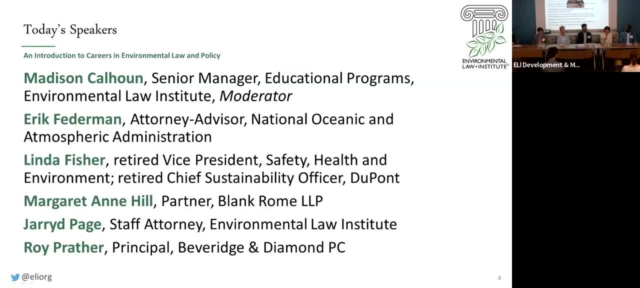 What's creative problem solving that we can be a part of with the agencies And inside the companies I was with. you can have a well-run, very strong compliance program and things can go wrong. People can make bad decisions Checking the bag with the pesticide at the passenger right. 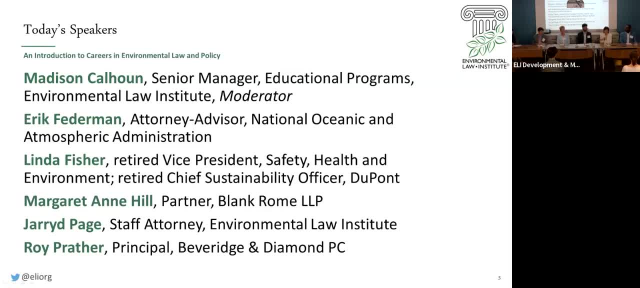 Or things happen, And how do you go in and fix it as quickly, as I want to say, as cost effectively as possible? Because, again, most companies- I hate to generalize with everybody- most companies are in business to do something and compliance is a part of that. 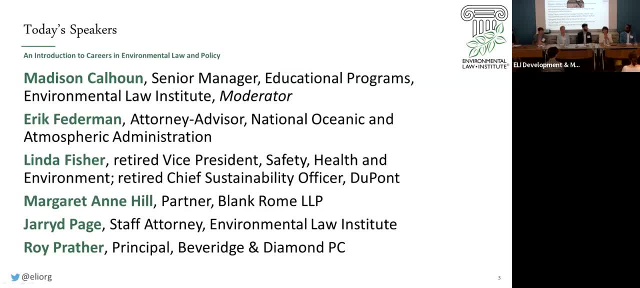 So if something goes wrong, they actually do want to fix it. Fix it quickly, Keep their reputation and brand out of the headlines. And as counsel, either inside or in private practice, you're really looking for people who can give you advice on how to get past this mountain so you can get on doing what? 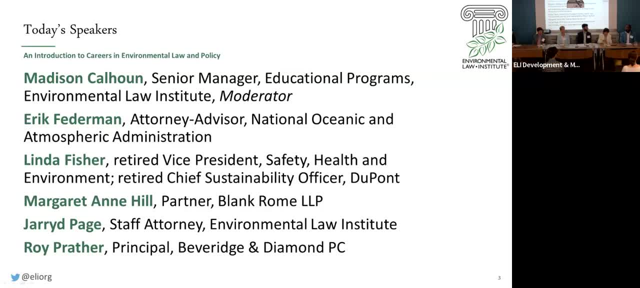 you really want to do So. I think Peg can entirely cover almost every single client that we work with. So what I'll add, because I don't want to repeat- In addition to the initial problem solving, where someone has a problem and they come, 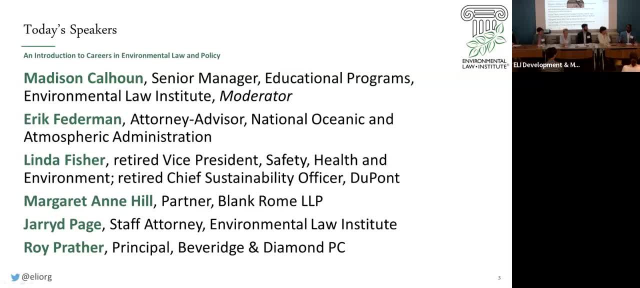 to you a lot of times. what we do now is anticipate right What direction. I think Jerry mentioned before how this is a very dynamic area. There's always some new regulation. The science is always improving. Now they can detect the contaminant at this level. 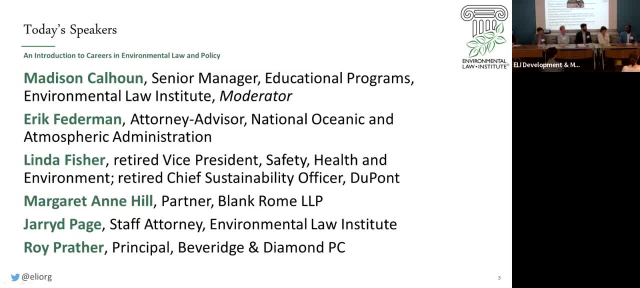 And what does that mean for application of whatever particular law you're looking at? And so can you basically let it go? Yeah, You can let a client know. look, this may be coming down the pipe. You want to consider how this will impact your operations. 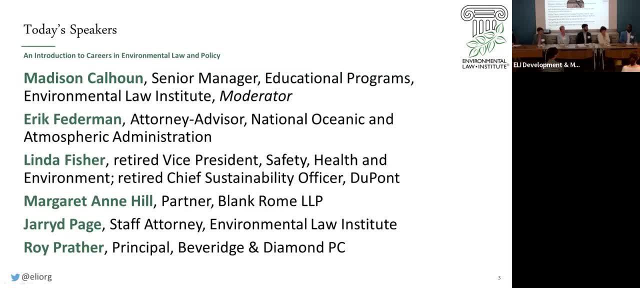 Here are some initial thoughts of how that might work, And then sometimes they're way ahead of you. I guess we thought about this and we're doing X, Y and Z Or other times. they're like: oh, we need to sit down and figure out how we're going to. 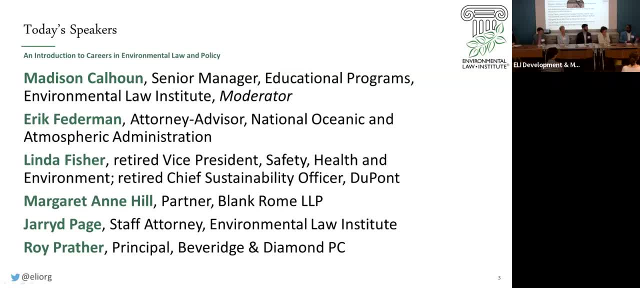 handle this? Or the administration is changing and there may be different priorities, And are we shored up in the right areas to make sure that our compliance program is still going to consistently be applied in a way that's not going to get any crosshairs right? 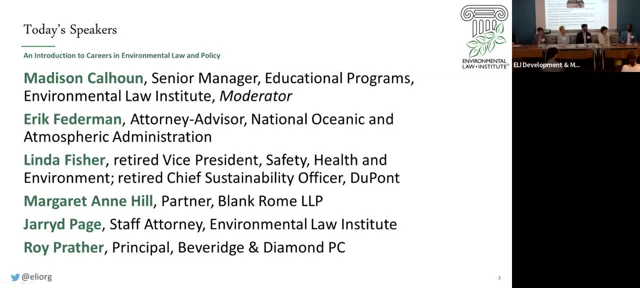 The other client base that I'll highlight- and Peg mentioned them- is the municipalities. They're a little bit- and I'd probably add utilities into that equation too- but they're a little bit unique to some of the industry clients that we work with, in the sense that 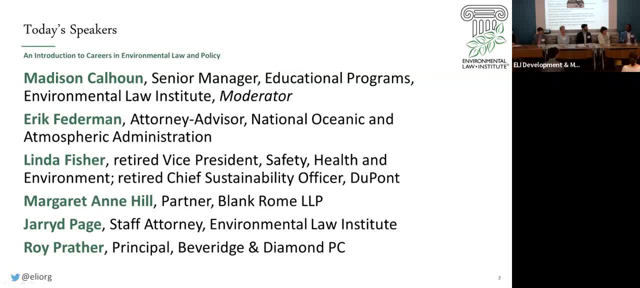 many of the industry clients. they have products or services that they're putting together and they're offering to the public, Whereas with municipalities, a lot of times what you're dealing with is government organizations, government bodies that are kind of charged with providing for the citizens that live. 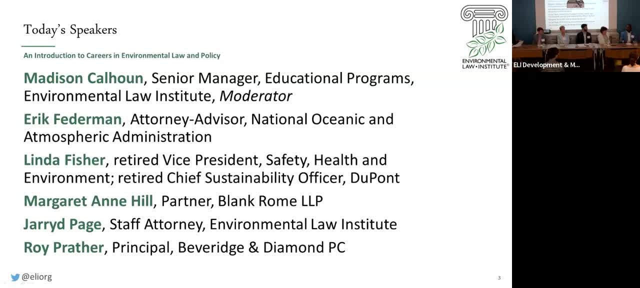 within that area of essential functions- drinking water, for instance. And so you end up with all of these clients having to think about, just beyond what the law says and what the regulations require, the impacts of all of those interpretations of the law, all of the implementations of the law, and the consequences of that can. 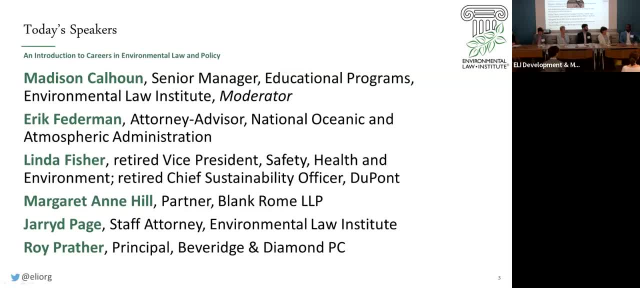 vary pretty widely, But you always have to be thinking about what is unique about this particular client that I should be thinking about, I should be thinking about, I should be thinking about, I should be factoring into, because it's not enough to just say here's what the Clean. 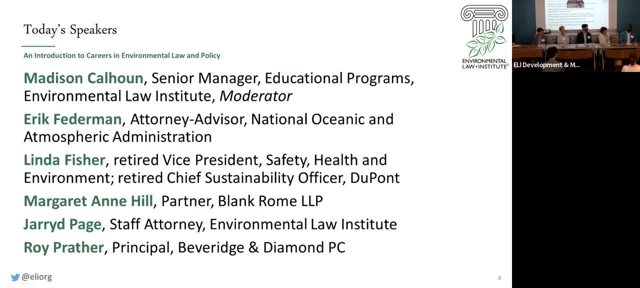 Water Act says. here's what the regulations say and here's what that case says. but we have to go through this process of talking with them about. here's what that means for you and for those that you serve or those that you work with. 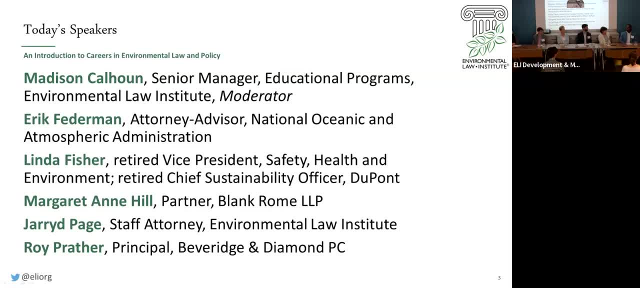 And so that's the nice part of having such a broad base of clients, honestly, But I think with any client relationship that's kind of what is entailed in that process. We'll go to audience questions in a few minutes here, but with our last couple of questions, 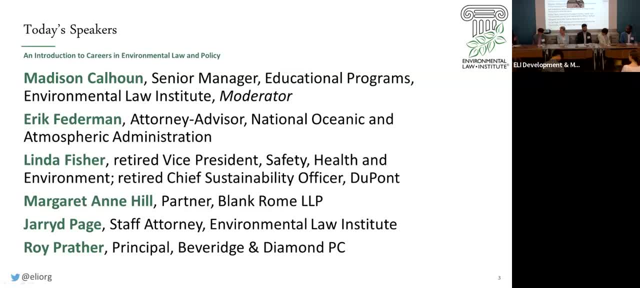 that we've prepared. I wanted to touch on some more advice-related questions. So most of our audience today, as I said earlier, is students and young professionals who are just starting their career journeys in environmental law or even just considering a career in environmental. 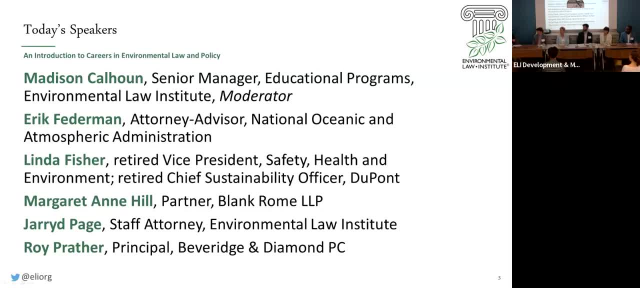 law. So what's one thing that you wish you had known about environmental law when you were just starting to practice? How friendly everyone is and how approachable they are, and how willing people are to help you if you have a question Or you. 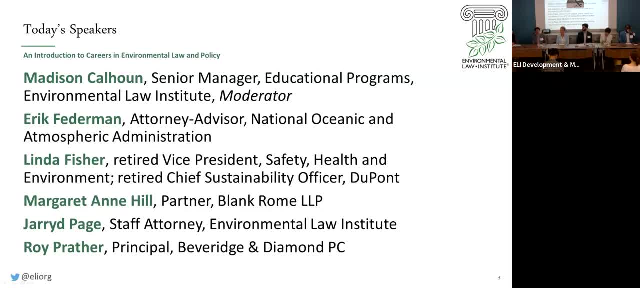 If you want advice. you know, I think there's sort of an intimidation factor when you're trying to break into a new field or you're trying to sort of find out if you're interested in something. And really I think to a person, everyone that I've approached, you know, in the past- 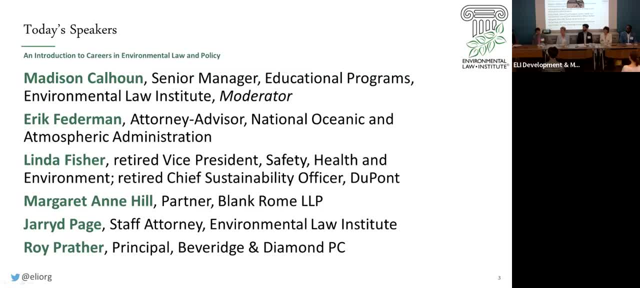 several years about some question of environmental law, career-related question- have absolutely been supportive and willing to talk And give advice and share their perspective And so you know, just knowing that early on I think would have been even more helpful. 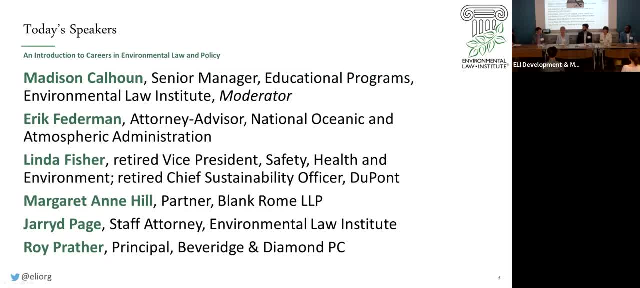 to me. So, yeah, I wish I had taken several science courses- I didn't- And environmental law. there's a lot of technology involved in practicing environmental law And we've all been talking about it, So I didn't take really many science courses in college. 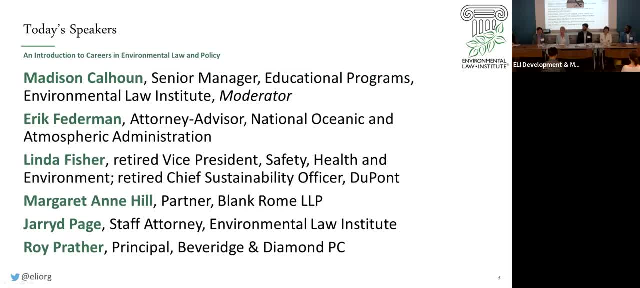 Or undergraduate And I'm basically learning on the job. I mean now there's a lot of things that I know, But again, if I could go back in time, I would have taken many more science courses, And that's one thing that I really regret that I did not do. 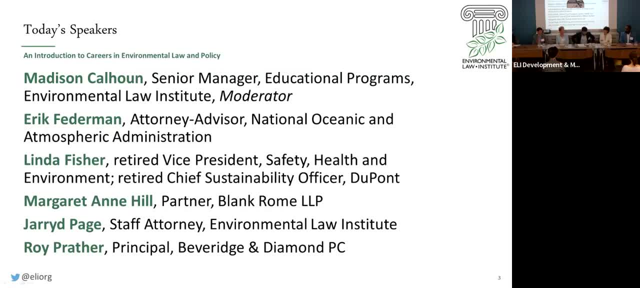 It's funny to hear that, Because what I was going to say is: you know, I had a big chip on my shoulder coming into this field, not having a science background, And it's something that really made me nervous, preoccupied me. 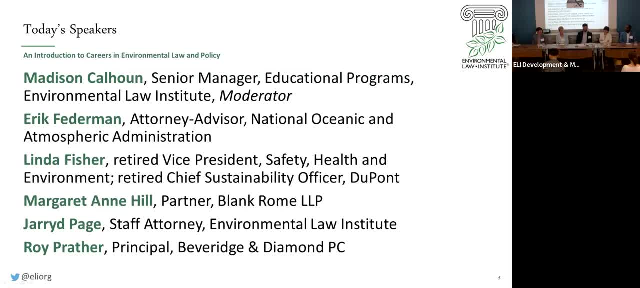 As I was going into the job market, But I have been relieved to find that I don't think it's a big impediment Or has been a big impediment to me as I've been starting my career. There are certainly things that I don't understand. 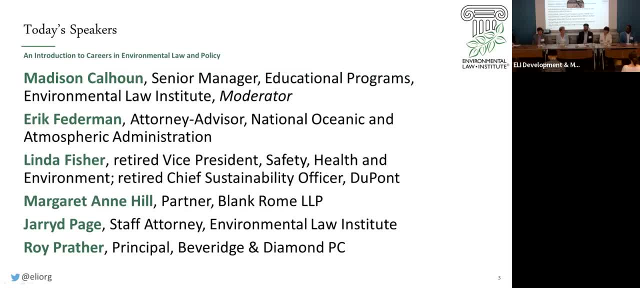 And maybe it would have been helpful to have taken some biology in college. But I think Roy said towards the beginning: you know, I think part of the job is translating the science for the public, Or I'm not before judges very often, Or ever. 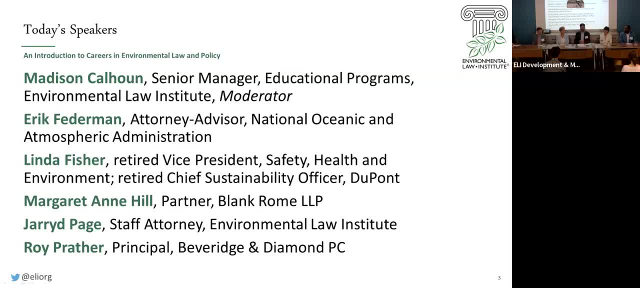 But, you know, trying to take the work that the scientists are doing and make it something that's, you know, intelligible to the broader public, And I think I'm able to fill that role, just you know, with like a willingness to learn. 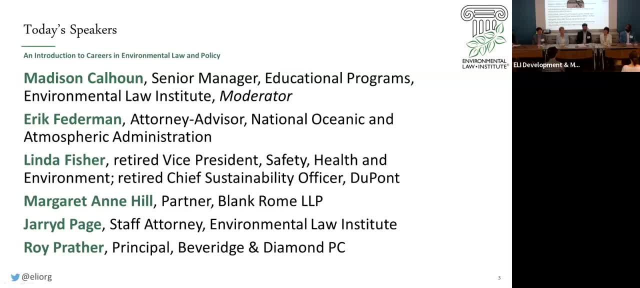 And I, like I said, I don't think it's really held me back to not have had a science background. I have two things That I wish I'd known. maybe Number one is: nothing in the environmental area is quite as black or white as people. 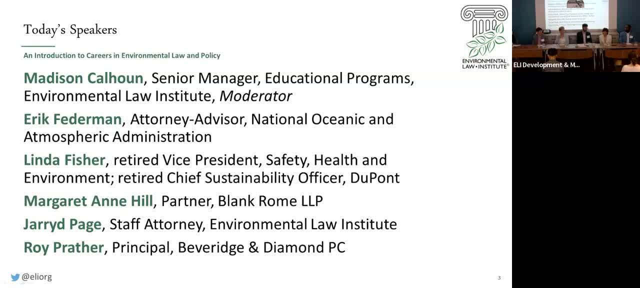 want to make it to be. The laws are complex, The issues are complex. The science does not give you an answer. Science leads you in a direction, It takes you close, But there's a reason why scientists shouldn't really make all the decisions, because there's 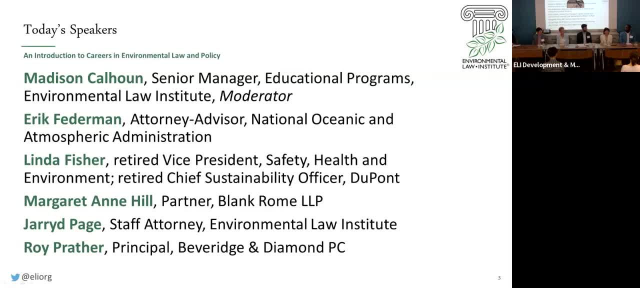 so many other things that influence. And that gets to my second point. The law only gets you so far. As I said earlier, environmental laws affect every business, every city, every town, every person, And if you're a company or an environmental group or a municipality, you've got to be 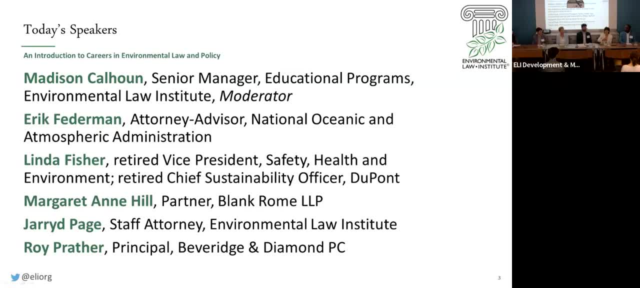 in compliance on the right side of the law, but it doesn't necessarily guarantee you what I call the freedom to operate. You've really got to understand that. You've got to understand that. You've got to understand that. You've got to understand where the community's coming from. the people are coming from, the 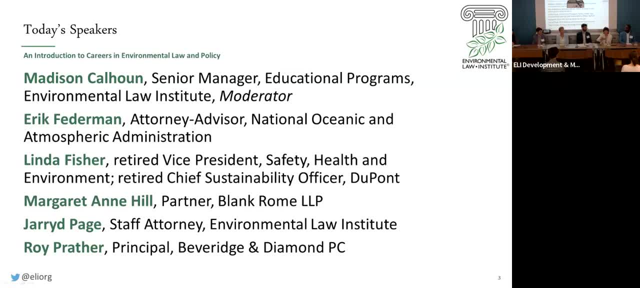 diversity of wherever you're operating, in many cases kind of the larger political arena that you're playing in, And so you really, as a lawyer- I think the best lawyers- understand the law. They understand, I'll say, the guardrails where the law takes you. 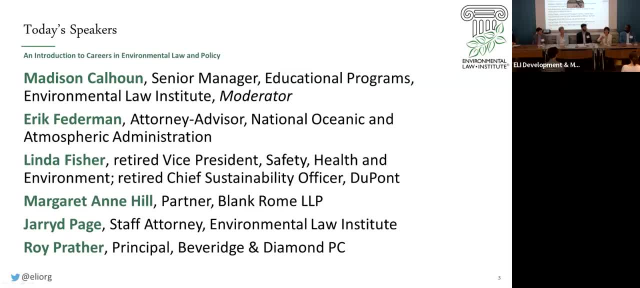 But I don't think I appreciated how much all the other influences We're going to either open doors or close doors for either my clients or when I was at EPA or when I was at the company, And I think the ability to understand those other forces or those other influencers is 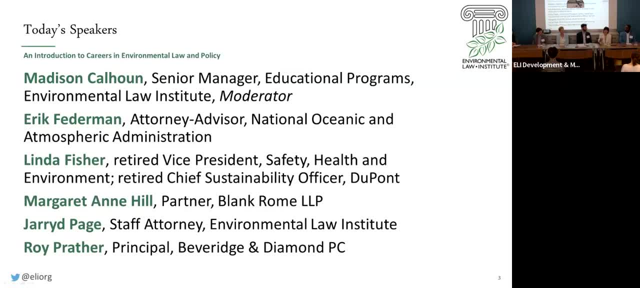 really critical, and even more so as you all go forward in your career, because the internet makes everybody an expert And it is very hard for people to understand. And it is very hard for people to understand who's got good science and who doesn't have. 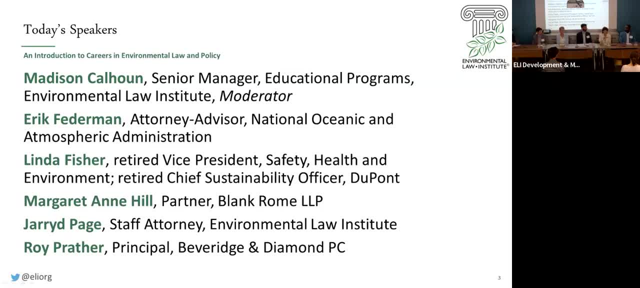 good science And, as a lawyer, really influencing people, not just again about the law, but how to navigate all of that, Wow. So I was going to say something very similar to what Linda said, but she said it better than I would have been able to. 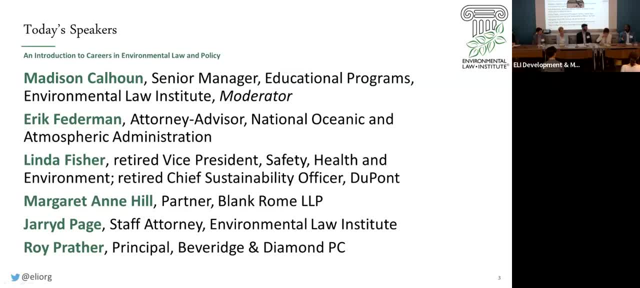 So I'm going to pick it different. So one thing that I wish I had known or understood or fully appreciated was just how broadly the variety that there is that exists. And when you say the term environmental law, everyone has an initial thought that comes. 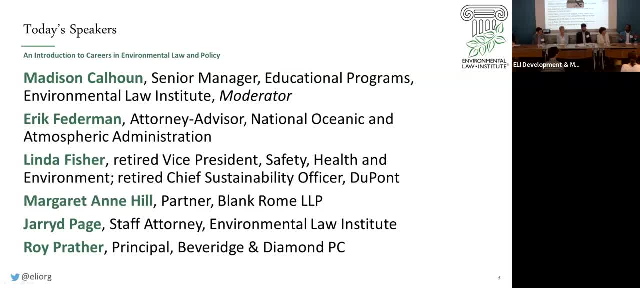 in their mind of what that means, And it doesn't matter who that person is. they're missing probably 90% of what environmental law actually includes, And if I had understood that earlier, I would have approached getting involved in environmental law a little bit different. 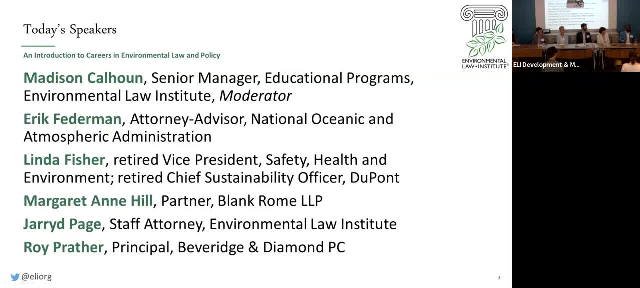 Fortunately it wasn't a total waste of time, because I stumbled around for a bit and then realized: oh, I can do a little bit of a lot of different things. So it worked out well, But if I'd understood it earlier I'd have been able to more. 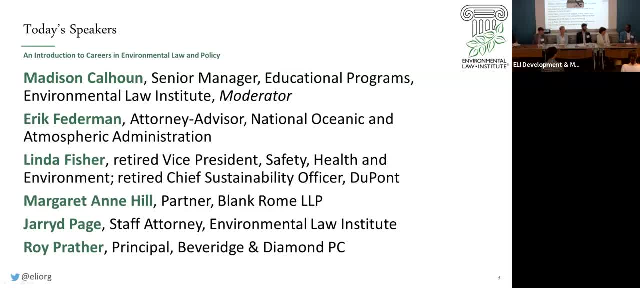 Easily identify the things that were most interesting to me, the things that were most challenging, and really dig in. And even though I said I wasn't going to say anything that Linda did, I wanted to add one other point, because this: I didn't appreciate this fully until after doing the work and 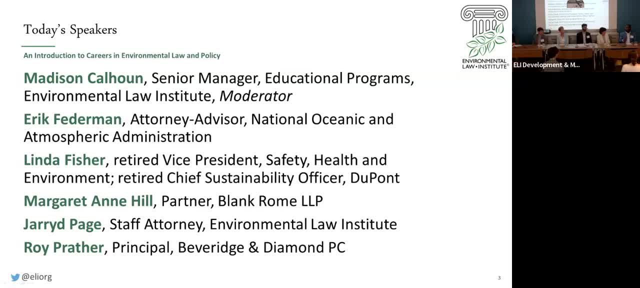 particularly the EJ, work for quite some time. When you do a lot of litigation and it involves, like I said, money back and forth, whatever it's, however you want to interpret that contract, you can find. you're a lawyer, you can find. 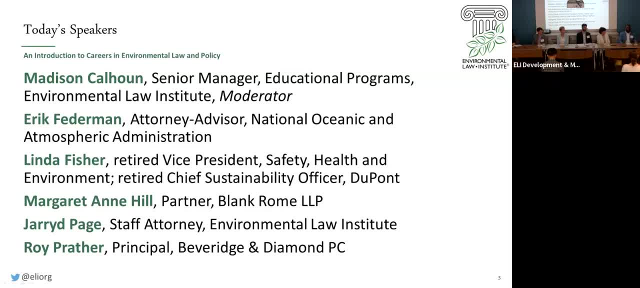 all kinds of things. You can find all kinds of ways to justify why it should be viewed that way. The same thing can be applied to laws. The same thing can be applied to regulations. So that's why the law only gets you something, right. 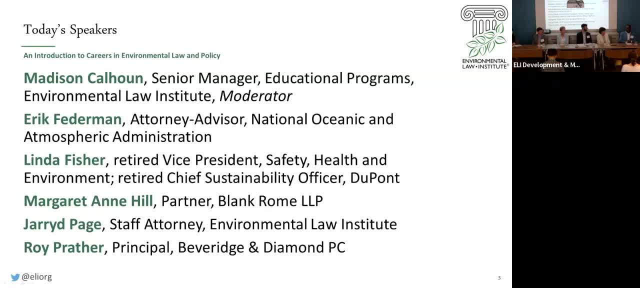 But once you start factoring in, like other policy, once you start factoring in impacts to business, impacts to individuals, then it makes you better able to come up with solutions that will be meaningful for you but also still respect the perspective of others who. 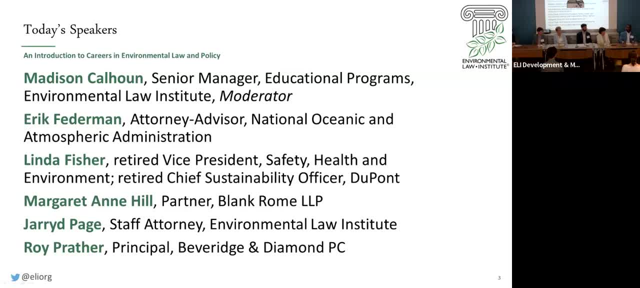 might be opposed to it, And one of the most difficult challenges that I've faced with litigating in general or just in dealing with negotiating an issue, is encountering individual people who don't appreciate or understand that everything is much more complex. I will caution everyone from kind of zeroing in on one particular outcome or viewpoint. 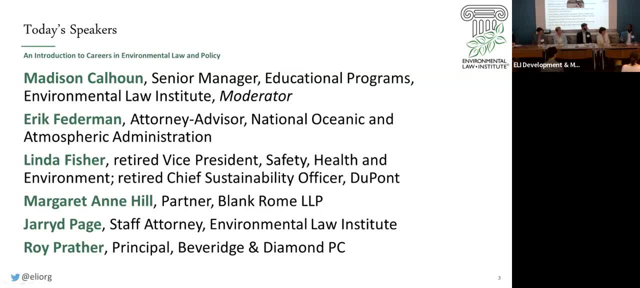 of how things are supposed to work, because what you will do, even if you get what you want, you're probably going to harm someone else And not even have known that you did it. And in the environmental justice context, that is a major challenge that I deal with, where 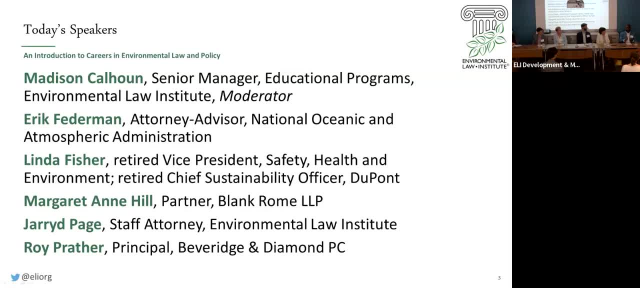 you'll have groups that are very focused on the climate, that are very focused on protecting, conserving lands right, And they'll engage with industry to say: you need to shut down this facility that's providing power to 100,000 people and you haven't offered any alternative for how they're going to get. 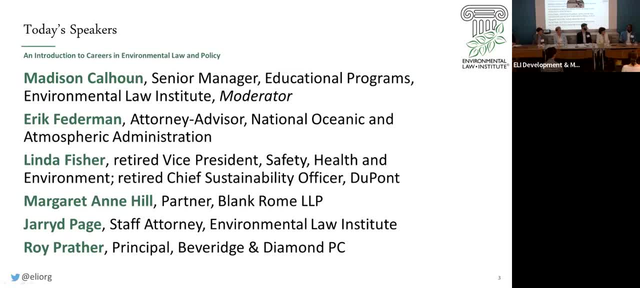 electricity or how they're going to get the other resources that they need. You just know that you don't like this facility because it's emissions. The emissions don't align with what you think it should be. Now maybe those emissions should be reduced and we should talk about ways to do that. 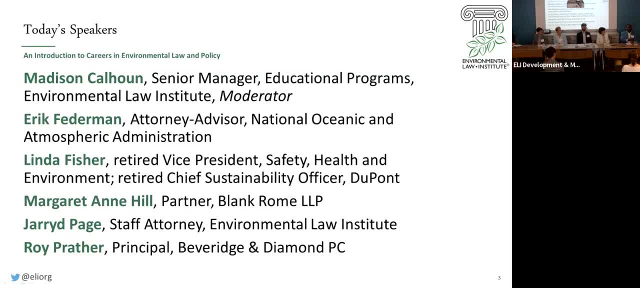 But if the only thing that you think the solution is is shut that facility down, you're not thinking about the actual impacts of what you're doing, And if that's how you approach it, then you're going to end up with suboptimal solutions. 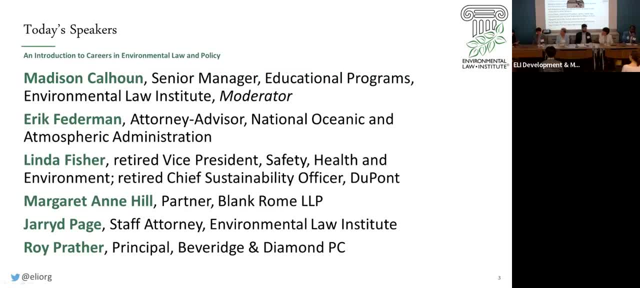 I'll ask one more question and then turn it over to the audience. So the last one is: a lot of people ask us about mentorship, So what roles did mentorship play in your Legal journey so far, and how can law students and new lawyers find mentors along the way? 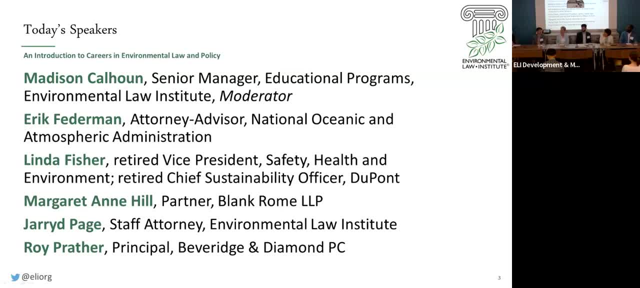 So mentorship got me to where I am today, As I described during my initial sort of how did I get to environmental law? You know I would not have gone to law school had it not been for a mentor at the University of Maryland who first sort of put it in my ear as something that might be of interest to me. 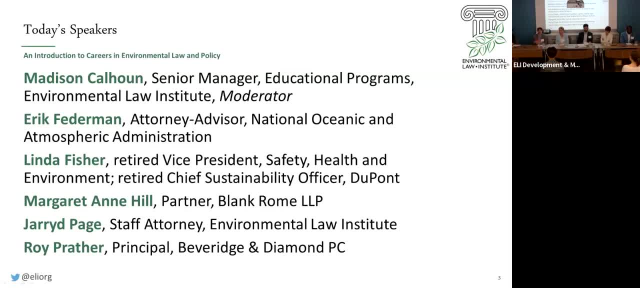 And that mentorship relationship developed Over time, with me sort of just going and asking a lot of questions and being interested, and we built up a dialogue over time and I managed to go to law school and then after law school and during law school- you know my relationship with my professor Rob. 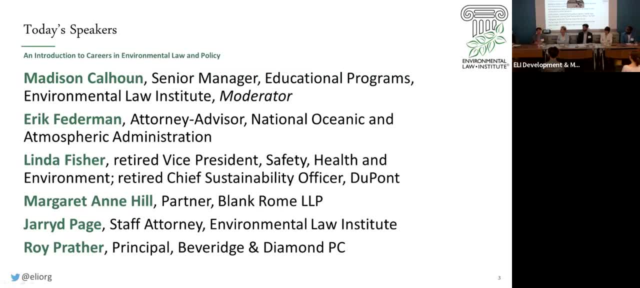 Glicksman, who sort of really helped me understand what it what it means to be an environmental lawyer, what are the opportunities that I might be able to take advantage of as an environmental lawyer, and then was instrumental in sort of And sort of helping me find my my place at at Eli and again, similarly, it was just sort of a me driving, driving those interactions, going, talking, establishing relationships and and sort of what can you do? 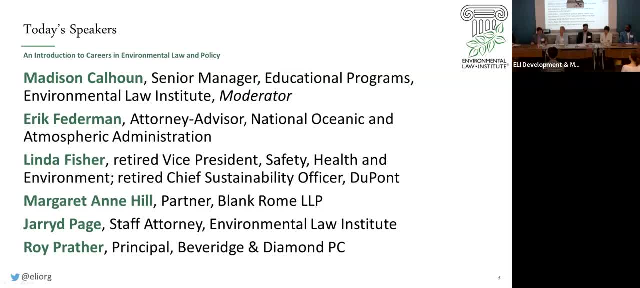 you're already doing it by coming to something like this today and learning about what types of careers are environmental law and asking us questions. But it also goes to my my answer to the previous question, Which is: just don't be afraid to reach out to people. don't be afraid to reach out to someone who is doing work that you think is interesting and just sending them an email or giving them a phone call and just saying hey. 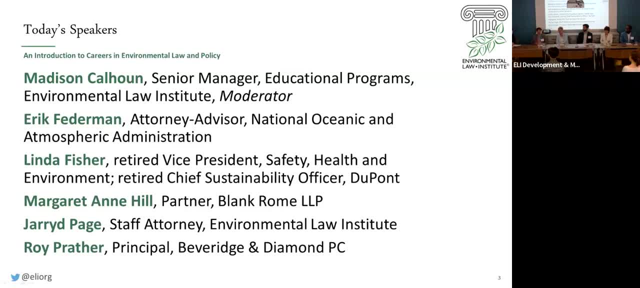 What you're doing is really cool and i'd love to talk to you about it. people like to talk about what they do, so if someone here is you're interested, chances are they'll be happy to talk to you and help you. so don't be afraid and just go for it. 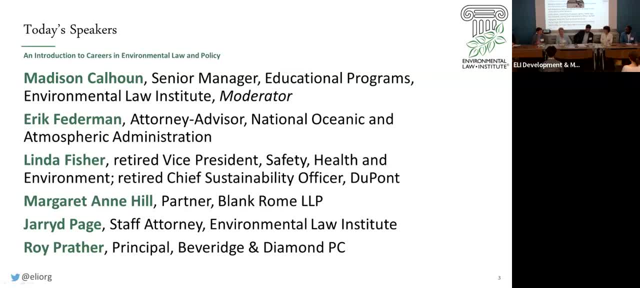 Thank you. I had a mentor when I was a Department of Justice. I really didn't have any other mentor but this person- I know that you know or and shields, close friend, yeah, And was someone that she was a assistant section chief when I went there and the group that I was in and she really 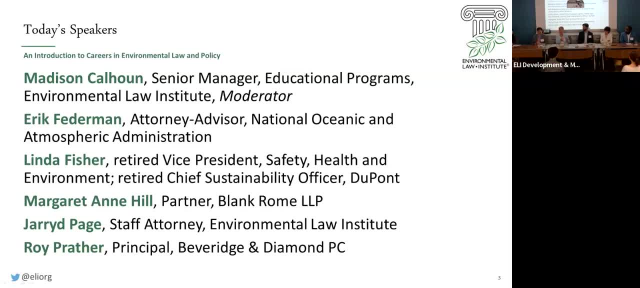 made sure that when I came into doj- because I had not been practicing that time, coming from Gulf oil- you know- I have my law degree- that I was exposed to a wide variety of practice areas in terms of environmental law, ability to assist with trial. 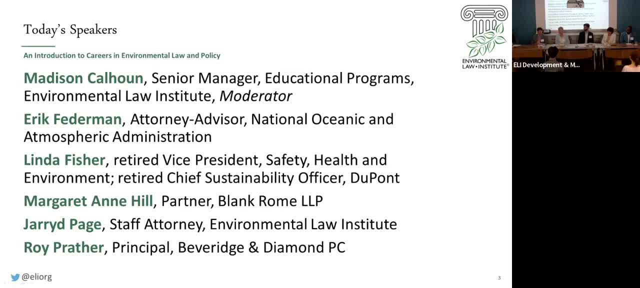 work, appellate work, work on the Hill, you know- policy work. So she really made sure that she took the time and effort to expose me to everything as much as she could, because she was a very busy person in terms of running the section that she was running. But I would say 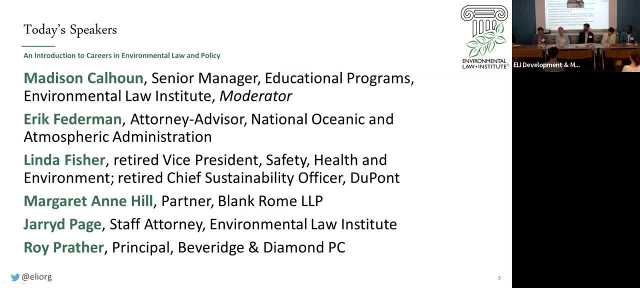 that she really helped me significantly in terms of expanding my interest in practicing environmental law. And then, when actually you all trying to reach out to mentor, the one thing I think that you're finding here is that probably everybody sitting here on this panel loves the practice of 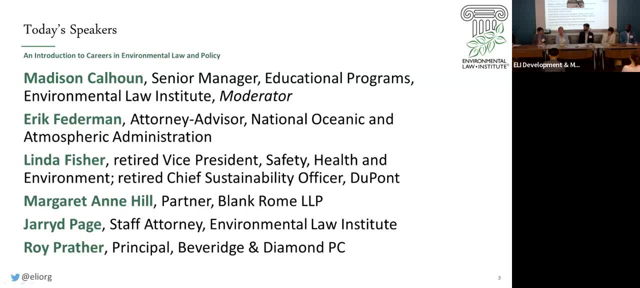 law, and especially environmental law, And that's the person- whoever- I mean, it could be any one of us- that you can reach out to after this program. But if you find somebody that's interested in the practice of law, whether it's environmental law or environmental law or environmental law, or 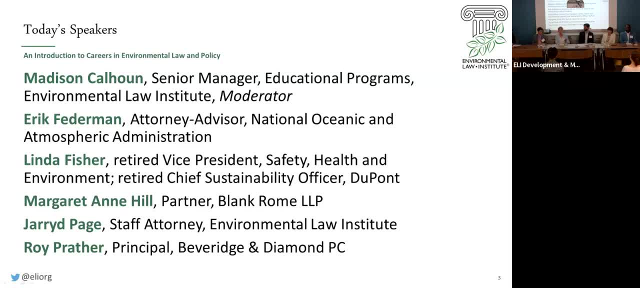 or not, and you're interested in practicing law, that's the person who I think can be really your best mentor, somebody that loves the practice of law. And some people go into law school and decide like hey, this is for me, and drop out. you know, first or second year Other people graduate and 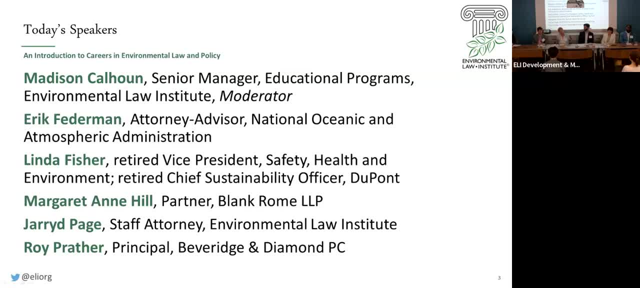 then decide it's not for them, But somebody like me who's been for a long time. you know that I must love the practice of law. I'm sitting here doing it forever, So I would just say that, yeah, find somebody that loves the practice of law, no matter how long they've been practicing, And that 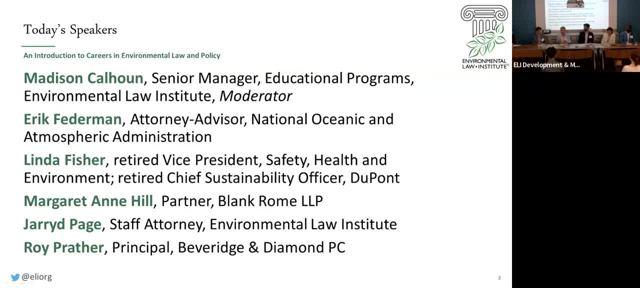 person is going to be a great mentor. They don't have to be in your firm, in your company, in your neighborhood, you know, in whatever organization you are, you can just reach out to people. I think you're exactly right that people that love the practice of law, whatever area of law it is. 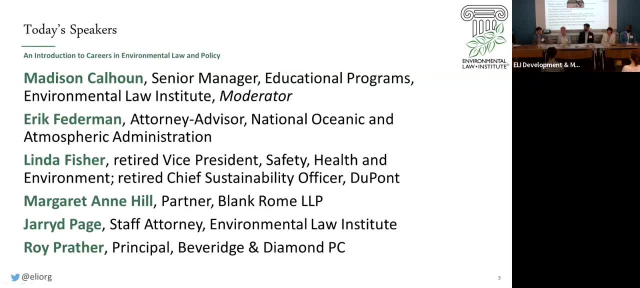 love to talk to upcoming students and associates and somebody interested in practicing law about what it's all about, Because the one thing- again I'll just go back to this- that I've found it immensely rewarding is that you're helping somebody with a problem, And it can be. 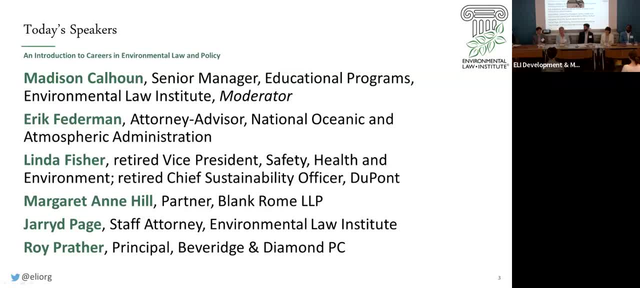 unbelievably, unbelievably rewarding. even if you don't get the result you want, want it or they want it, you did your best And that can really make you feel good inside that. okay, I tried or I achieved my objective. So I would say: find that mentor, but it doesn't. 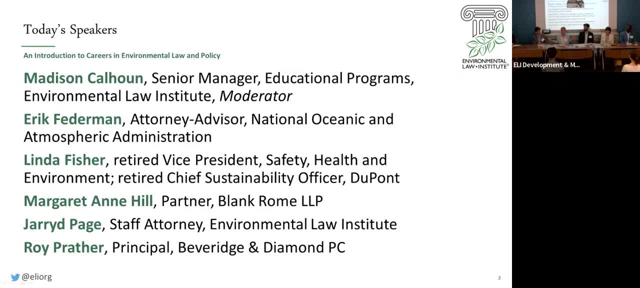 have to be in your organization. It can be somebody outside, it can be any one of us. Yeah, I'll second everything That Peg and Jared said. I found people to be very welcoming and generous with their time, So I'd encourage you to reach out to folks whose work you find interesting, especially ones who 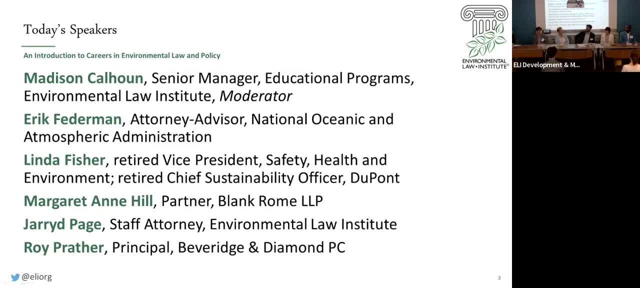 seem passionate about it. I'll say my own experience, at least in law school and since then, people who I consider to have kind of a mentor-mentee relationship with are all people that I've worked with. I found it really hard to like approach professors and go to all the 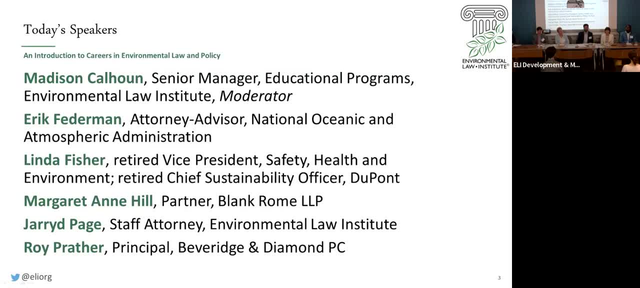 office hours and talk to them and get advice that way. I mentioned that I had some clinical experience in law school And I think in the process you know of working in the clinics I was able to really build relationships with the clinical staff and the clinical directors. 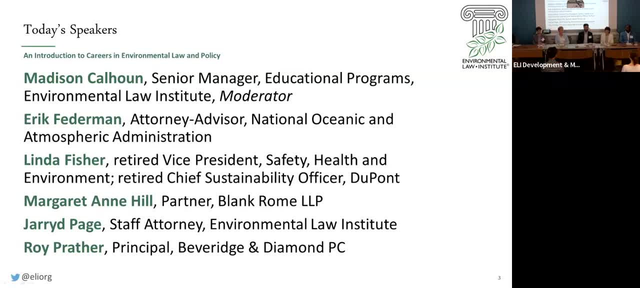 And those were really valuable, helpful relationships for me as I was thinking about kind of what the field was and what a career in environmental law could be. And I'd say the same thing about the folks who I worked with during my internships. 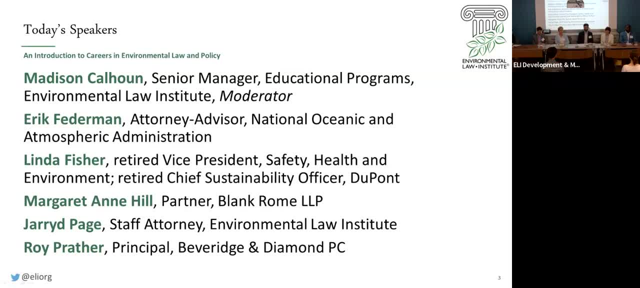 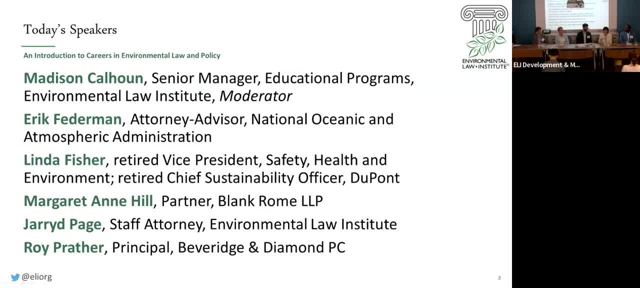 particularly if you enter into a new organization, you need to find, you know, mentors, people that can kind of help you navigate, learn the new who's, who, who to stay away from, who to really understand and and can help you figure out how to handle difficult circumstances. 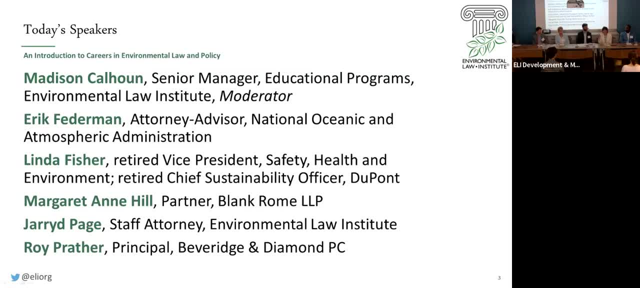 difficult personalities and that sort of stuff, And they may or may not also be sponsors. Sponsors to me are somebody who knows you, knows your strengths, is willing to open a door and shove you through it. And when I look at how I kind of came up, 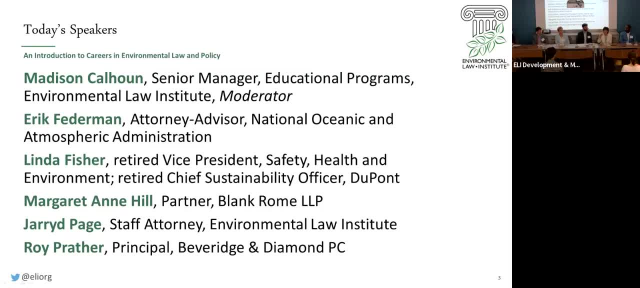 both in my career at EPA and even in corporate America, it was really having somebody who could open doors I didn't know needed to be opened or should be opened and had the confidence in me to push me through the door and say I can do it, And so that kind of sponsor role, I think. 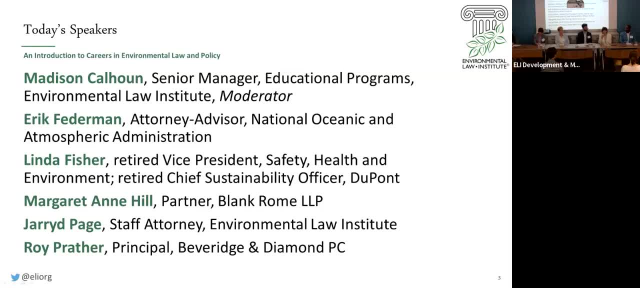 is as important as a mentor, And sometimes they can be the same person, but sometimes they're very different people And I'd encourage you to look at both. So I agree with that a thousand percent. My career would not even exist if not for a couple of key sponsors, but also a number. 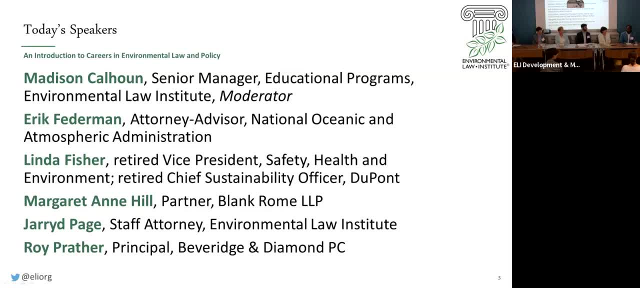 of mentors who helped me navigate. I was terrible, really, for the first few years of my career in actively seeking or taking advantage of mentoring opportunities that were available to me, And what I quickly learned after a year or two of stumbling around is that no person is an island. I'm sure all of 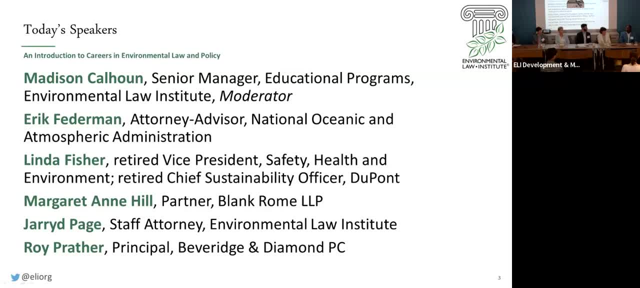 you are incredibly intelligent, hardworking, all of that great stuff. That will not be sufficient to get you where you want to be, wherever you go, because everything's relationship-based right: The opportunities that you learn about, the information that you gain, access to that everyone. 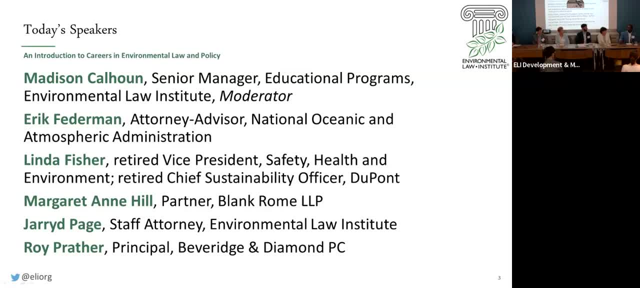 else may not know about. that will help you maneuver in a way or find the opportunity that fits what you want to do. that all comes from relationship, So I echo everything they said in terms of actually reaching out to people And don't be shy about it, Don't email someone, and 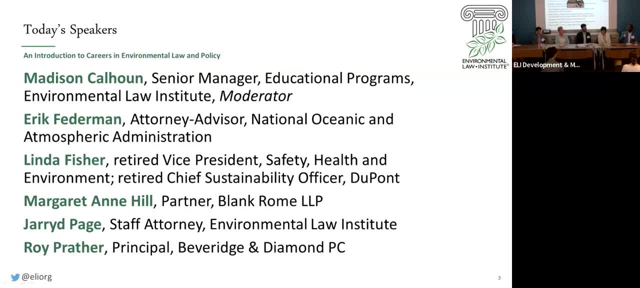 say, hey, please will you be my mentor. I mean, that's a little awkward, But people still will likely respond. But instead showing that curiosity about what they do, that's how you just start that process of them getting to know you better, you getting to know them better, And I think that's. 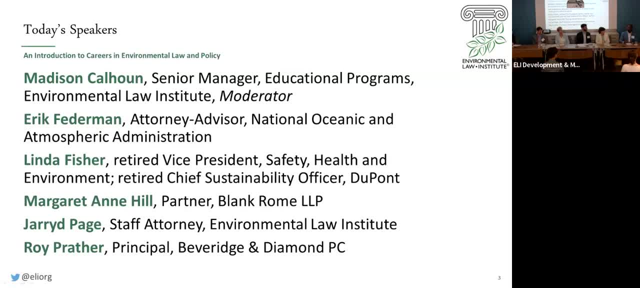 what I would say to them and what they do, And that's a relationship they can develop. And also, the one thing that I would highlight is: don't underestimate the value of the relationships you have with your peers, Because what they do is they know other people, They have other mentors. 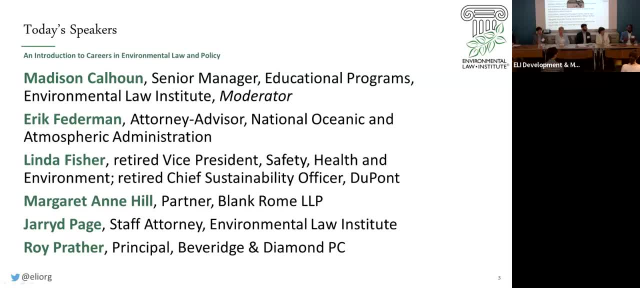 And you can actually be expanding potential mentors for yourself through the relationships you have with people you're already in class with. Maybe that person has a great relationship with a particular professor and can say, oh, you're interested in this, You should really talk to. 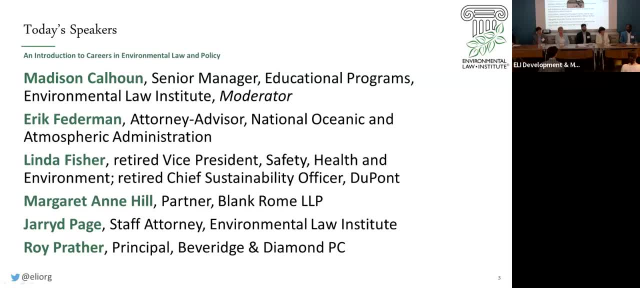 this person And that professor can then expose you to other opportunities, And so one thing that people, particularly early on in careers, have a tendency to do is kind of identify that person that's at the very, very top, that runs the company, that is like the general. 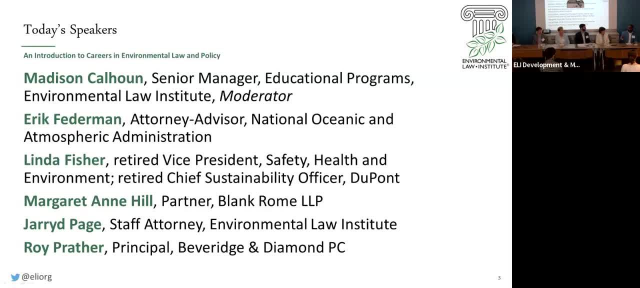 counsel of the organization, things like that, And then say I'm going to go find that person and make that person my mentor, Which totally fine, But there's all kinds of different people along the way who are in very different roles and different capacities They're doing really. 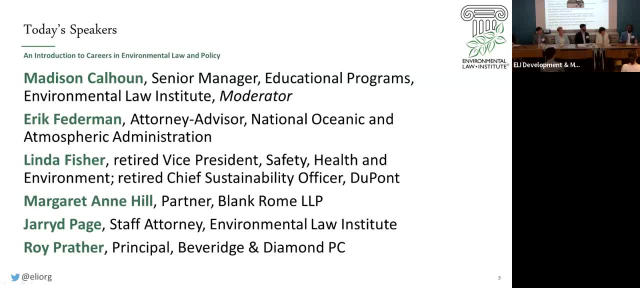 interesting things and are great people that you can meet and that you can learn from, and that you who could turn into A sponsor for you, for example, And so you know everything that everyone said I think is great And I think you know making sure you're intentional about trying to reach out to people. 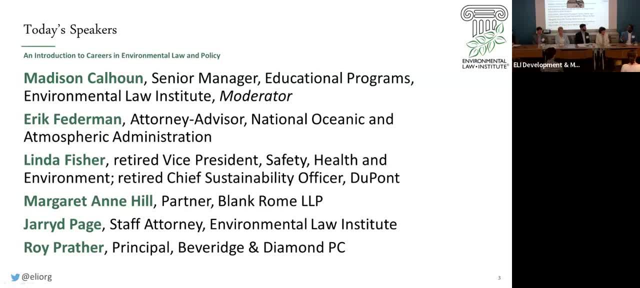 And this panel is a perfect example, And I'm sure you'll, you know, hear from other people over the course of summer school. When people say, reach out if you have questions about X, Y and Z, take them up on that, because they do want to hear from you and be helpful to you in some way, And even 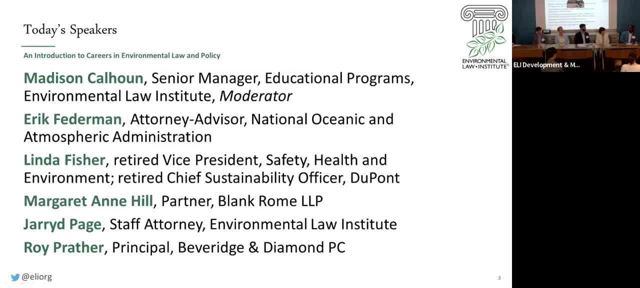 the ones who don't say it. if they're doing something interesting, reach out to them And also don't be afraid to follow up either. I mean, people are incredibly busy, And sometimes the timing of that email coming in might have been while I was right in the middle of doing a whole bunch of things. 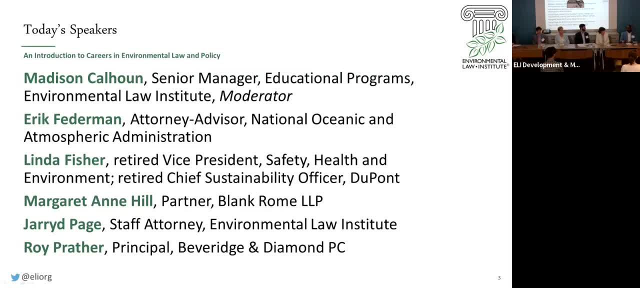 And I meant to respond to the email and just forgot Send a little follow up note, you know, a week or so later- Oh yeah, I meant to respond to that. you know that kind of thing, And then we can find time to chat next. you know, you know we're on our way. So, yeah, reach out, follow up and, you know, think broadly about who can be mentored, who can provide, you know, give you the support. 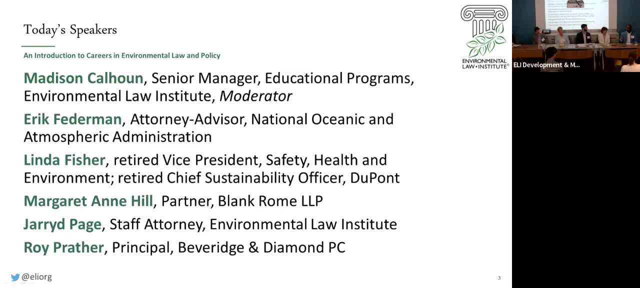 And also the last thing. I keep going on here because this is a big thing for me, because, like I said, I wouldn't be anywhere in my career without mentors and sponsors. But also, when you're thinking about having that relationship, also think about you know, you have something that you bring a value to the table too. 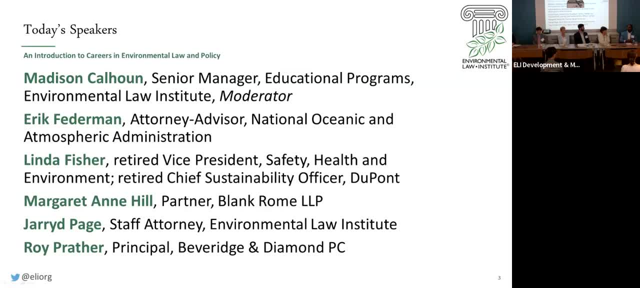 How could you be, you know, helpful to or, you know, expose someone to something interesting that they might not even be thinking about? Like they can mentor you, but they can learn from you too. Sometimes it's just a difference. 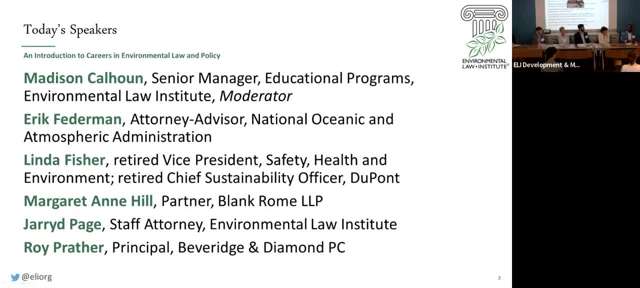 Sometimes it's just a traditional perspective, Sometimes it's: you know you're doing something that that person hasn't actually been familiar with, and now you can expose them to. you know, something that they can explore further, And so it doesn't have to be a one-way street either. You actually do bring something unique and significant to the table as well, which is part of the reason why people will invest and, you know, want to put that time too. 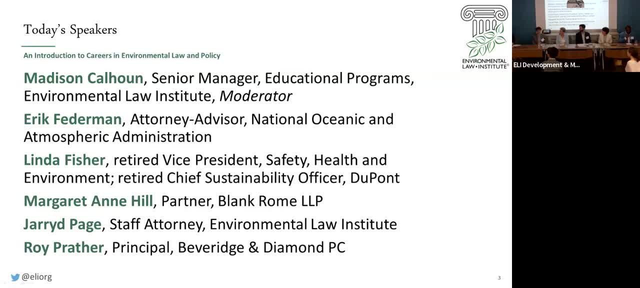 Thank you so much. We're going to turn things over to the audience now. So our educational programming intern, Grace, is going to bring a microphone around so that anyone watching backwards- And you know later- can still hear your questions. 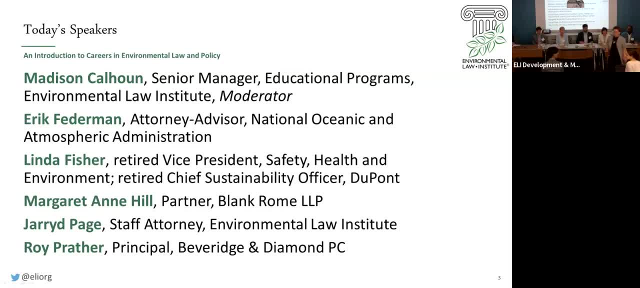 So I think I still look back. Yeah, so I have a question. I'm kind of mid-late. career in environmental and cultural resource compliance and cultural resources was something that hasn't really been included in the conversation so far. Do you see a place for that in historic properties? 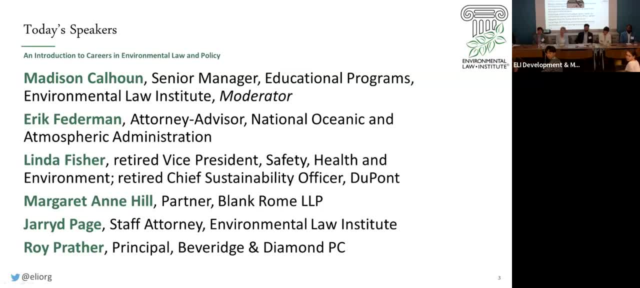 I would say absolutely representing companies that are interested in developing property. We've run across issues all the time having to do with conducting archaeological surveys and trying to understand where there might be historic artifacts. and what do we need to do to, you know, to comply with respect to the National Historic Preservation Act and then also state historic preservation. 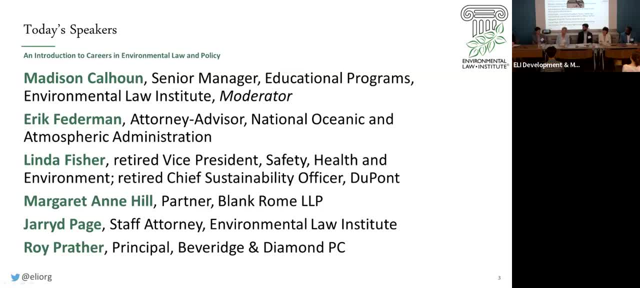 Okay, So we do run across that all the time And in fact I had a matter that I settled last year with a community group that was concerned about a college. happened to be a college in Philadelphia who was expanding its entranceway and there was some concern that there might be some revolutionary artifacts or old Indian artifacts in that area. 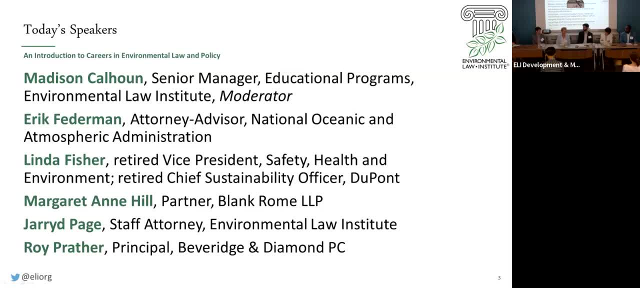 So we followed up, I mean in terms of, you know, getting somebody to do the archaeological survey and understand what impacts there might be. same thing in Philadelphia with a. it was supposed to be a casino that was built on the Delaware River and there was a big, big issue about whether or not that area of the Delaware River was actually. what would you say at the time, during the Revolution War, whether it was river or whether it was land. 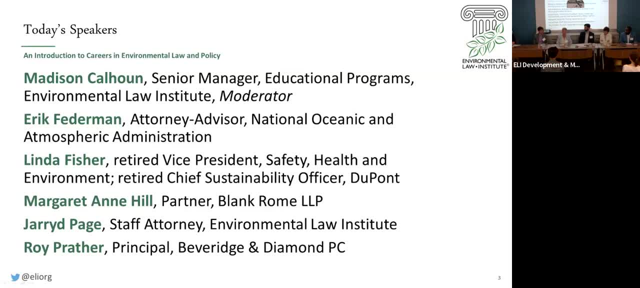 And so that generated a whole lot of activity in terms of archaeological surveys. Indian artifacts or cultural resources might be there, revolutionary artifacts, So it definitely comes up in that aspect. That's how I've seen it in terms of development. Yeah, 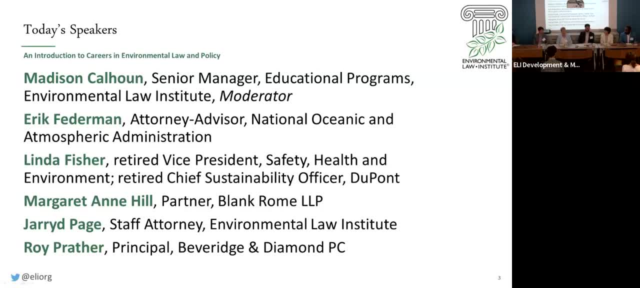 I would say it comes up in my practice a lot too. A couple of the program offices that I work with their missions include cultural heritage and conservation, especially of cultural resources. So with the Office of National Marine Sanctuaries They have a couple sites that are devoted specifically to maritime cultural heritage. 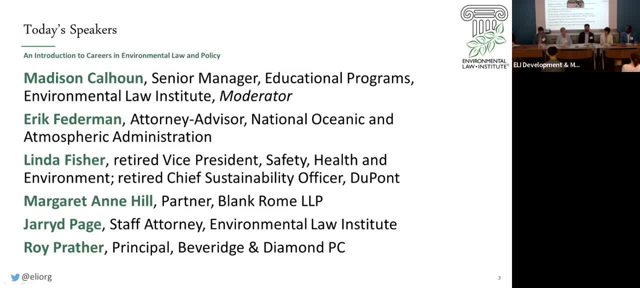 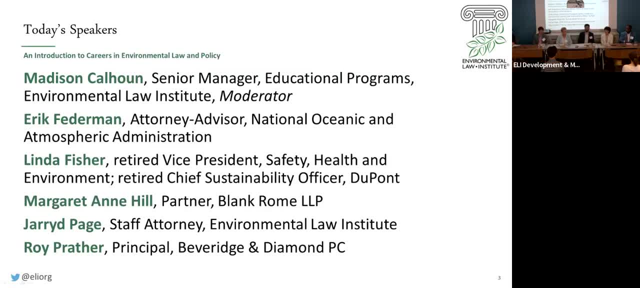 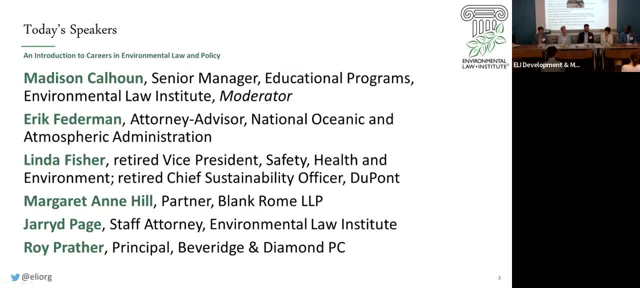 tribe's interest or as partners for a number of things, And those conversations often involve cultural heritage issues. I was just wondering if you, from your experience when you mentioned not having necessarily a science background, a well-being science background and some capacity of translating science and 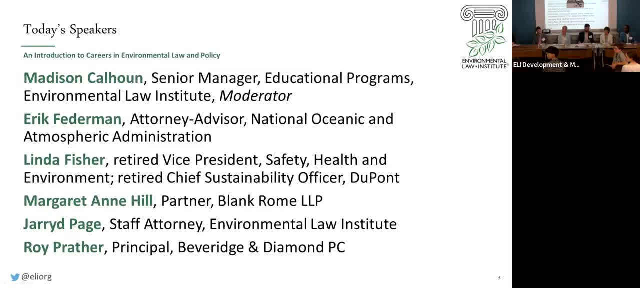 if you had any commentary on maybe seeing scientists transition into more of the policy and law positions, given that you're not a scientist but you're working with them. So Yeah, I don't know the exact numbers, but I have a sizable number of partners in my firm who 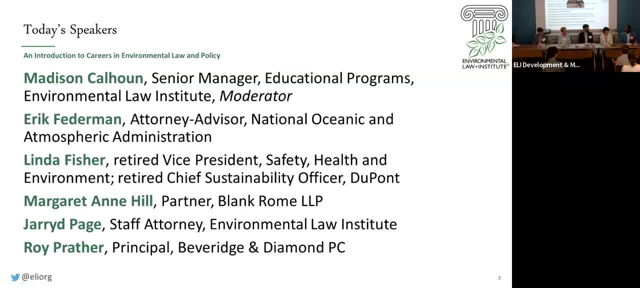 are scientists, So they're the people I actually call and say so I have this issue. I have no idea what this engineer is saying. Can you join this call And they talk and they speak in whatever engineering language they make. Someone was a marine biologist, this other person was a hydrogeologist, all those kinds. 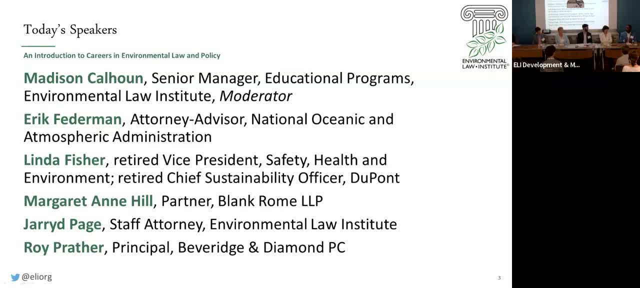 of things. So the transition, I would say, at least in terms of private practice environmental law, I would say in some ways you have a bit of a leg up, as long as you're interested in working in the area that you have the science background in, but also just the exposure to the science. 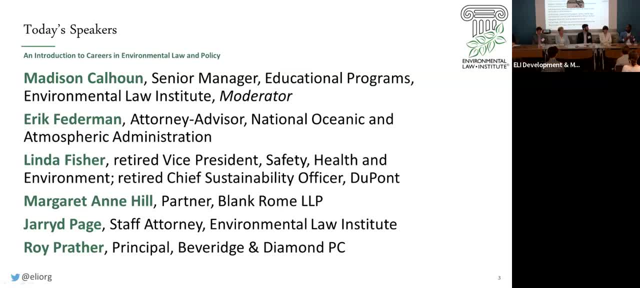 in general, You're going to have to spend a lot less time than I do to get up to speed on what those issues are, And so it's a really great benefit. I think It may be different in other circumstances, but at my firm I mean as soon as we even 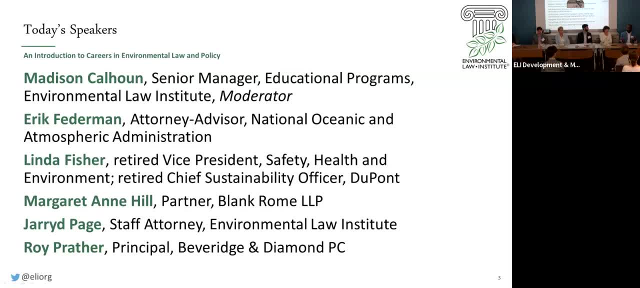 see a resume like, okay, we need to talk to them because there's so much value in having people that you can talk to, You can quickly call that, have that background that can help drill down an issue or talk, like I said to the engineers, who are not lawyers, so they're not going to be thinking. 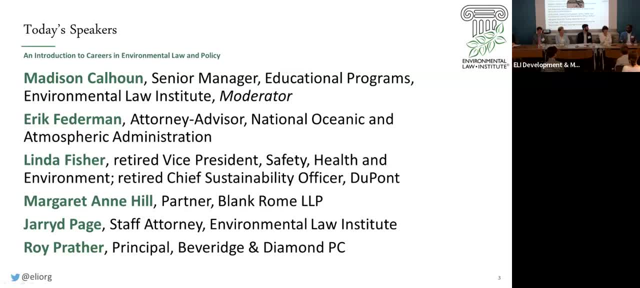 about things in the same way that you are and speak the same language that they speak, to help them understand either? yes, this is what compliance means. No, I understand that you do X, Y and Z this way and the reason you do it, but the law. 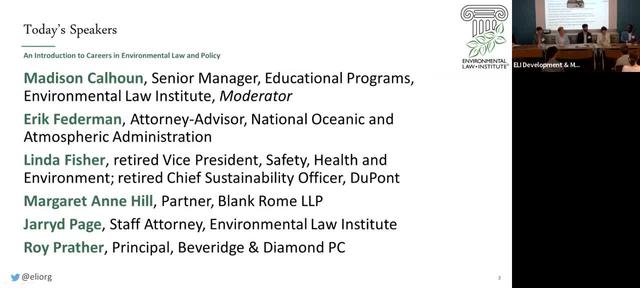 requires us to do this additional thing. Here's what that translates to in terms of what your processes are. So yeah, it does translate, definitely. I would add that At ELI, we've got a couple of PhD scientists on our staff. 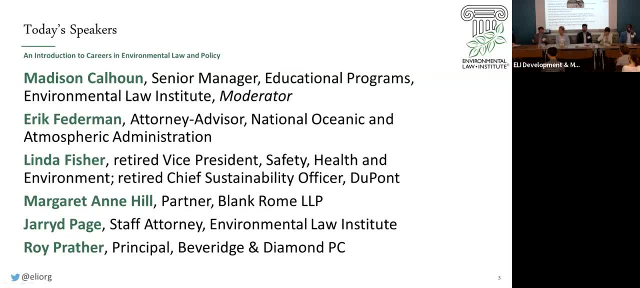 And, as Roy mentioned, we need you, we need the scientists and the science. So we have a PhD climatologist who works on the Climate Judiciary Project, who is essential in helping us understand issues of climate science, how the science is arising in the 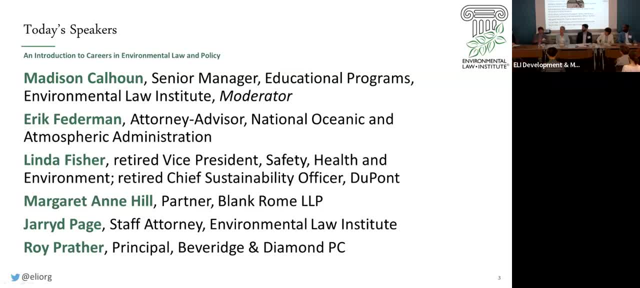 cases And he is a go-to resource for us in answering questions about science topics. And yeah, Thank you. Thank you, That's just to say that you are needed and, with a demonstrated interest in policy, it's a really sort of critical piece. 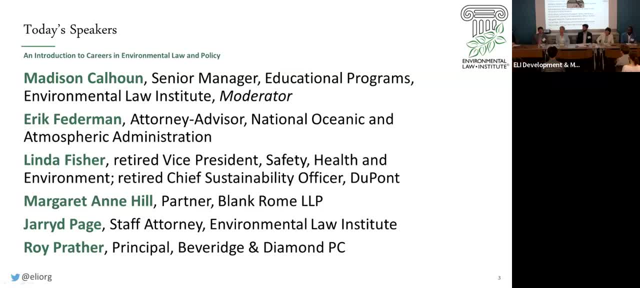 Yeah, We have one or two more questions, Hi, Thank you. I would like to thank all of you for coming and sharing today. I think this would be for everyone that I say that your insights were very helpful. I just wanted to ask a quick question about getting more exposure into the field of environmental. 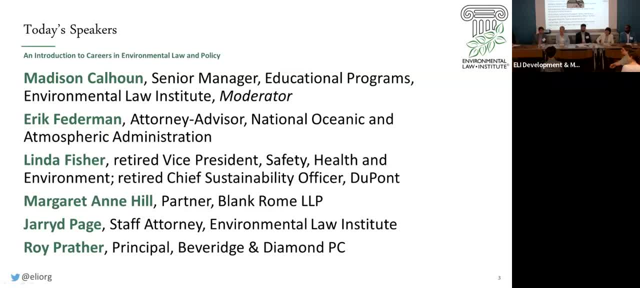 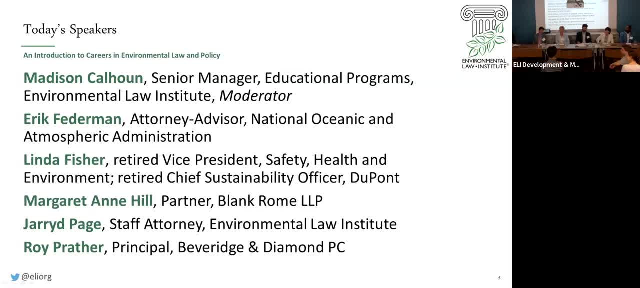 As a pre-law student. law school is a little far away from you and I realize a lot of you kind of figured your way into the field of environmental law during or even after law school. How would you recommend that students like me or people who have yet to attend law school kind of get experience working with environmental lawyers in the field? 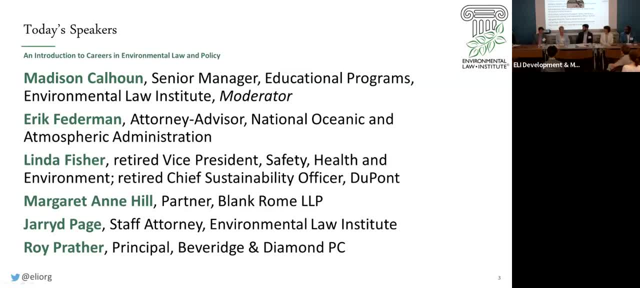 I think one of the things that you could do is: there's a lot of every neighborhood has it. you know there's a local citizens group that might be involved in environmental laws, environmental compliance or non-governmental organizations. you know environmental organizations that usually I'm on the other side of. 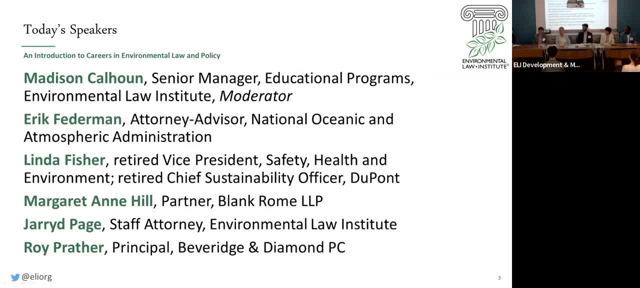 I would definitely recommend that you know, like the Sierra Club or, you know, Center for Biological Diversity, other groups at NRDC that you can reach out to. that would probably help. We'd love to have some interns or somebody coming in trying to assist them with case review. 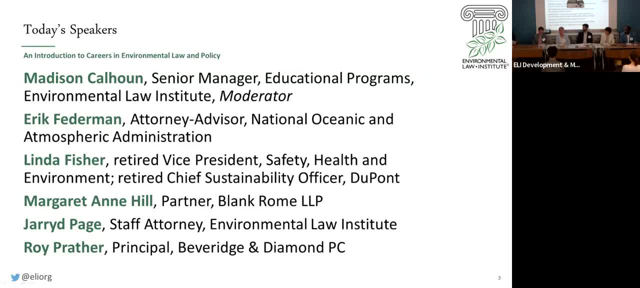 So there's tons of groups out there. Those local groups have never been heard of, and then there's also national organizations. That would be one way of doing it. There may also be law firms, and I'm not thinking big law firms, but maybe smaller law firms, whether it might be an environmental practice or a land use development practice. 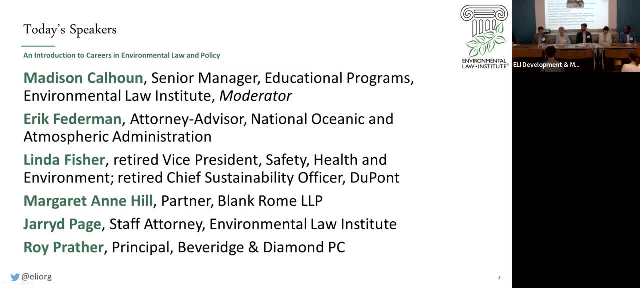 that might be interested in having somebody come in and just assisting you know over the summer months in terms of whether or not it's evaluating again. you know cases, or you know pulling out cases or trying to read documents, review them, evaluate them- in terms of you know where the litigation is going. 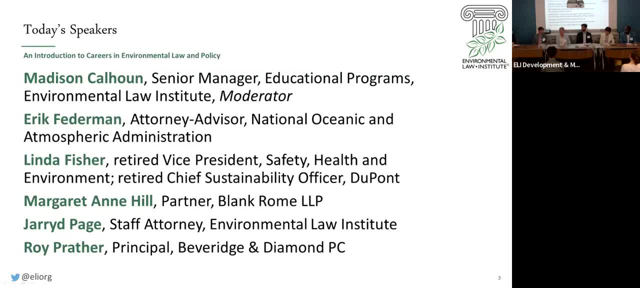 I'm not saying you're practicing lawyer, but they might need that help So. but I would definitely say the environmental organizations would probably be a really good place to start, Adding that ELI has internships During each school semester and during the summer.